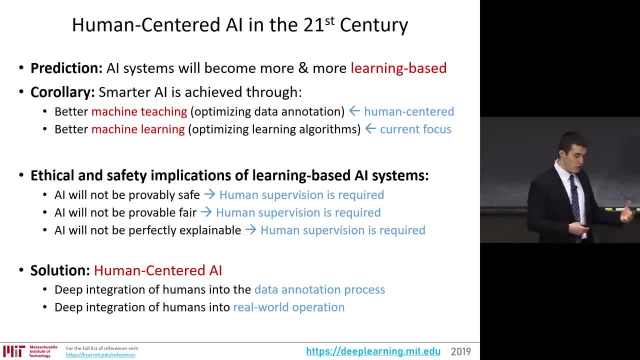 in order to make the systems learn well and operate in the real world. The underlying first challenge, the first prediction under the idea of human-centered AI in this century, is that the learning-based approaches that have been successful over the past two decades- like deep learning, machine learning, approaches that learn from data- 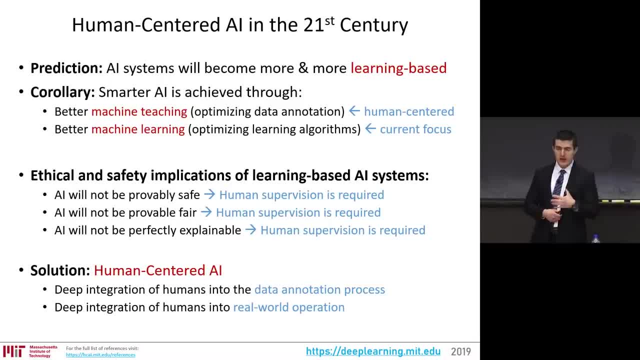 are going to continue to become better and dominate the real-world applications. So, as opposed to fine-tuned, optimization-based models that do not learn from data, more and more we're going to see learning-based approaches, learning-based methods, dominate real-world applications. 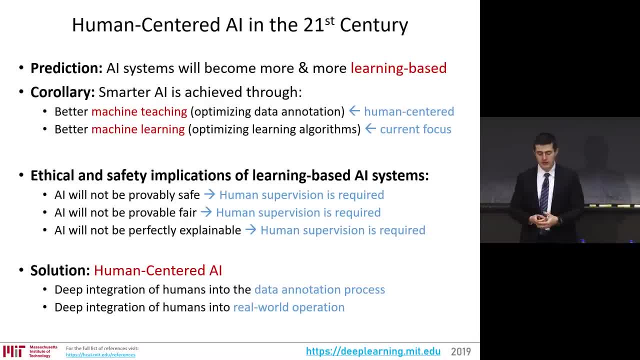 That's the underlying prediction that we're working with Now. if that's the case, the corollary of that, if learning-based methods is the solution to many of these real-world problems, is the way we get smarter AI systems is by improving the machine learning and the machine teaching. 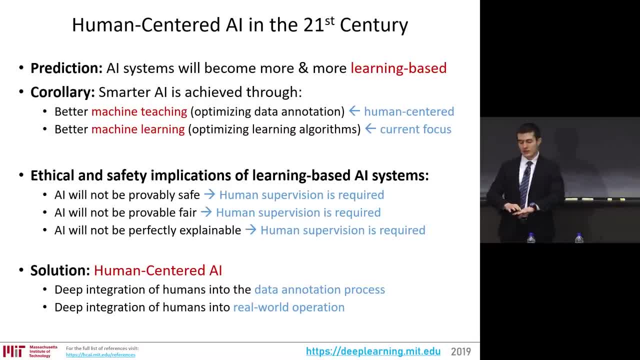 Machine learning is the thing that we've been talking about quite a bit. that's the deep learning, that's the algorithm, the optimization of neural network parameters, where you learn from data. That's the current focus of the community, current focus in the research. 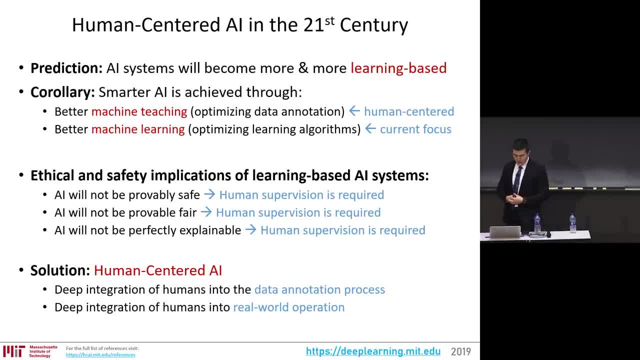 and the thing that's behind the success of much of the developments in deep learning. And then there's the machine teaching. That's the human-centered part. It's optimizing not the models, not the algorithms, but optimizing how you select the data based on which the algorithms learn. 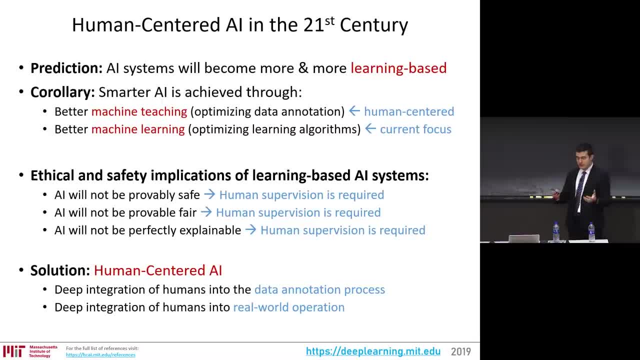 It's to make better teachers, Just like when you yourself are learning as a student or as a child how to operate in this world. the world and the parents and the teachers around you are informing you with very sparse information, but providing the kind of information that is most useful for your learning process. 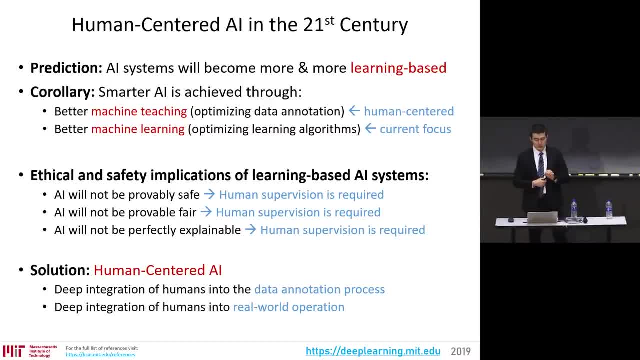 The selection of data based on which to learn, I believe, is the critical direction of research, where we have to solve in order to create truly intelligent systems, the ones that are able to work in the real world, and I'll explain why in ways that I'm referring to. 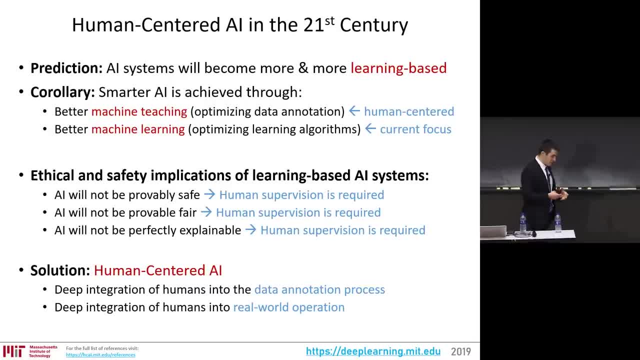 The implications of learning based systems. So, when you have a learning system, a system that learns from data, neural networks, machine learning learns from data- the fundamental, the fundamental reality of that is the model is trying to generalize across the entirety of the reality, which we'll have to be tasked with operating. 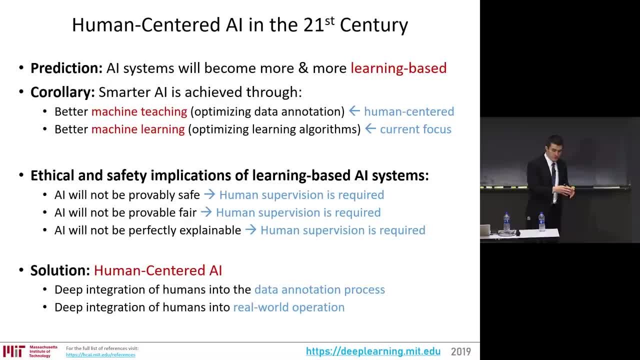 based on a very small subset of samples from that reality, And that generalization means that there's always going to be a degree of uncertainty, There's always going to be a degree of incomplete information, And so, no matter how much we want to, 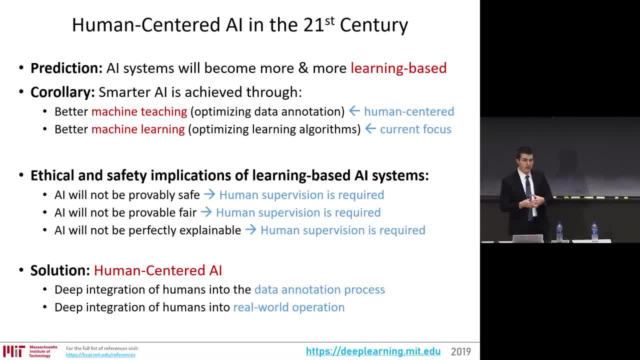 these systems will not be provably safe, So we can't put anything concrete down to how guaranteed to be safe in some specific way, unless it's extremely constrained. Therefore, we need human supervision of these systems. The systems will not be provably fair from an ethics perspective. 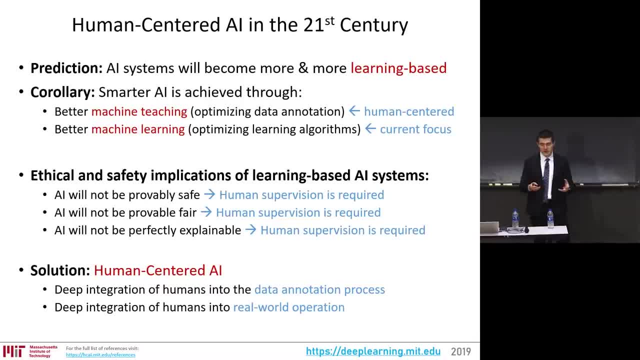 from a discrimination perspective, from all degrees of fairness. Therefore, we need human supervision of these systems And it will not be explainable At any step of the pipeline in which they made the decisions. AI systems will not be perfectly explainable to the satisfaction of us as human supervisors. 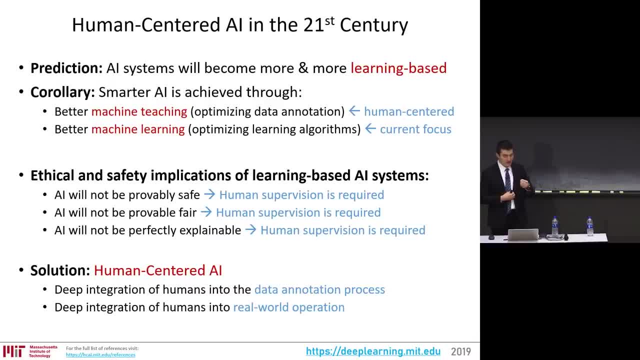 So, there again, human supervision constantly will be required, And the solution to this is a whole set of techniques, whole set of ideas. They're kind of we're putting under the flag of human-centered artificial intelligence, human-centered AI, And the core ideas there is that we need to integrate. 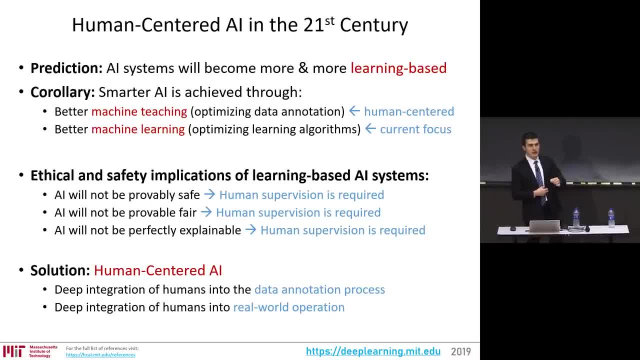 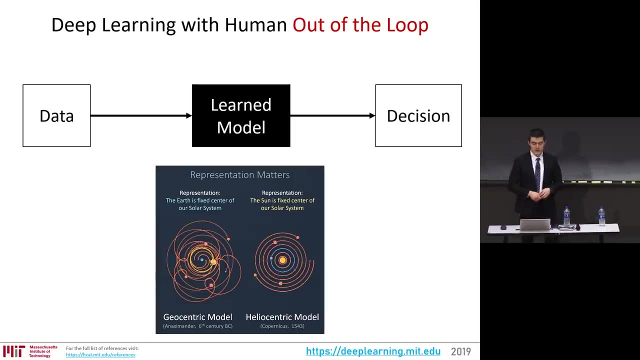 the human being deeply into the annotation process and deeply into the human supervision of the real-world operation of the system. So, both in the training phase and the testing phase, the execution, the operation of the system. So this is what deep learning looks like. 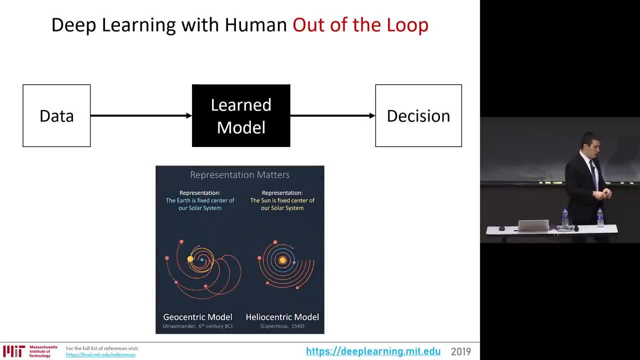 with the human out of the loop. The human contributes to a learning model by helping annotate some data And that data is then used to train, to train a model that hopefully generalizes in the real world And that model makes decisions. And deep learning is really exciting. 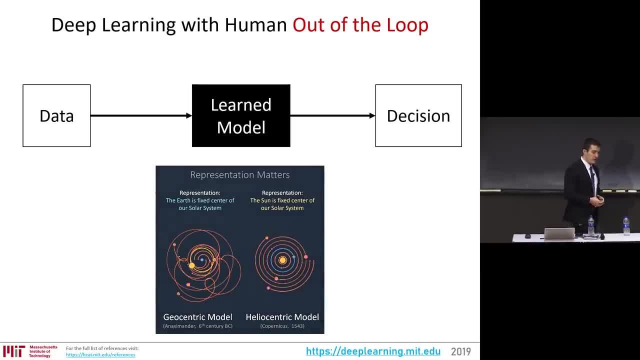 because it's able to, in a greater and greater degree of autonomy, able to form high-level representations of the raw data in a way that it's actually able to do quite well on certain kinds of tasks That were before very difficult. But fundamentally, the human is out of the loop. 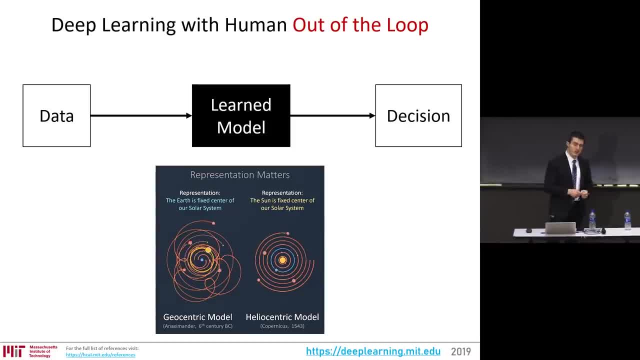 both of the training and the operation. First you build the dataset, annotate the dataset and then the systems run away with it. They train on the data and the real-world operation does not involve the human except as the recipient of the service the system provides. 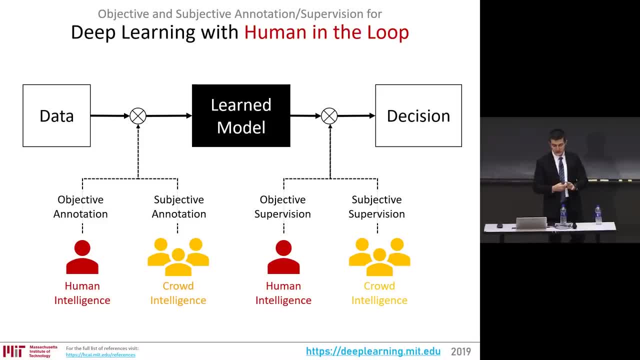 Now the human in the loop version of that. the human-centered version of that means that annotation and operation of the system is both aided by human beings in a deep way. What does that mean? So we can look at human experts, so individuals. 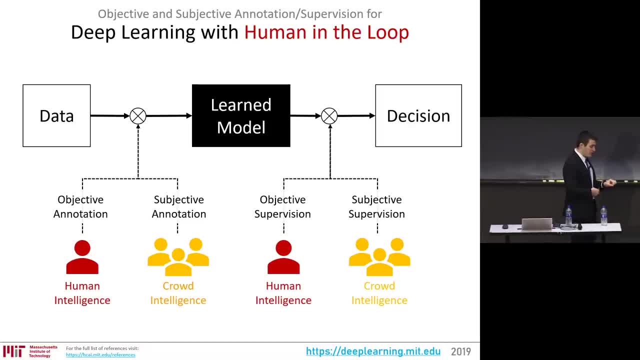 and crowd intelligence, The wisdom of the crowd and the wisdom of the individual At the training phase. the first part of that is the objective annotation. We need to significantly improve objective annotation, Meaning annotation where the human intelligence is sufficient to be able to look at a sample. 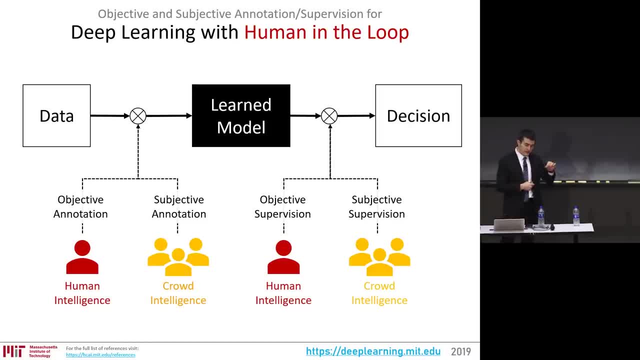 and annotate it. This is what we think about as an image net and all the basic computer vision tasks where a single human is enough to do a pretty damn good job of determining what's in a particular sample. And then there's subjective annotation, Things that are difficult for humans. 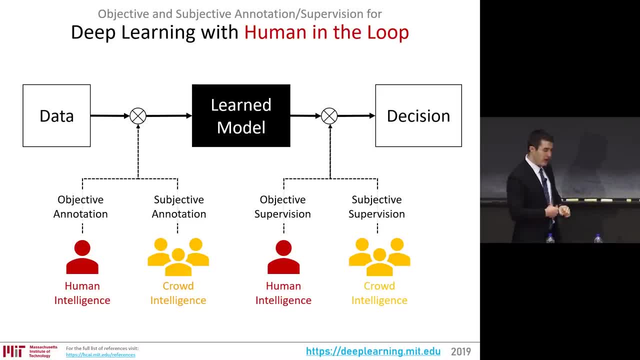 to determine as a singular sample of a human being. As a crowd, we kind of converge in these difficult questions. These are questions at a low level of emotion, These things that are a little bit fuzzy, that require multiple people to annotate, And at the high level. 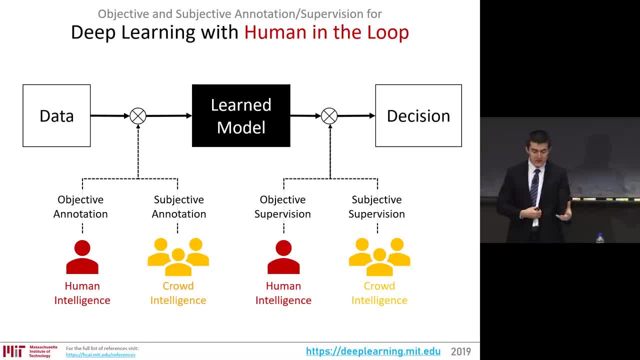 are ethical questions of decisions that an AI system is tasked to making or we're tasked to making, that nobody really knows the right answer to, And as a crowd we kind of converge in the right answer. That's where the crowd intelligence comes in. on the data annotation step, 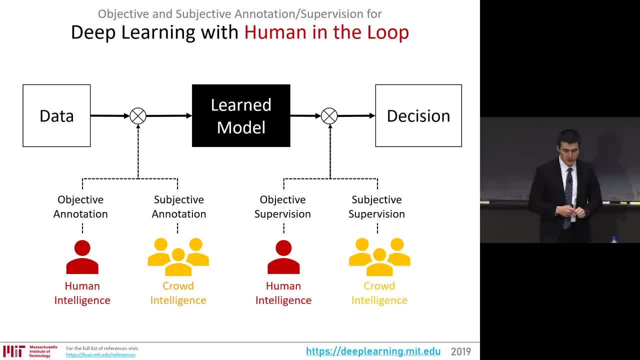 Now in the operation, once you train the model, the supervision again of the system based- and I'll give examples of this more concretely- the wisdom of the individual is, for example, operating an autonomous vehicle, the supervision of that autonomous vehicle. 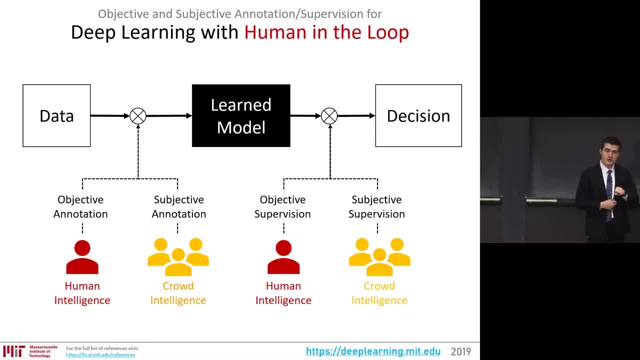 a single driver is tasked with supervising the decisions of that AI system. That's a critical step for a learning-based system. that's not guaranteed to be safe, that's not guaranteed to be explainable and the subjective side of that, where the crowd intelligence is required. 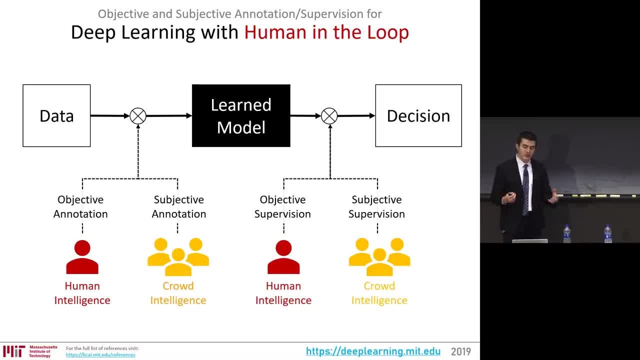 where a single person is not able to make it. these are again ethical questions about the operation of autonomous systems, The supervision of autonomous vehicles, the supervision of systems in the medical diagnosis, in medicine in general, and this is AI operating in the real world. 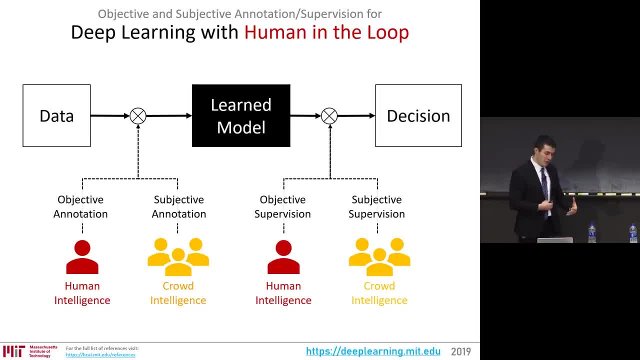 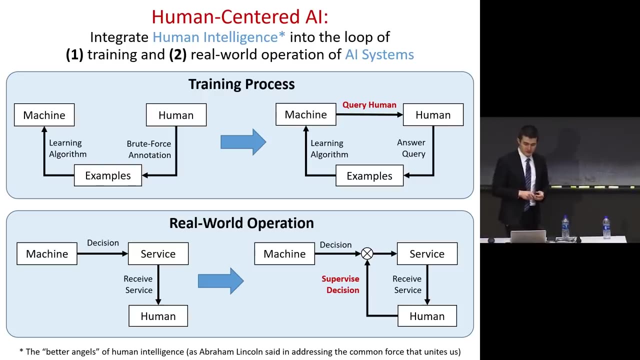 making ethical decisions, and making ethical decisions in the real world, Making ethical decisions that are fundamentally difficult decisions for humans to make, and that's where the crowd intelligence needs to come in, And so we have to transform the machine learning problem by integrating the human being. 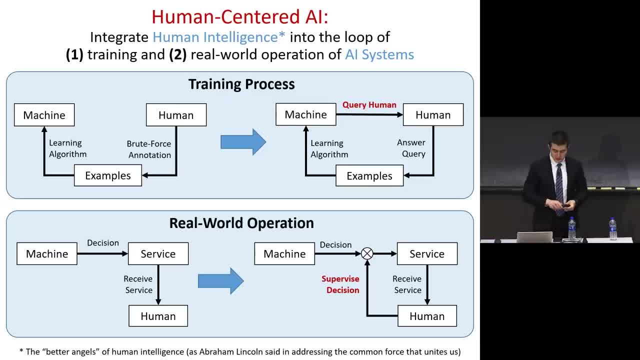 First up top in the training process on the left, that's the usual machine learning formulation of a human being doing brute force annotation of some kind of data set: cats and dogs in ImageNet segmentation, data set and cityscapes. 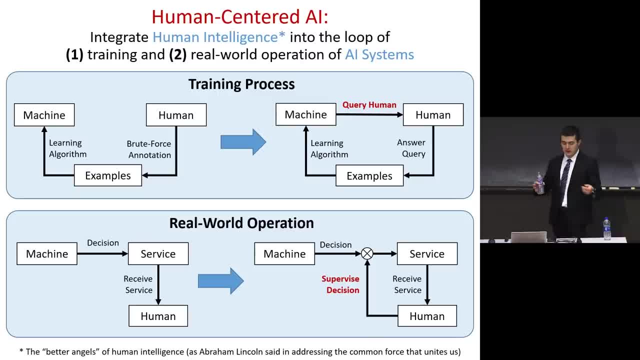 video action recognition in the YouTube data set. Given the data set, humans put in a lot of expensive labor to annotate what's going on in that data and then the machine learns. The flip side of that, the machine teaching side, the human centered side of that. 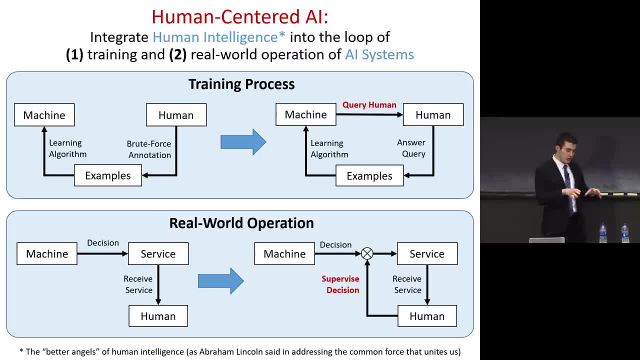 is the machine. instead, The learning model, the learning algorithm- talking about most of the neural networks here- is tasked with providing the machine selecting the subset, the small, sparse subsets of the data that are most useful for the human to annotate. So, instead of the human doing the brute force task first, 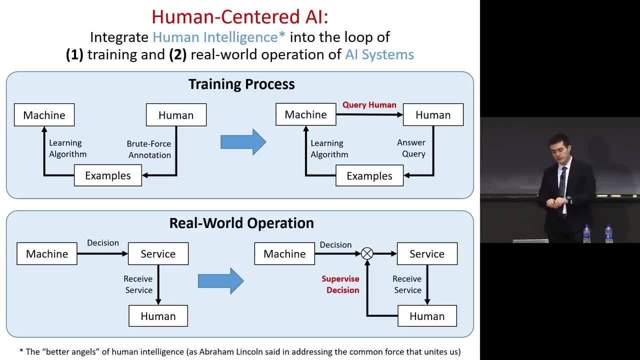 of the annotation. the machine queries the human. This is the field called machine teaching. The machine queries the human with questions And therefore the task is- and this is wide open research field- the task is to minimize in several orders of magnitude. 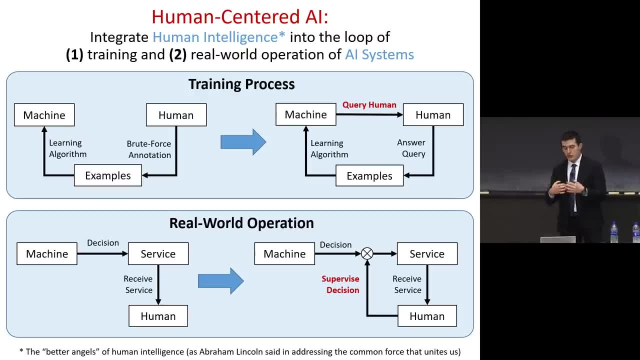 the amount of data that needs to be annotated. In the real world operations side, the integration of the human looks like this: On the left, the machine now trained with the learning model makes decisions and the human living in this world receives the service provided by the machine. 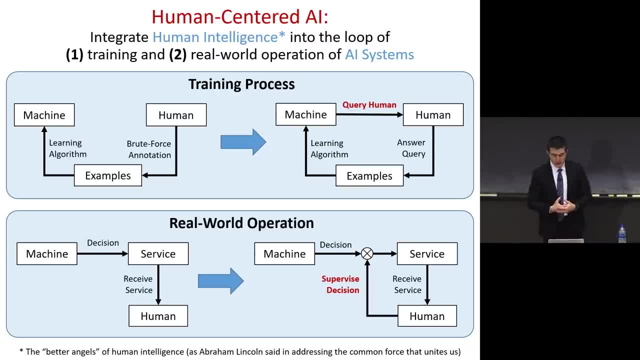 whether that's medical diagnosis, whether that's an autonomous vehicle, whether that's a system that determines whether you get a loan or not, so on. With the human-centered version of that, the machine makes a decision, but it's able to provide a degree of uncertainty. 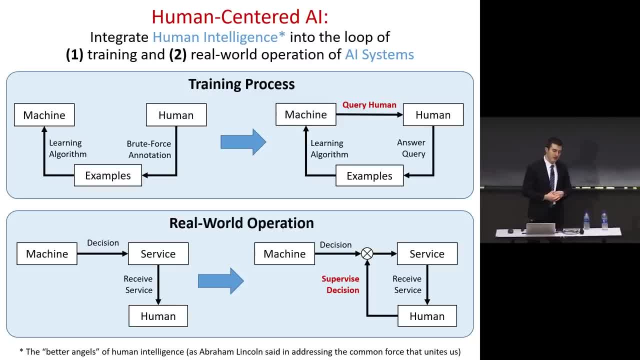 This is one of the big requirements: to be able to specify a degree of uncertainty of that decision such that when uncertainty is below a certain threshold, human supervision is sought And again in that decision, whether that's a costly decision financially or a costly decision in terms of human life. 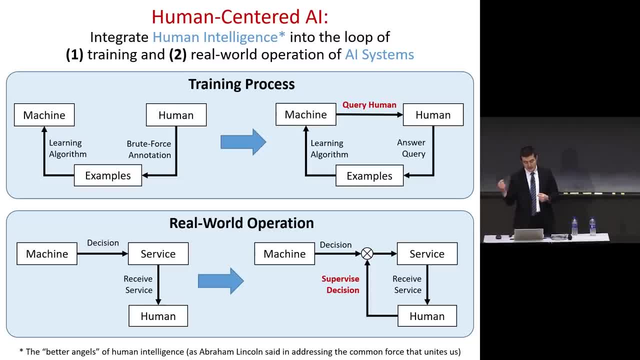 human supervision is sought And the service is received by the human, by the very same humans that are providing the supervision, or another set of humans, But ultimately the decision is over-sought by human beings. This is what I believe is going to be. 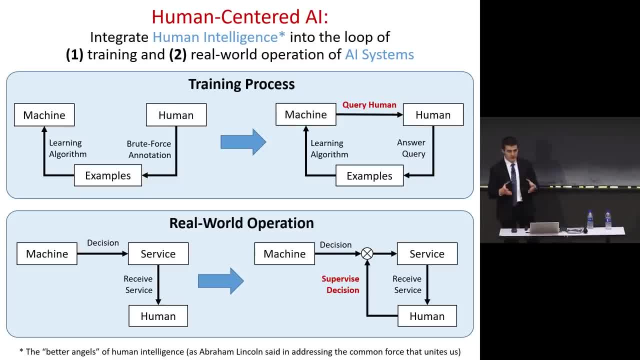 the defining mode of operation for AI systems in the 21st century is: we won't be able to, as much as we'd like to escape, to create perfect AI systems that escape the need to work together with human beings at every step. 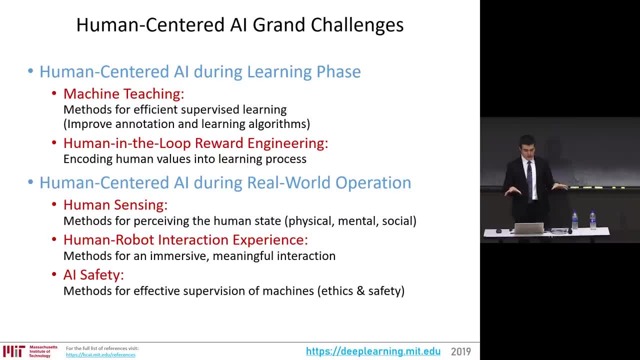 There is five areas of research, grand challenges here that define human-centered AI. I'll focus on a few today and focus on one very much so. And even with that degree of high pruning, we have 120 slides, so I'll skip around. 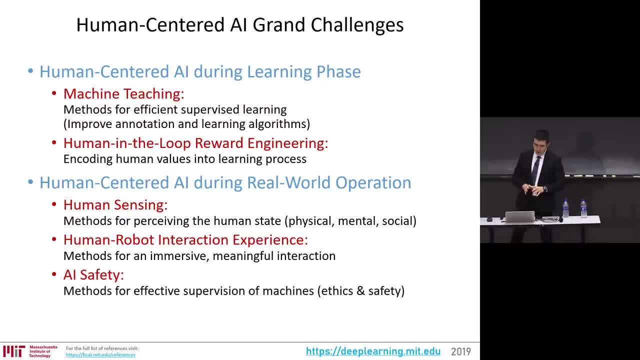 But on the human-centered AI, during the learning phase, there is the methods, the research arm of machine teaching. How do we select, how do we improve supervised learning, as opposed to needing 10,000, 100,000, a million examples? 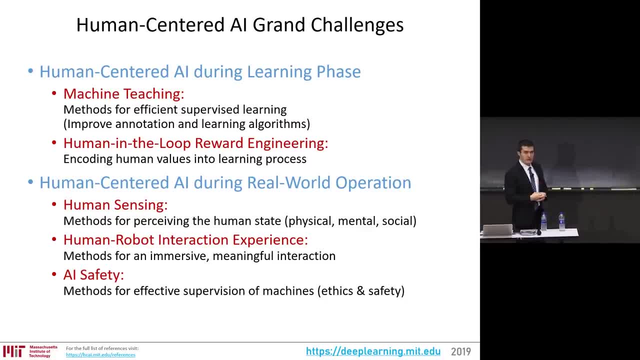 How do we reduce that, where the algorithm queries only the essential elements and able to learn effectively from very little information, from very little samples, Just like we do when we're students, when we learn fundamental aspects of math, language and so on? 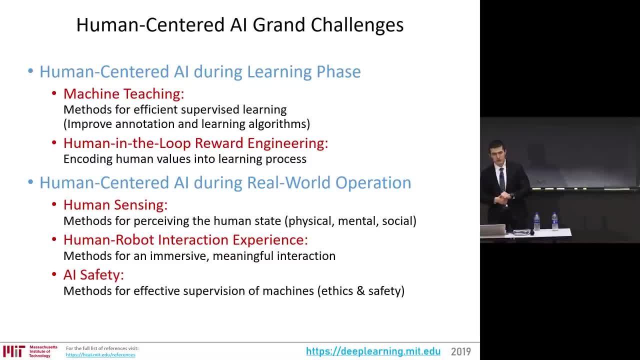 We just need a few examples, but those examples are critical to our understanding. And the second part of that is the reward: engineering That, during a learning process, injecting the human being into the definition of the loss function of what's good, what's bad. 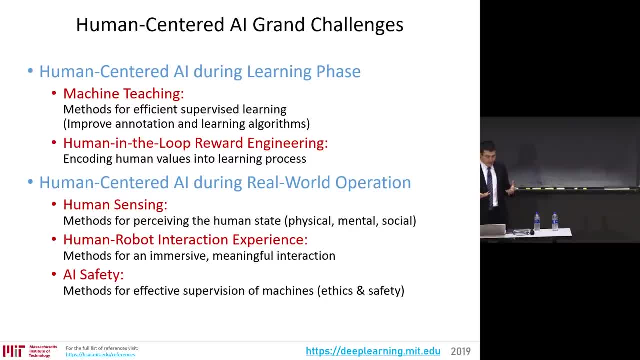 Systems that have to operate in the real world have to understand what our society deems as good and bad, And we're not always good at injecting that at the very beginning. There has to be a continuous process of adjusting the rewards, of reward re-engineering by humans. 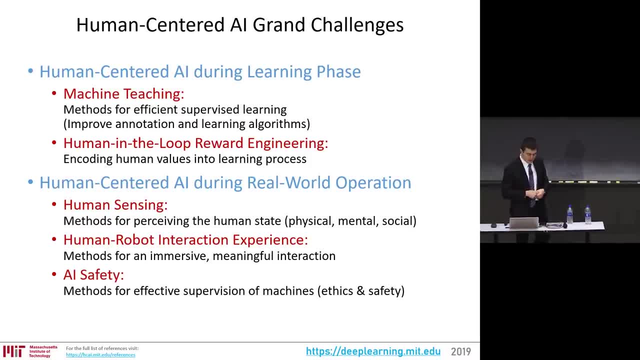 so that we can encode human values into the learning process. Now on the second part, on the human-centered AI. during real world operation, when the system is actually trained, there is the, there is the interactive element of robots and humans working together. 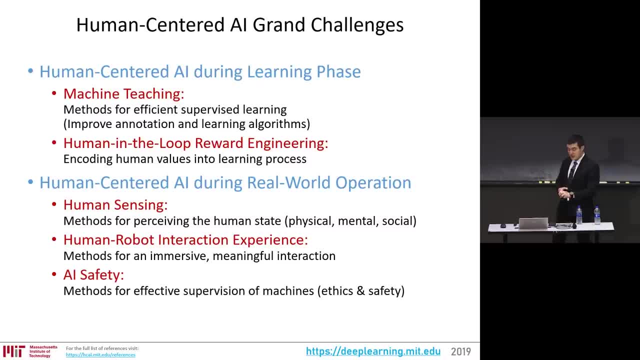 That means the part I'll focus on quite a bit today because there's been quite a lot of development and progress on the deep learning side- is human sensing, is algorithms that understand the human being, Algorithms that from taking raw information, whether that's video, audio text, 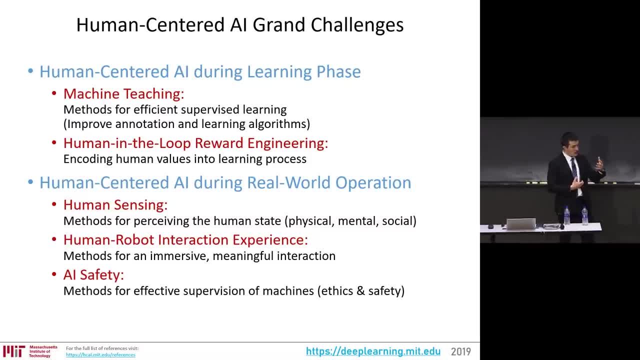 begin to get a context, a measure of the state of the human being, the short term and the long term over time, the temporal, the temporal understanding and the instantaneous understanding. Then there is the interaction aspect. So once you understand the human, 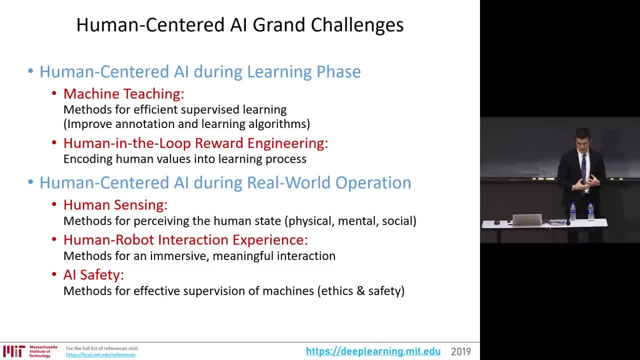 the perception problem. you have to interact with them And interact in such a way that is continuous, collaborative and a rich, meaningful experience. That's a we're in the very early days of creating anything like rich, meaningful experience with AI systems. 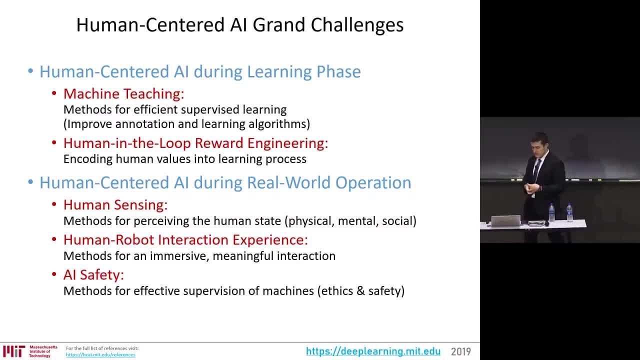 especially learning-based AI systems And safety. The real-world operation safety ethics unrolling the results of the engineered rewards that were in place during the learning process now come to fruition, And we need to make sure that the train model does not result in things that are. 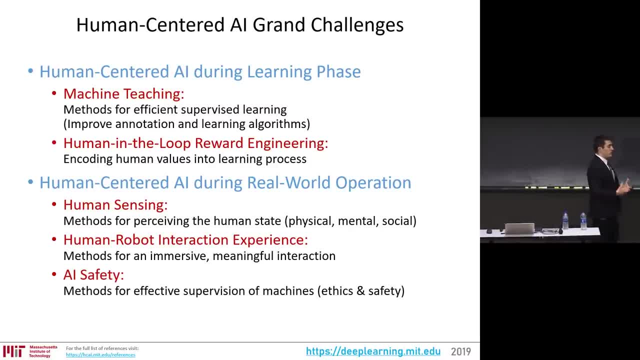 that are highly detrimental, catastrophic to our safety or highly detrimental to what we deem as good and bad in society, of discrimination, of ethical considerations and all those kinds of things. The gray area, the line we all walk as a society in the crowd: intelligence. 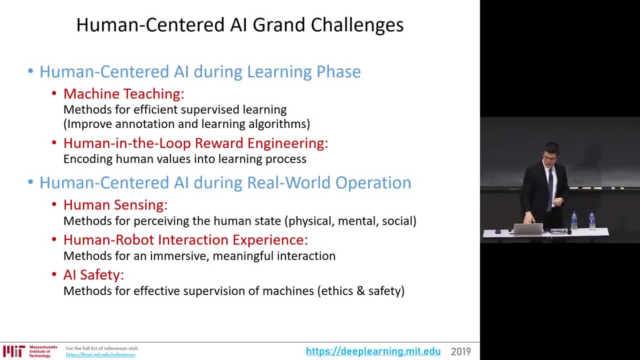 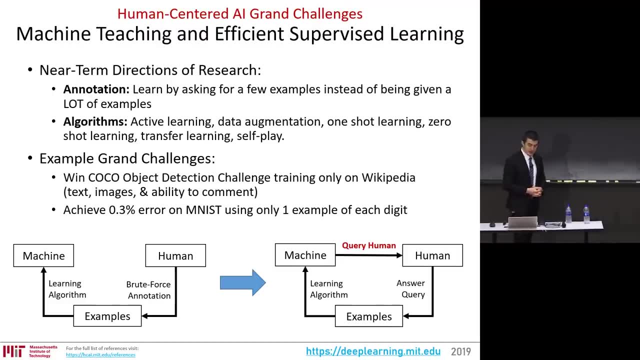 We have to provide bounds on AI systems and there's an entire group of work and I'll mention what we're doing in that area. So first, on the machine teaching side and the efficient supervised learning, I'd like to sort of do one slide on each of these. 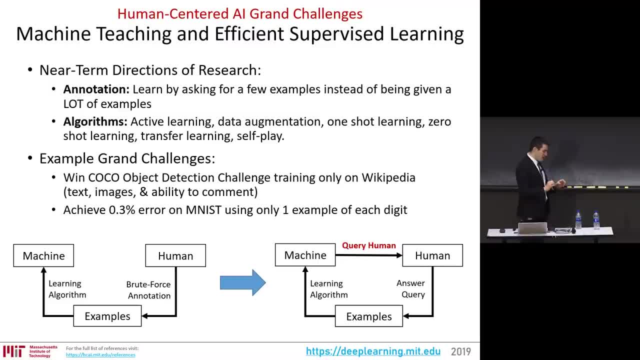 to kind of give you an idea Near term and do two things for each area that we will elaborate in future lectures on, and some of it I'll elaborate today. First, the near term directions of research, the things that are within our reach now. 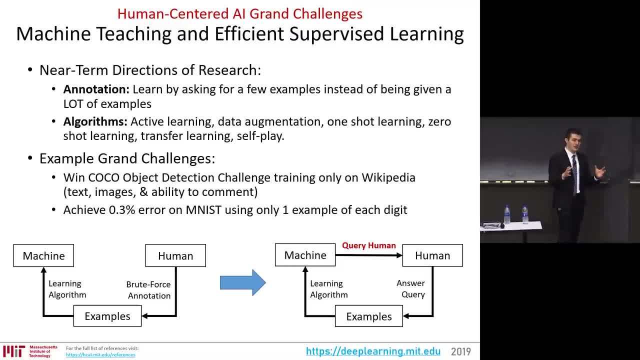 and a sort of thought experiment and a grand challenge that if we can do it that would be damn impressive. That would be a definition of real progress in this area. So near term directions of research for machine teaching, for improved supervised learning, integrating the human into the annotation process. 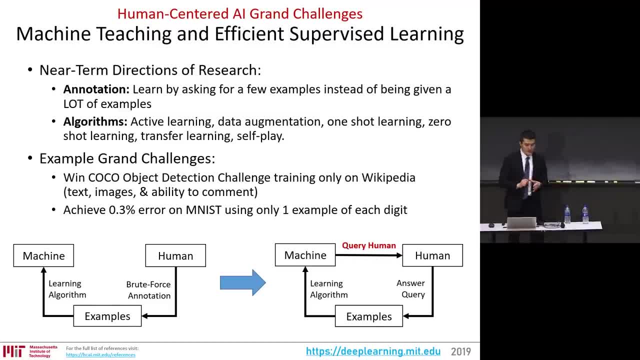 is, instead of annotating, brute force is annotate by asking the human questions. So we have to transform the way we do annotations, where the process of annotation is not defining the data set, and then you go through the entire data set. It's a machine teaching system. 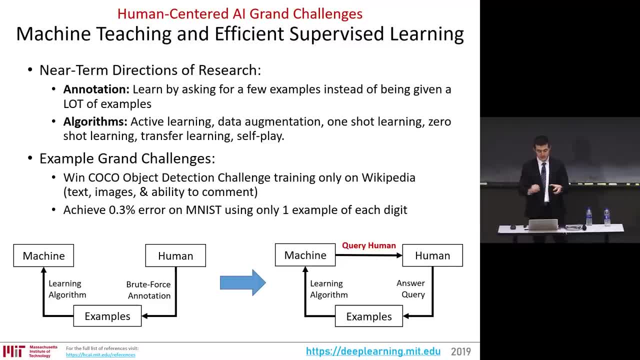 that queries the user for questions to annotate, And, on the algorithm side, active learning. these are all sort of areas of work where we can be more clever about the way we use data, select data on which to train. So active learning is actively selecting. 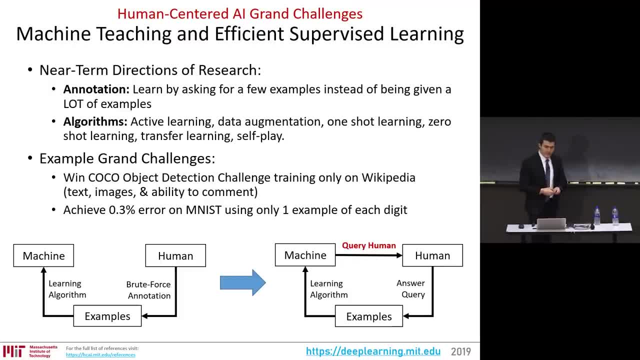 during the training process, which part of the data to train on And you can annotate Data augmentation is taking things that have been supervised by a human and expanding them. Modifying the data, warping the data in interesting ways such that it expands. 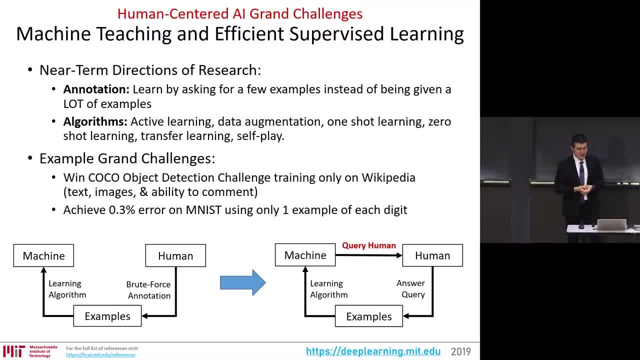 it multiplies the human effort that was injected into helping understand what's in the data. The one shot learning, zero shot learning and transfer learning are all in that category, And self play is in the reinforcement learning area, where the system constructs a model that is self made. 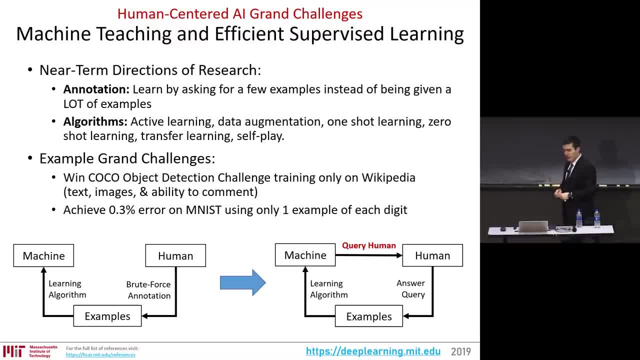 Again a protein system, Again a protein system And again a protein system model of the world and goes along alone in a room and plays with that model to try to figure out the different constraints of the model. how do you achieve good things there? 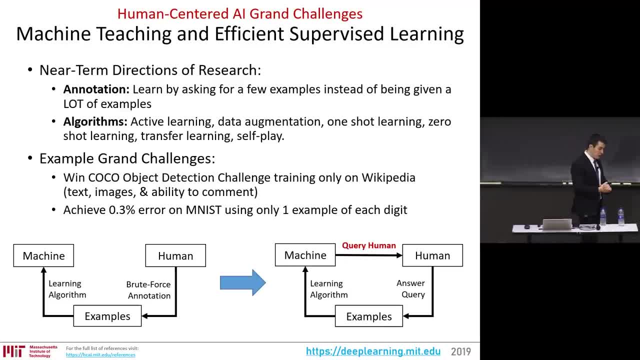 An example: grand challenge here that would define serious progress in the field is, if we take ImageNet or COCO- the ImageNet Challenge or COCO Object Detection Challenge- and training only on a totally different kind of data, be able to achieve state-of-the-art results. 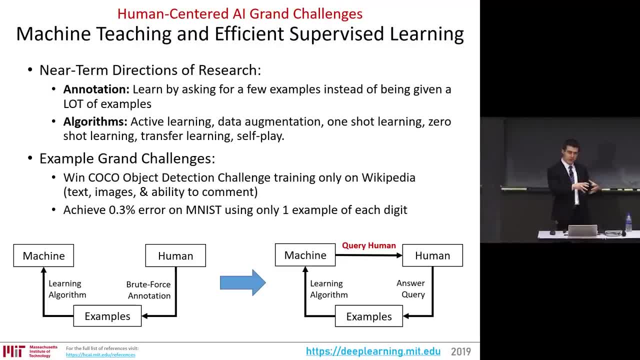 So training only on Wikipedia, with the text and images that are there on Wikipedia, be able to perform object detection on the state-of-the-art benchmark of COCO. The COCO is a data set of different objects with rich annotation of the localization of the objects. 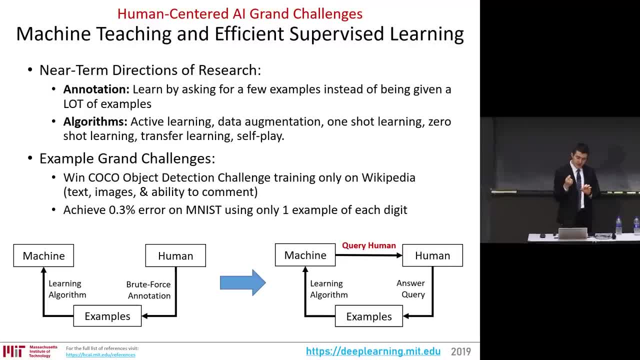 That, I believe, is exactly the kind of thing that all the problems in the transfer, learning and efficient data annotation, machine teaching, have to be solved to achieve that. Another way to another challenge you can think of if we could even just simplify it more. 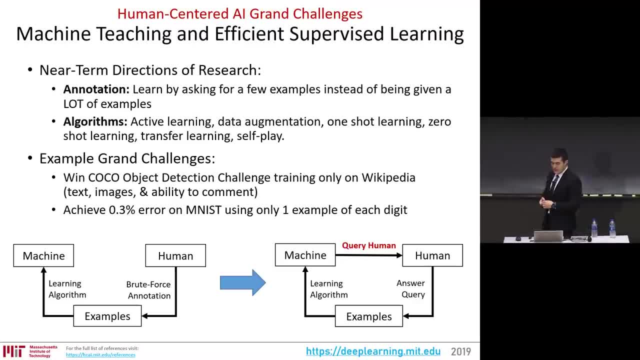 is: achieve 3%- 0.3% error on MNIST. that's the handwritten recognition task that everybody always provides as an example. So achieve a very good accuracy, state-of-the-art accuracy, by training only on a single example of a digit. 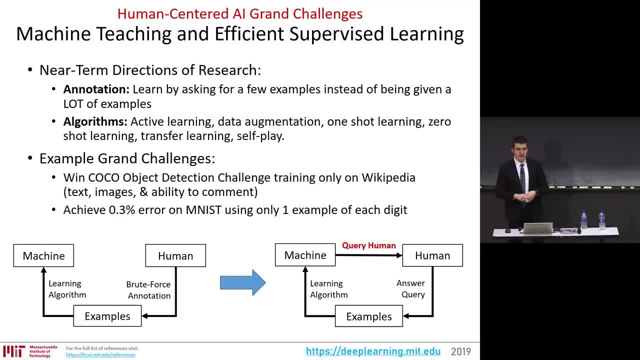 As opposed to training on thousands. training on one example. That's something that most of us humans can do: given one example of a new language you haven't seen before for each character, after studying them for a little bit, be able to now classify future characters at high accuracy. 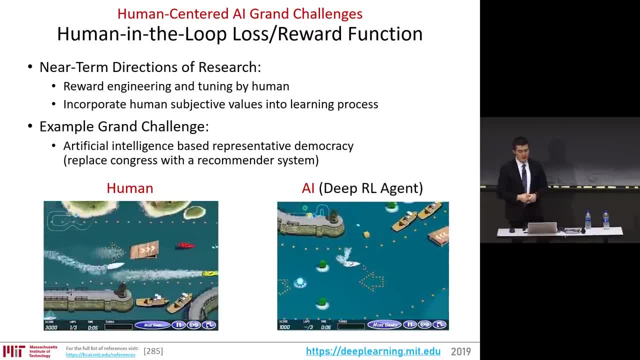 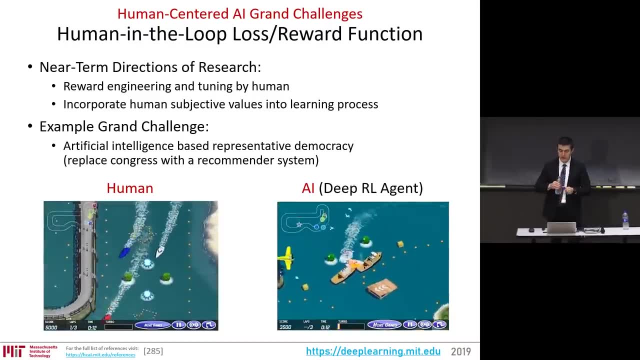 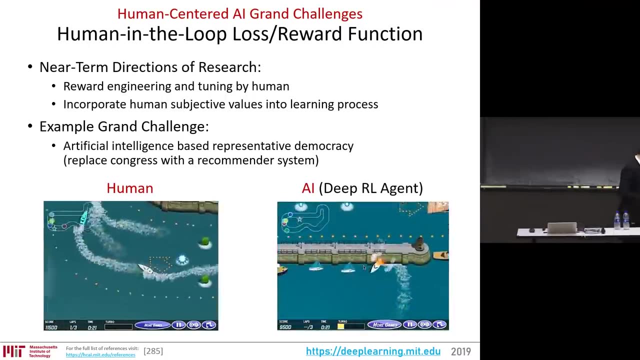 The second part of the learning process, where the human needs to be injected, and then near-term directions, the research. there is the reward engineering And the tuning of those, continuous tuning of those rewards by a human being. So OpenAI is doing quite a bit of work here. 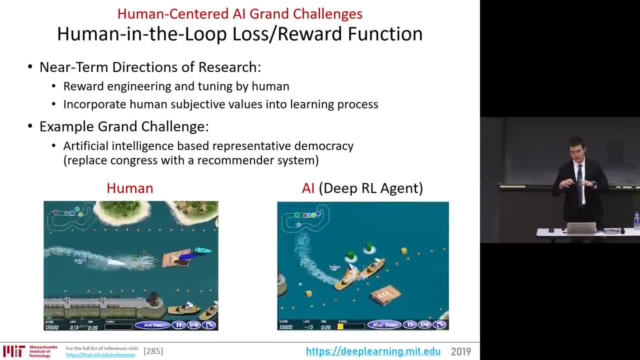 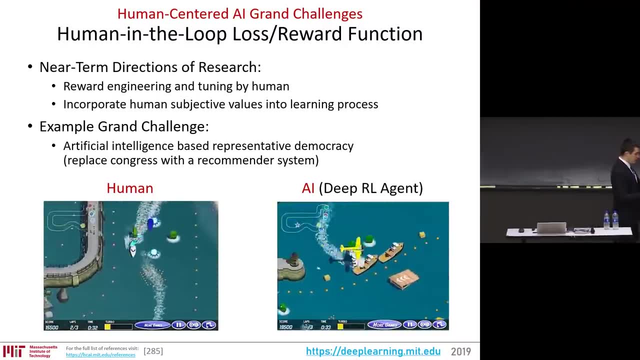 Here's a game played by human and AI, and it's really my favorite example of this. On the left, human is controlling a boat that's finishing a race. On the right is a RL agent- reinforcement learning agent- that's controlling a boat. 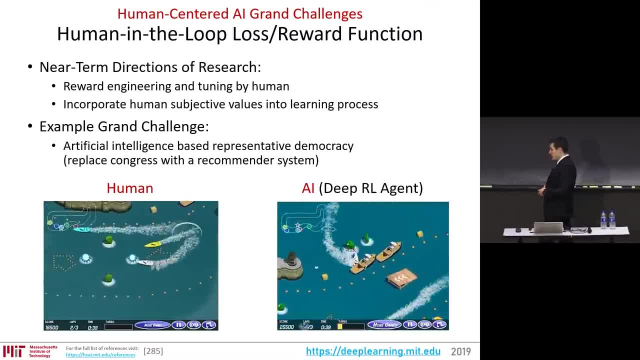 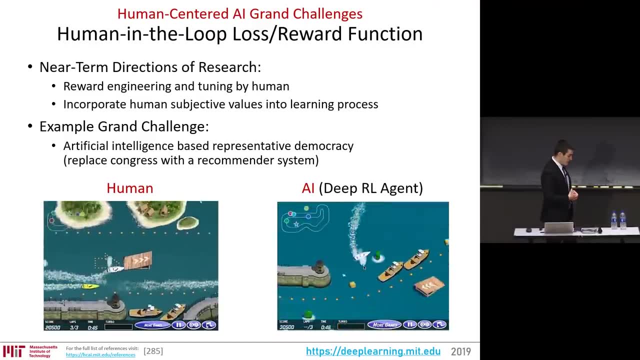 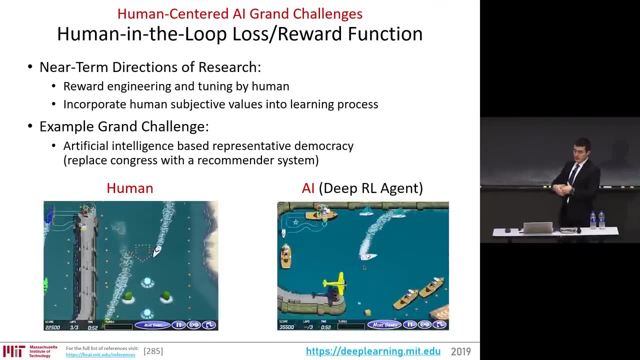 that's trying to not finish a race, trying to maximize the reward defined prior to by- initially by a human being, And what it finds is that you can get much more reward by collecting green turbos that appear as opposed to finishing the race. 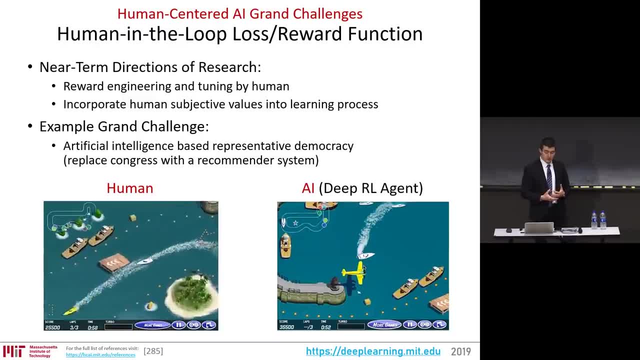 It realizes that finishing the race actually gets in the way of maximizing your reward, And so that's the unintended consequences of a reward function. that was that was specified previously, and most human supervisors of this result would be able to adjust, through the re-engineer, their reward function. 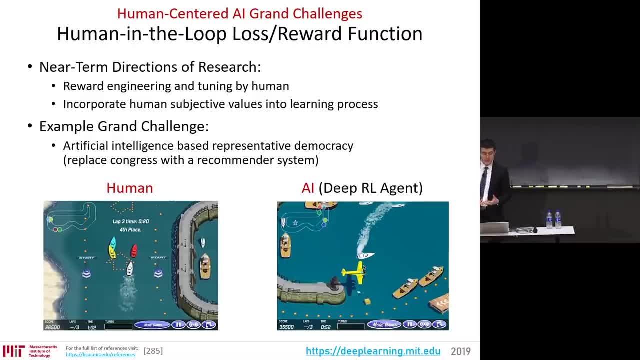 to be able to get the robot to the AI system here to finish the race, And that kind of continuous monitoring, monitoring of the performance of the system during the training process, is a near-term direction of research. that's a few DeepMind, OpenAI. 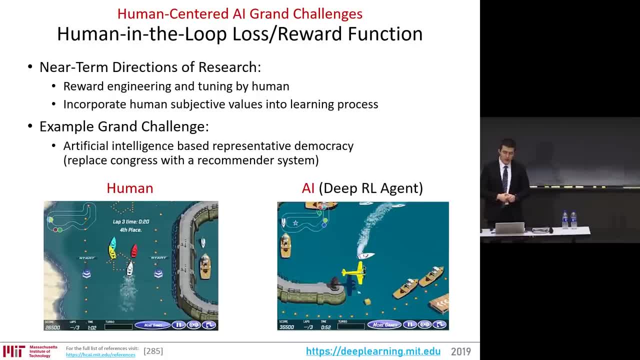 and ourselves are taking on Example. grand challenge is allowing AI system to operate in a context where there's a lot of fuzziness for us humans. There's a lot of uncertainty, There's a lot of gray area, There's a lot of challenging aspects in terms of 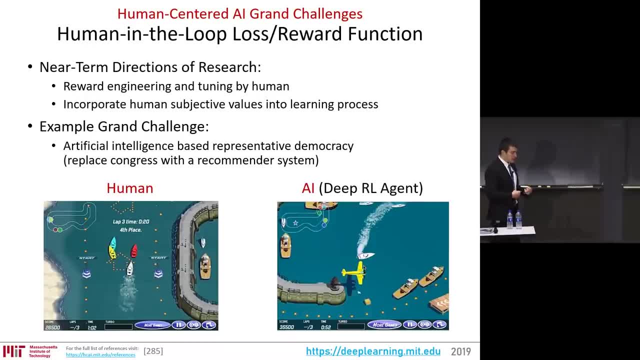 what is right and what is wrong that we continually need to improve on. Example I provide here is: one of the least popular things in the world is the US Congress, So replacing US Congress. it's a body of representatives of the people. 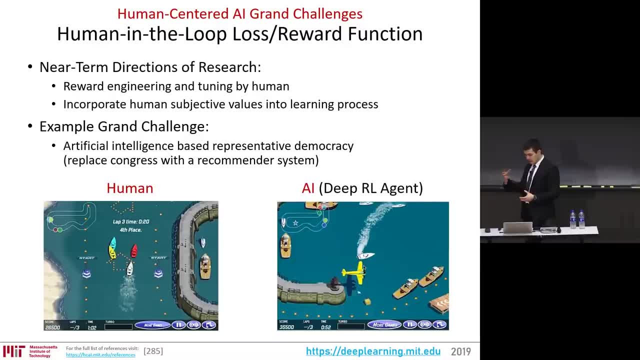 of the United States and they make bills based on the belief of the people That you know. that sounds a lot like what Netflix does in recommending what movies you should watch next, in representing what people love to watch. So it's just a recommender system. 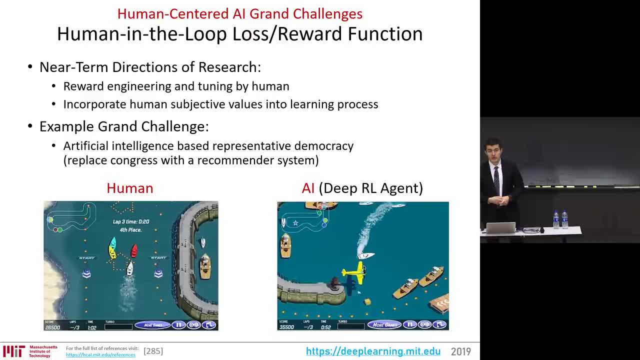 So it makes perfect sense that an AI system should be able to take on this challenge, And that would I see that as a grand challenge- is replacing some of the fundamental representation of large crowds of people that make ethical decisions, replaced by a human-centered AI system. 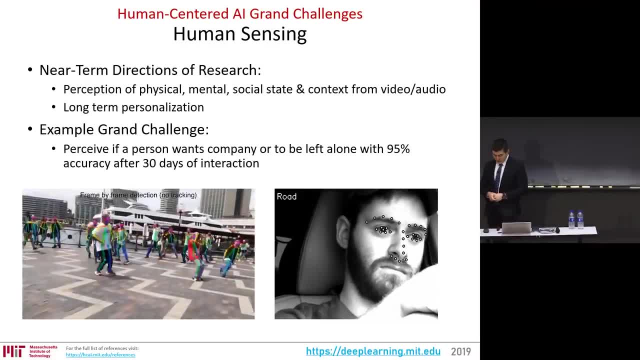 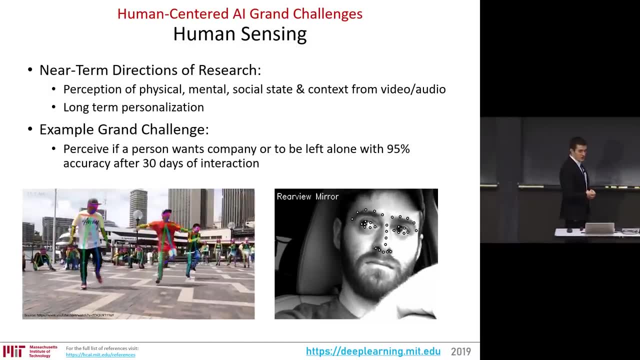 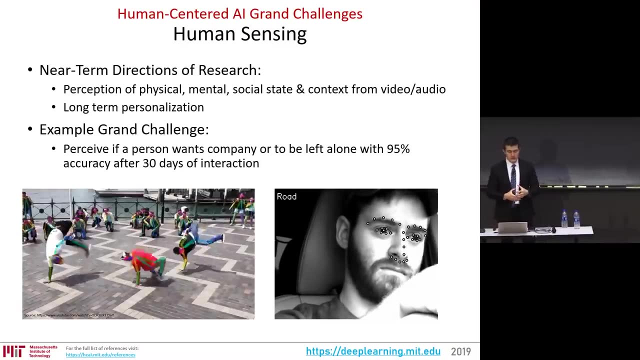 Okay, in real world operation, the first thing we have to do before we have a robot and a human work together. the first thing is the robot has to perceive the human Question. The question was: do you want to? so there's currently there's a Congress. 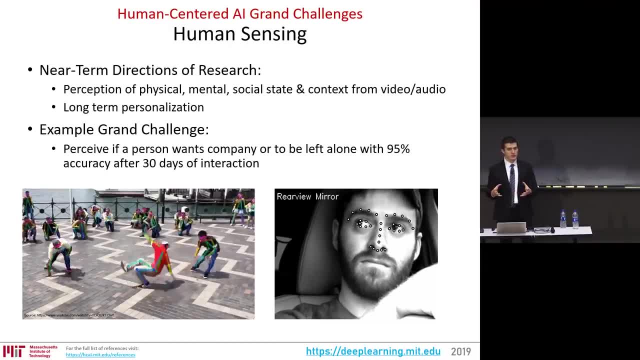 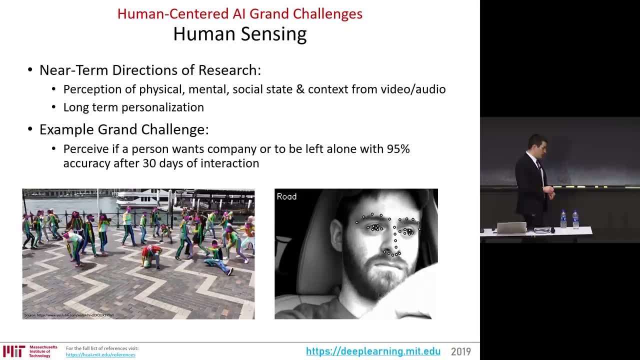 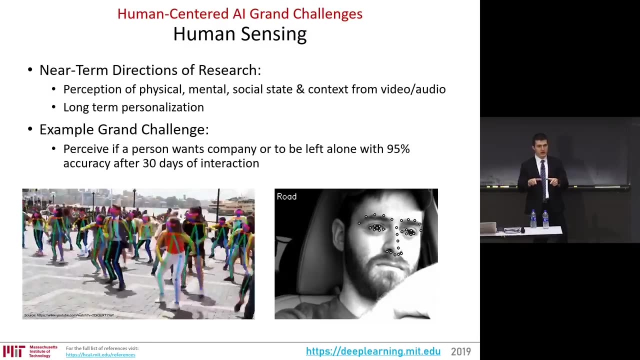 do you want to change the way Congress works, make it better, or do you wanna just take the system that currently is and automate it? So the idea is: take the system as it currently is supposed to be and automate that. So an AI system can provide a lot more transparency. 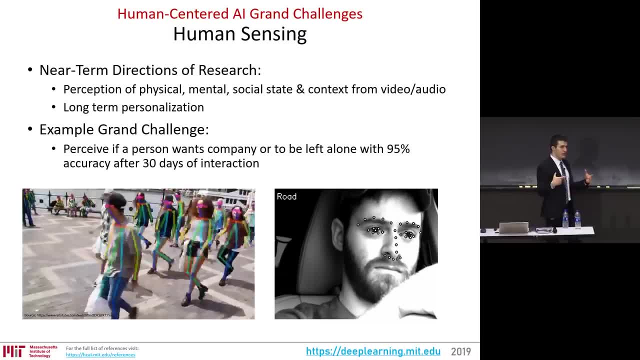 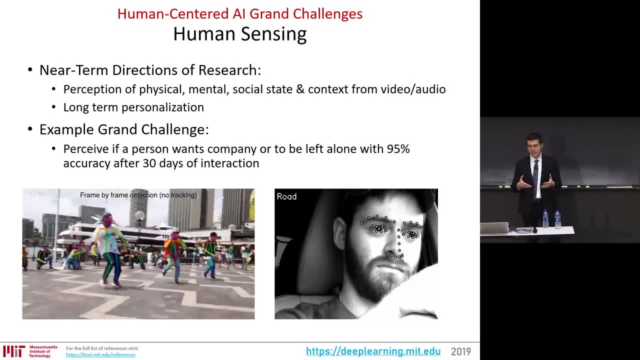 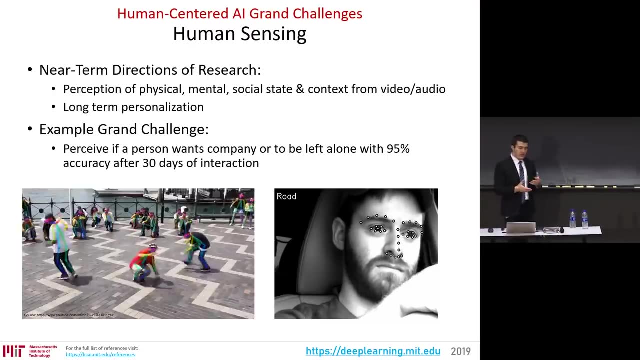 of the inputs, The idea of Congress. the only inputs is supposed to be the people and the beliefs of the people, And there's also- but that's- rich information there. So, for example, I mean the input for me not saying anything, politics. 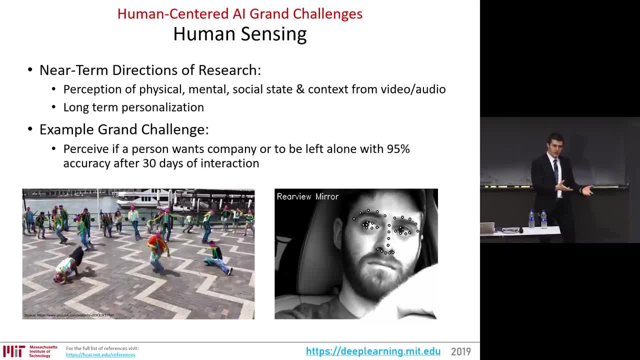 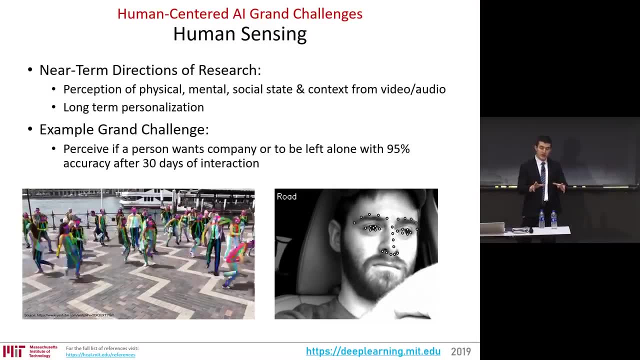 but there's certain issues I care a lot about, certain issues I care a lot about and certain issues I care a lot about that I don't care much about and put that aside. And then there's certain issues that I know a lot about. 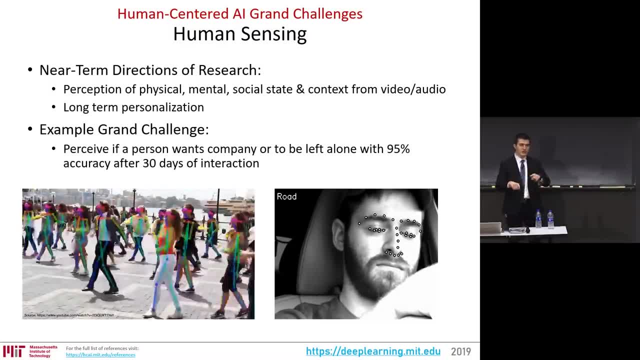 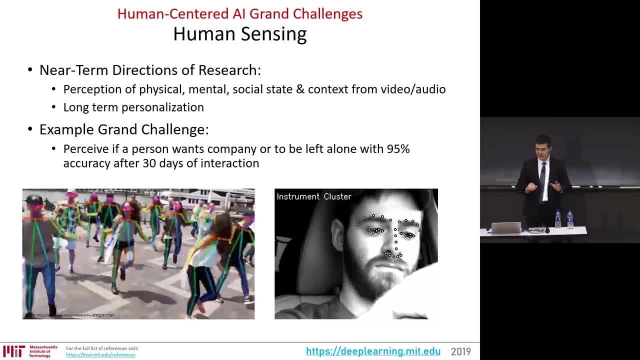 and certain issues I know very little about And those don't actually intersect that well. I'm very opinionated about things I don't know anything about. it's very common all of us are So being able to put that representation of me into a system. 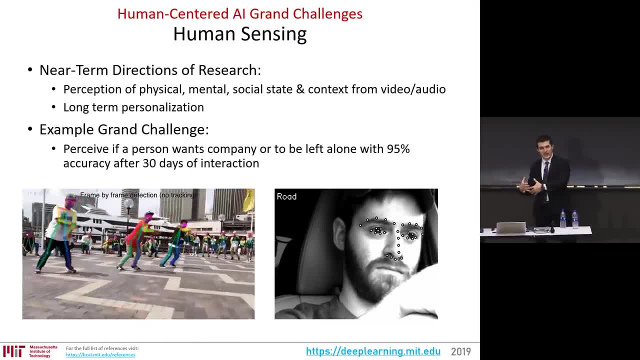 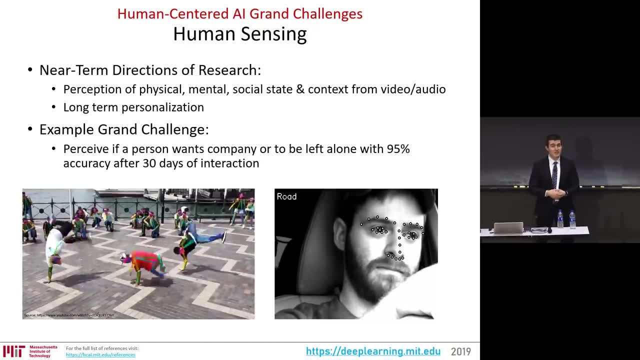 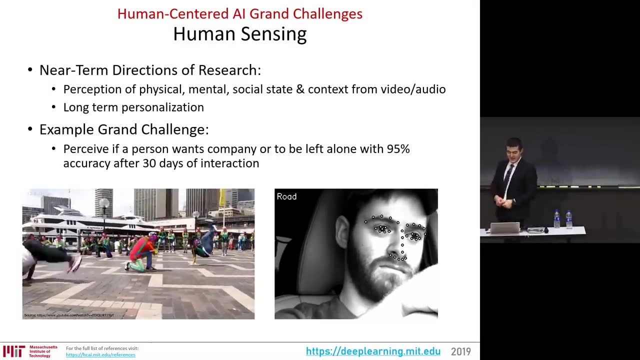 that would take a lot of our entire nation together and be able to make bills that represent the people. Now the challenge there. it can't be just the training set and then the system now operates. AI is running the country. No, there has to be that human-centered element. 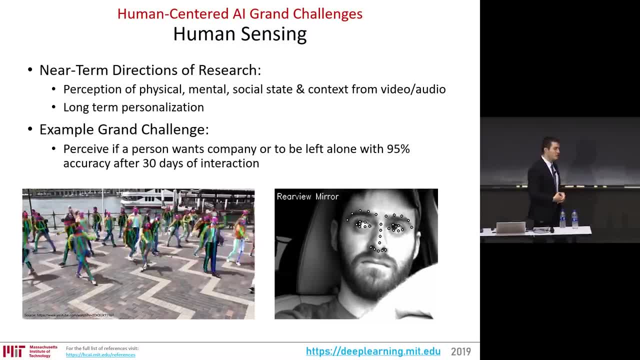 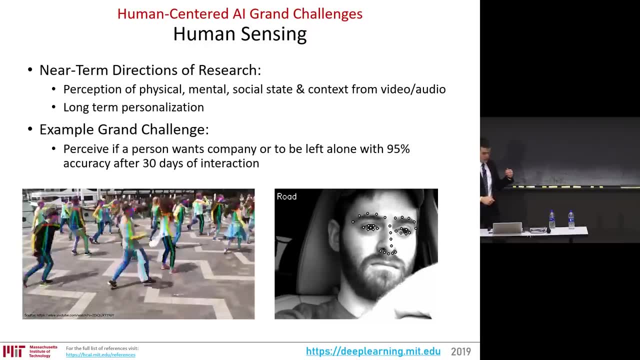 where we're constantly supervising, just like we're, in theory, supposed to be supervising our congressmen and congresswomen. Human sensing- the first part: in order to have an AI system that works with a human being, the AI system has to perceive, understand. 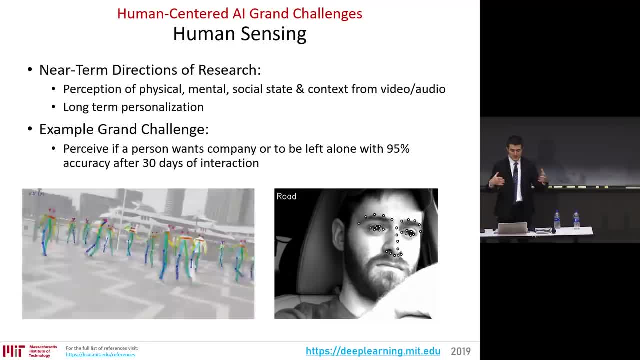 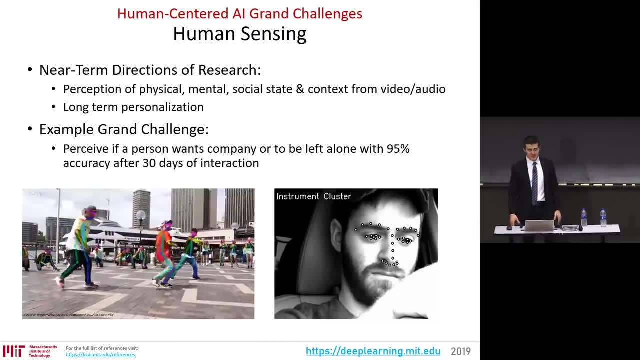 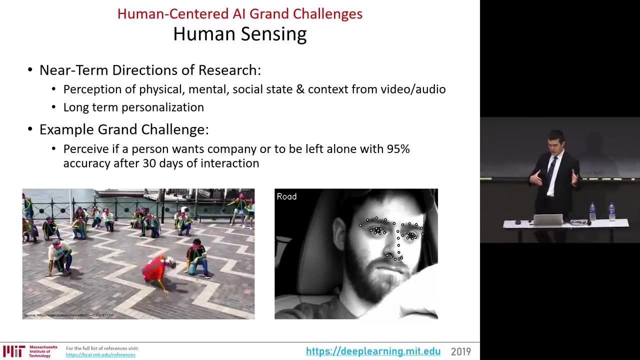 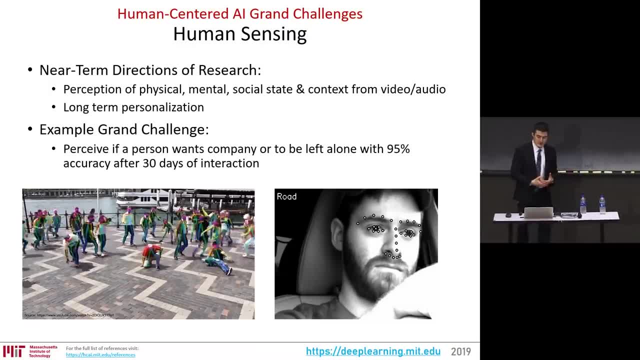 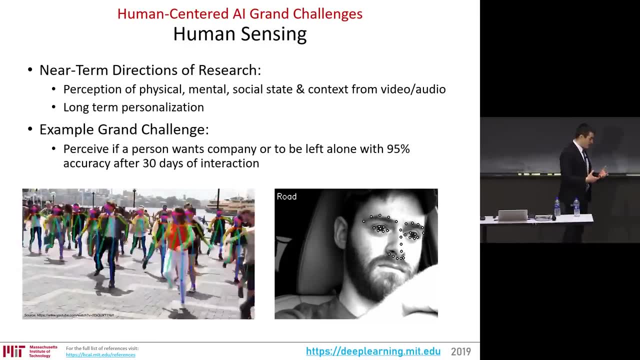 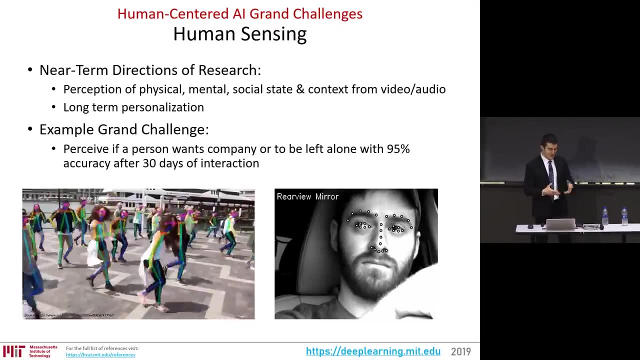 the physical, mental, social state, social context of the person, Be able to everything, and this is what I'll cover a little bit of today: everything from face detection, face recognition, emotion recognition, natural language processing, body pose estimation. 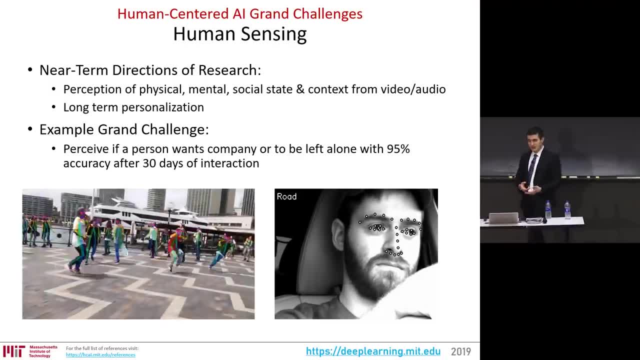 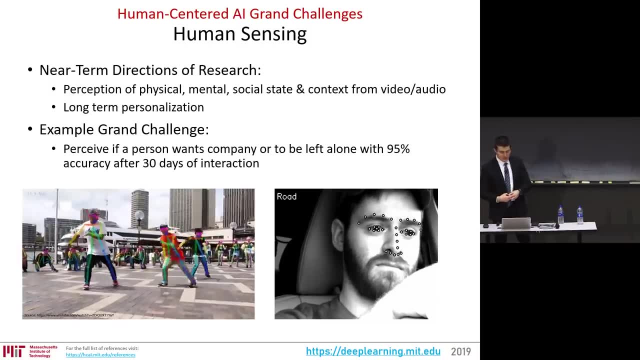 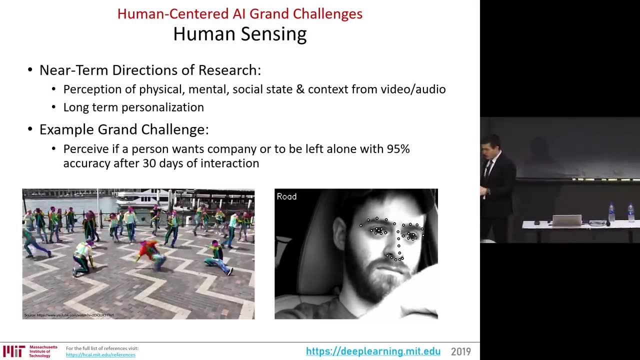 those same recommender systems, speech recognition, the all of those conversions of raw data capture something about the human being into actually meaningful, actionable information. The grand challenge there is emotion recognition. You know there's been a lot of companies and ideas. 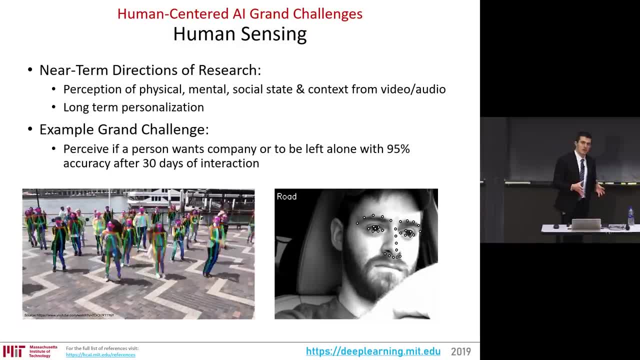 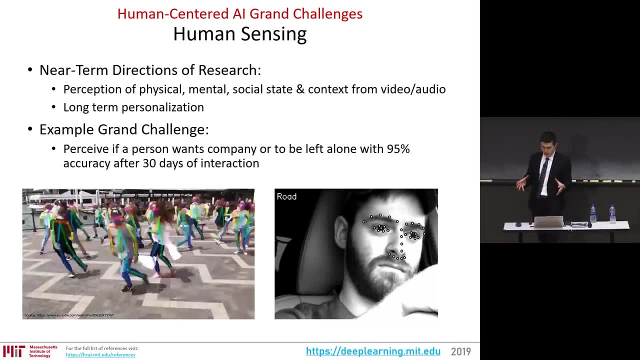 that we've somehow cracked emotion recognition, that we are able to determine the mood of a person. But really that's for those who were here last year with Lisa Feldman Barrett. but just if you're sort of very honest and you know, 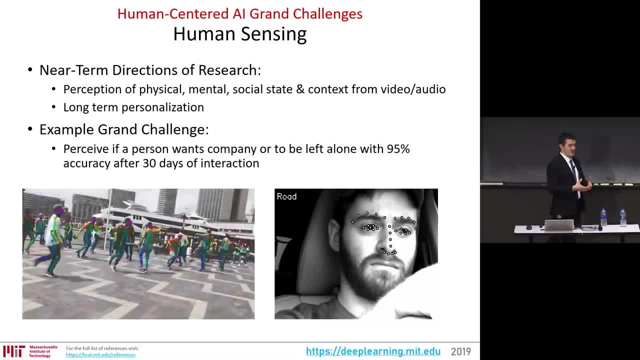 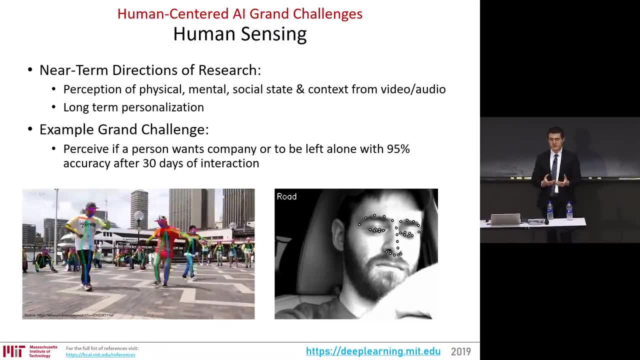 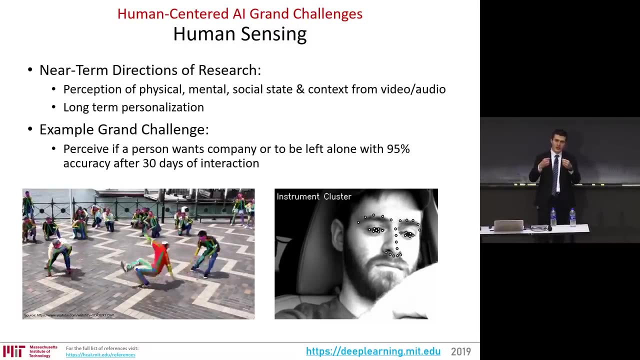 you study emotional intelligence and emotion and the expression of emotion. it's a fascinating area, and we're not even close to being able to build perception systems that detect emotion. What we're more so doing is detecting very simple facial expressions that correspond. 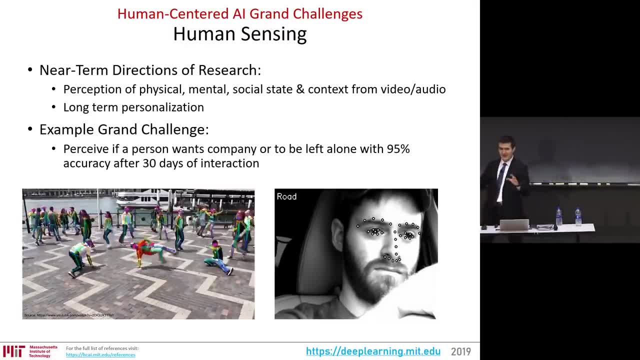 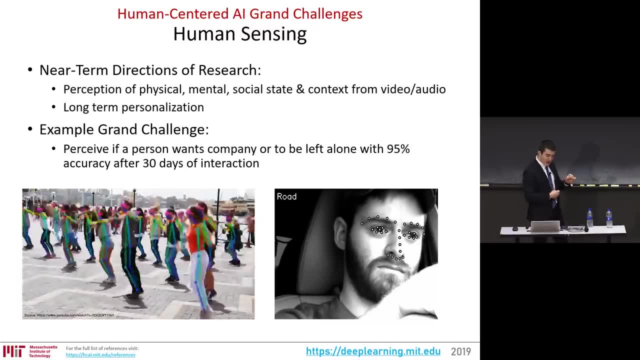 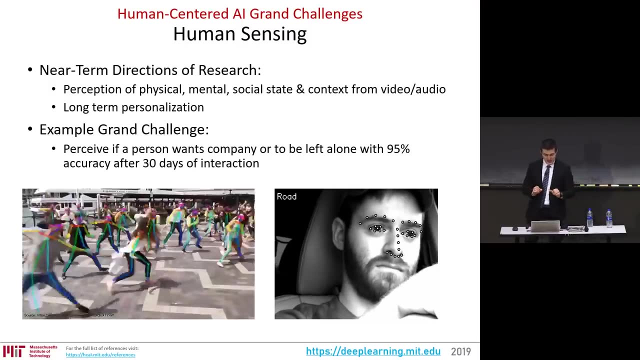 to our storybook versions of emotion: Smiling, crying, like frowning, in a caricatured way. So if you build a system that has a high accuracy of doing real emotion recognition, you can think of it as stated here. 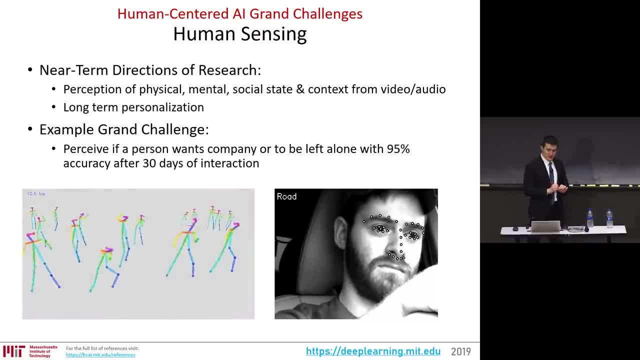 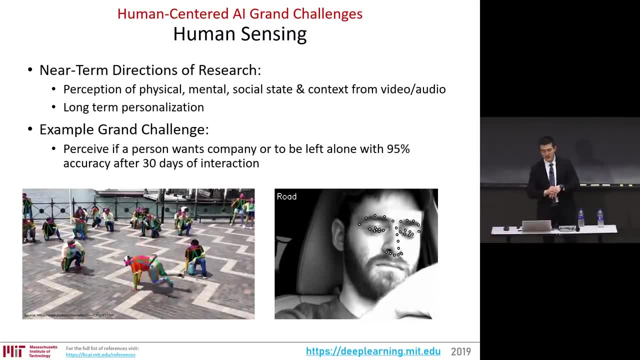 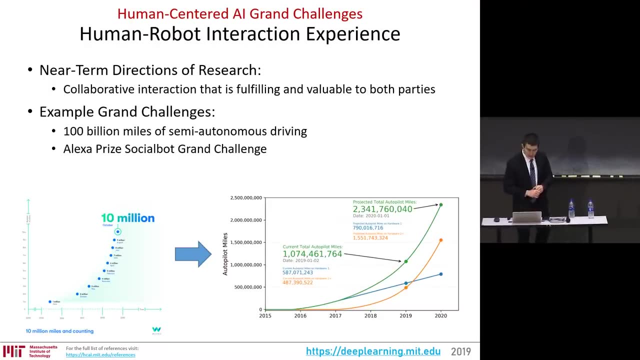 an AI system that classifies binary classification problem with 95% accuracy of whether you want to be left alone or not, And being able to do that after collecting data for 30 days. that I see as a really clean formulation of exactly some. 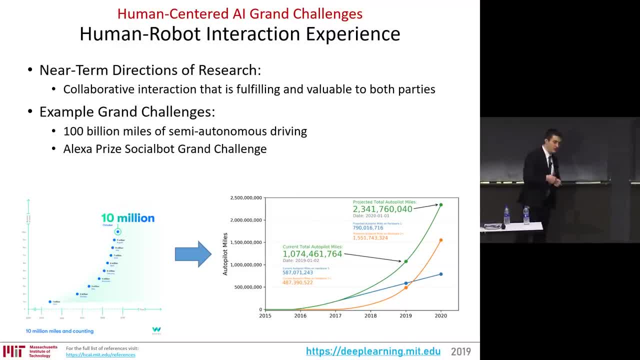 exactly the kind of human understanding we need to be able to build In our learning models, and we're very far away from that, especially the long temporal aspect of that of being able to integrate data over a long period of time. Then the second part of human robot interaction. 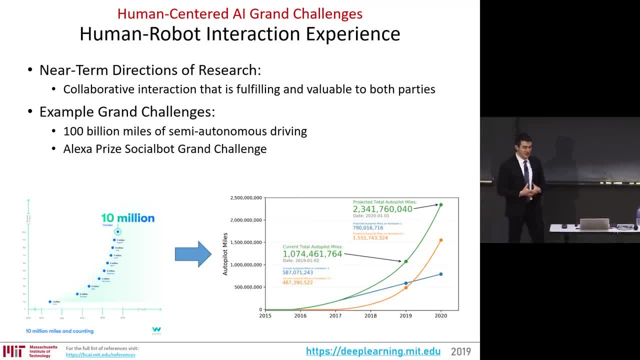 in the real world. operation is the experience. This is where we're now just beginning to consider that interactive experience of how do we have a rich, fulfilling experience? We have autonomous vehicles, for example, semi-autonomous vehicles, whether that's Tesla, Volvo, Super Cruise with the Cadillac. 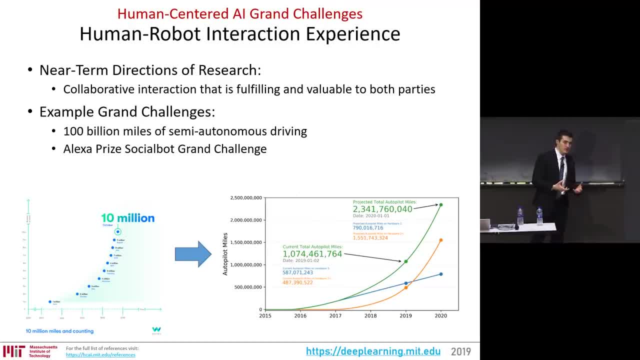 There's a bunch of systems that have now greater and greater degrees of automation in the car and we get to have the human interact with that AI system and trying to figure out. how do we have a rich, fulfilling experience In the- currently the Volvo system? 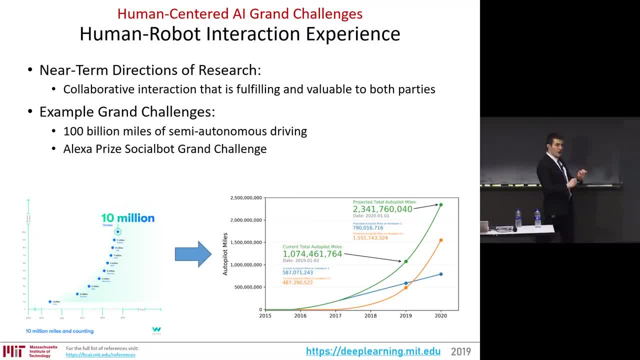 that experience is more limited. There's a little icon. it's more kind of traditional driving situation. There's a little icon. it's more kind of traditional driving situation. There's a little icon. it's more kind of traditional driving situation. 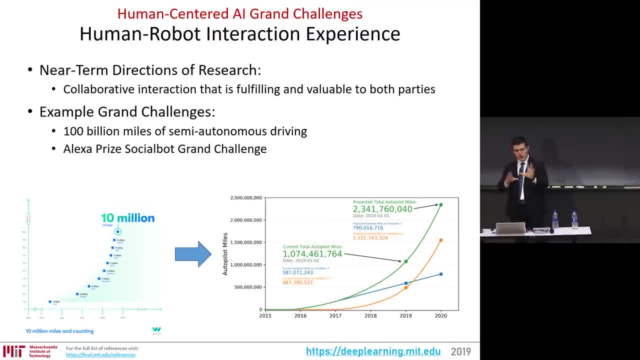 In the Tesla, you have a much bigger display about what's going on. In the Super Cruise, there's a camera looking at your eyes. In the Cadillac Super Cruise system, there's a camera looking at your eyes, determining if you're awake or not. 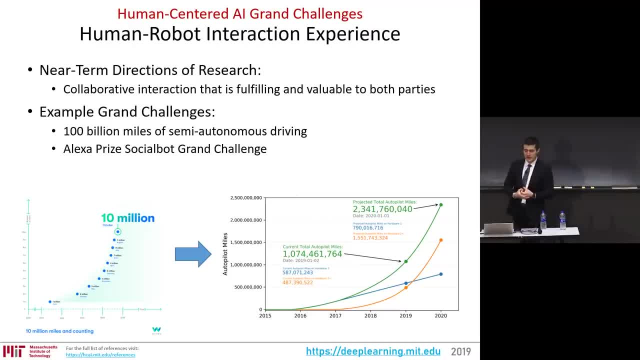 or paying attention or not, And that there's like an experience there that we're trying to create And in the Tesla case, the miles are racking up. We have real data. Here at MIT we're studying this exact interaction. 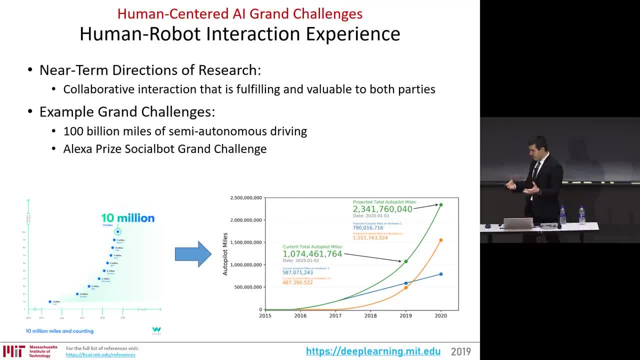 Over a billion miles driven in the Tesla And the same in the fully autonomous side with Waymo. they've now reached 10 plus million miles driven autonomously And there's a lot of people experimenting with this. But that's that collaborative interaction. 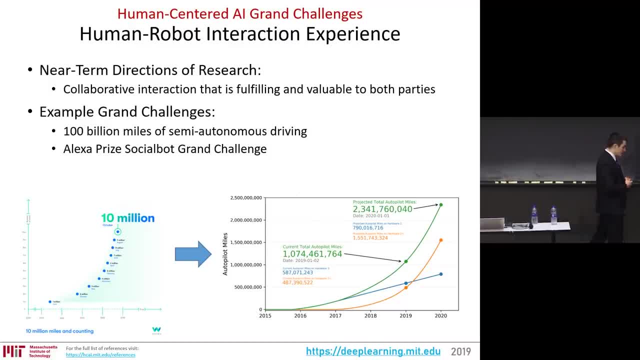 of going back and forth, of being able to for the AI system to express the degree of uncertainty it has about the environment, The AI system being able to express when it needs help and not be able to communicate- what are its limitations and capabilities, and so on. 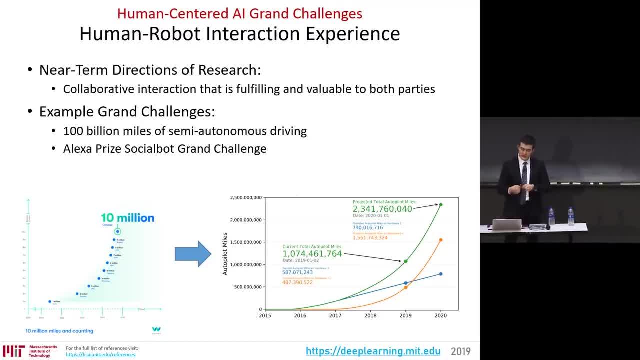 Trade off control, be able to seek human supervision. There's a dance there that's really- that takes into consideration everything from the neurobiological research to psychology, to the deep learning, to the pure robotics, HR or HRI- human robotic interaction aspects. 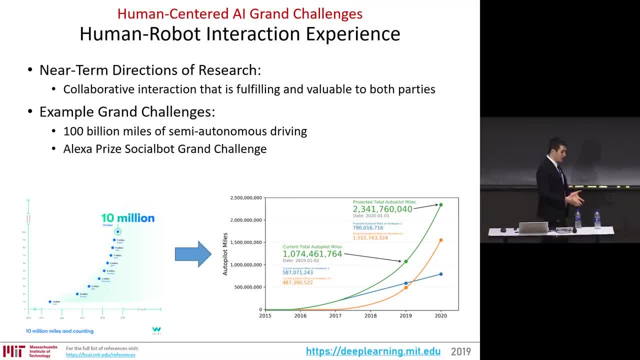 One grand challenge would be: you know, Tesla's driven 1 billion miles now under autopilot, under the semi-autonomous mode. The grand challenge here is when we start getting to the kind of mileage that we see in the United States every year. 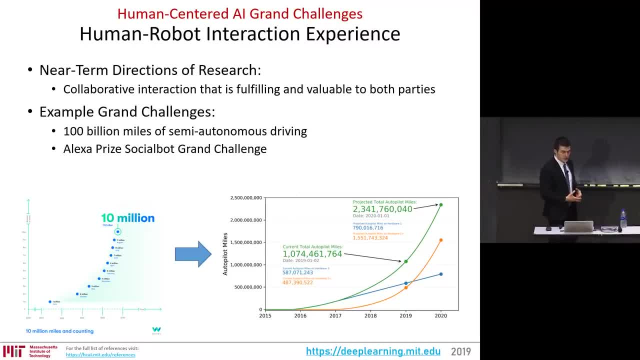 you start getting into the hundreds of billions of miles driven semi-autonomously. We get to see teenagers- 16,, 17,, 18, using these systems for the first time. We get to see older folks, folks who don't necessarily drive. 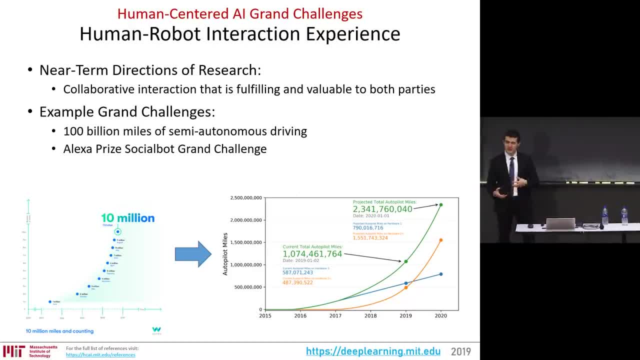 or use any kind of AI in their lives, get to use these systems. We start to explore that aspect. That's the real challenge. And, of course, the Turing, the old Turing test, now re-imagined by Alexa with the Alexa Prize challenge. 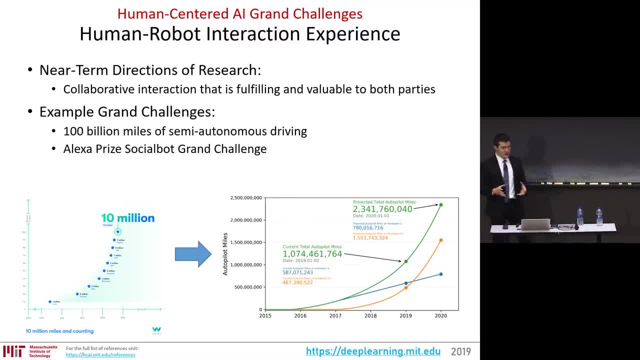 of social bot is creating natural language is such a beautiful thing to explore. human robot interaction with is both on the audio side and just the tech side is passing the Turing test. That's a true grand challenge in a real way, where you wanna have a conversation with a robot. 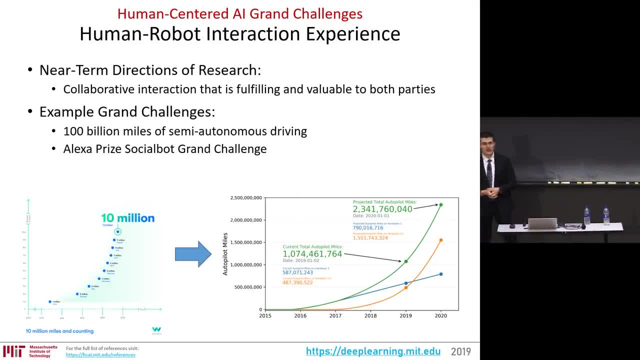 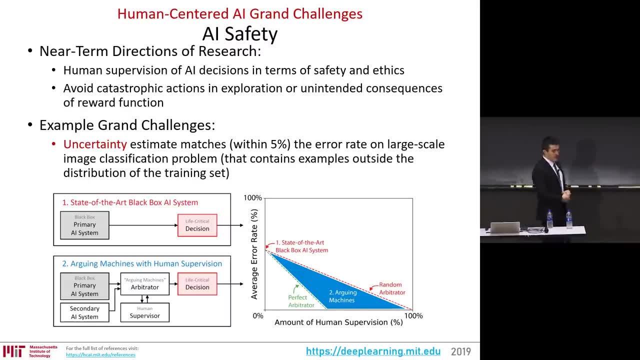 for prolonged periods of times, maybe more than even some of your other friends. And on the other side of friends is the risk, the catastrophic risk that's potential when you have an AI system that's learning from data. The near-term directions of research. 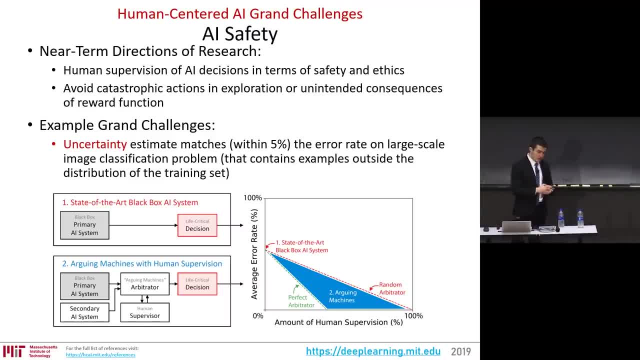 is purely the human supervision of AI decisions in terms of safety and ethics. There's a lot of systems, like with cars or medical diagnosis and so on, where there's some life critical, safety critical aspect that we want to be able to supervise the safety of that. 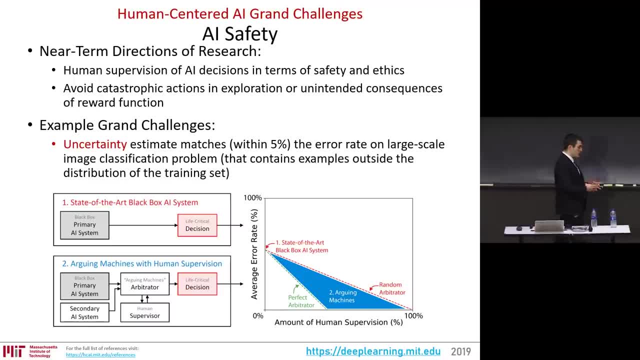 And there's ethical decisions in terms of who gets a loan or not, who gets a certain criminal penalty or not, the any degree to which AI systems are incorporated into that. you have to consider ethical questions And even just the crude, the low level perception systems like face recognition. 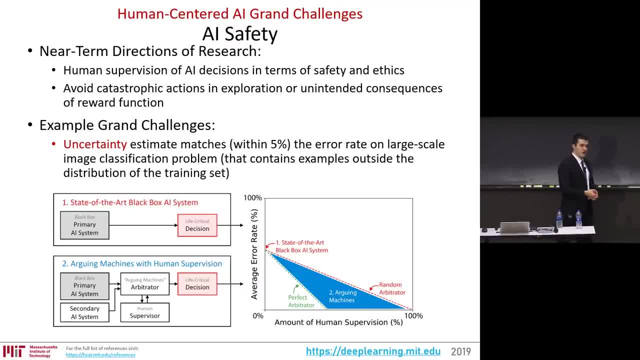 you wanna make sure that your face recognition systems are not discriminating based on color or gender or age and so on. You wanna make sure that at that basic, fundamental level of ethics, the systems are trained in a way they maintain our human values or the better angels of our nature. 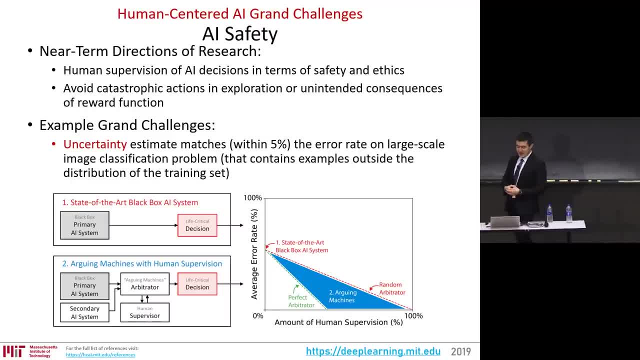 the better sides of our values, some of the brighter aspects of our values, And the other thing is in terms of just maintaining values. that's the normal, that's looking at the mean of the distribution, But we also want to do control the outliers. 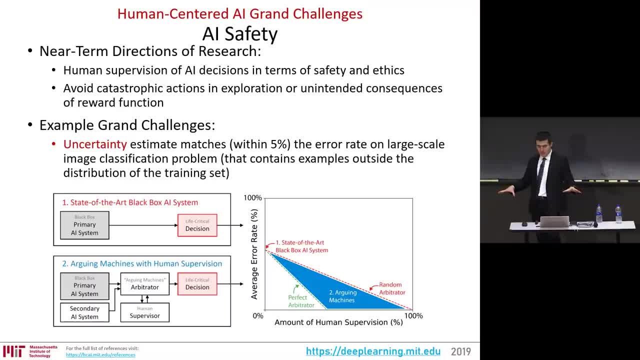 from the AI system not to do anything catastrophic. So the unintended consequences when something happens that you didn't anticipate, you wanna be able to put boundaries on that And the grand challenge there. really it all boils down to the ability of an AI system. 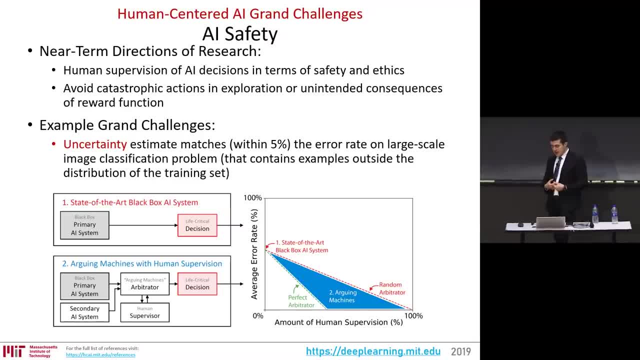 to say that it's uncertain about something, And that measure of uncertainty has to be good. It has to be able to make a prediction, always accompanied with uncertainty, even on things it hasn't seen before. That's the real challenge: to be able to be trained on cats and dogs. 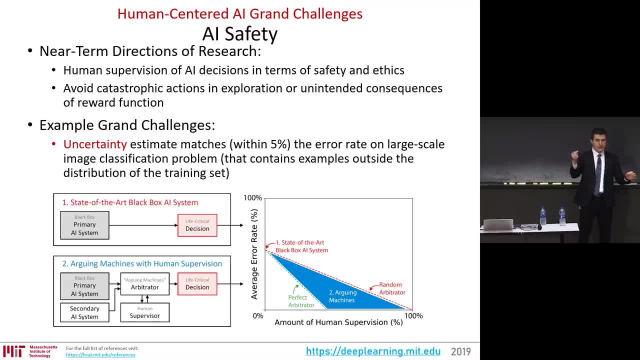 and then seeing a giraffe and saying I'm not sure what that is. We're quite far away from that, because right now it would probably confidently say it's a dog, depending on the giraffe. But we want to be able to. 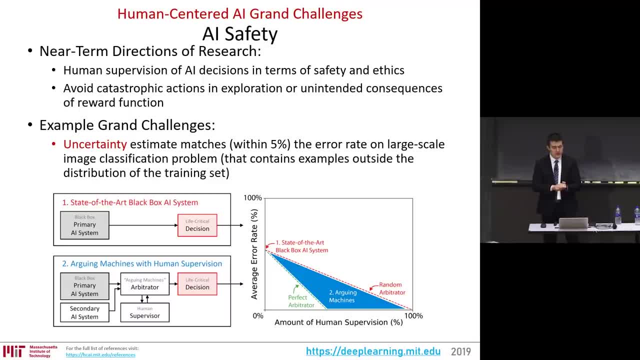 be able to have an extremely high accuracy in the ability of AI systems to determine their own uncertainty, to know what they don't know, Because from that comes the supervision, From that comes the ability to stop under things that it's uncertain about, catastrophic events. 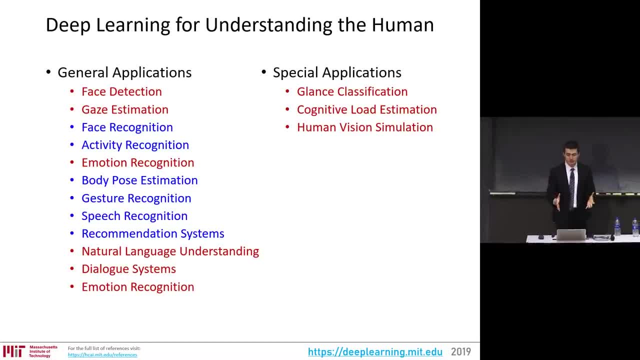 The first aspect of real world operation is understanding the human. One of the places where deep learning has really shined is the perception problem, And it all begins at the ability to look at- to look at raw data and convert that into meaningful information. 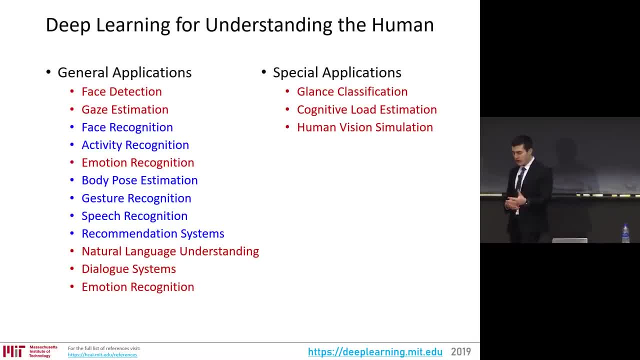 That's really the understanding the human comes in, Not the kind of understanding that when you're in a relationship with somebody, when you're friends with somebody over a long period of time, you gain an understanding of their quirks, limitations, capabilities, so on. 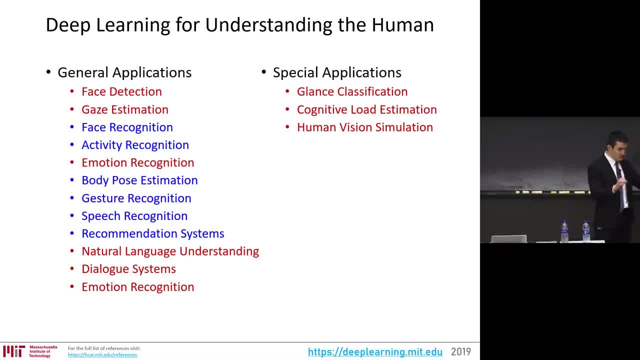 That's really fascinating, But the first step is to just to be able to, when you see them, recognize who they are. what's on their mind, what's their, the body language, the, what are they saying with their mouth, all those basic raw perception tasks. 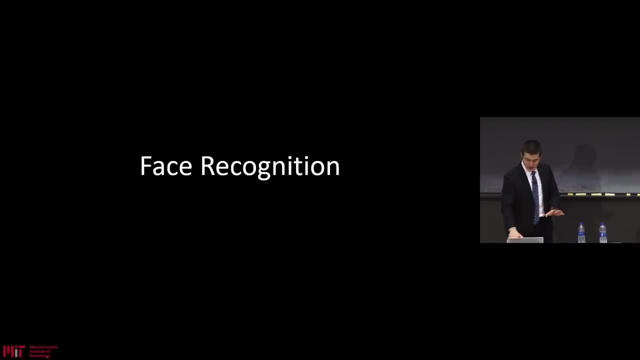 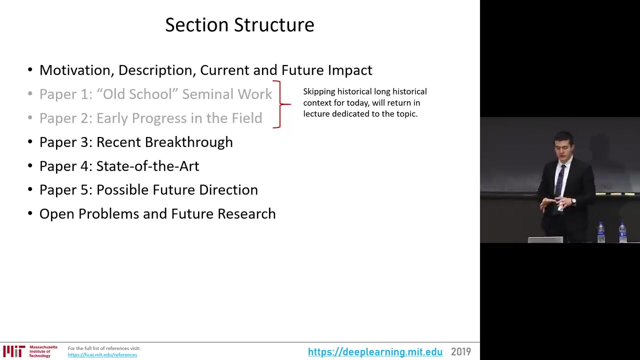 That's where deep learning really shines. I'd like to cover the state of the art in those various perception tasks. So first, face recognition. Now there's a full slide presentation with this, and I'm skipping around. The full slide presentation has the following structure: 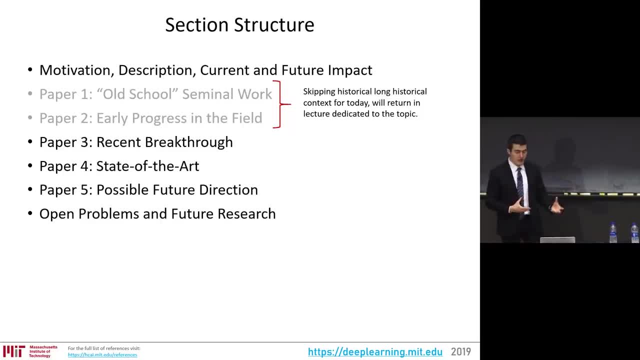 for each of these topics It has the motivation, description, the excitement, the worry, the future impact is the first part, And then there's five papers: One defining the quote unquote- old school seminal work that opened the field, Then the early progress in the field. 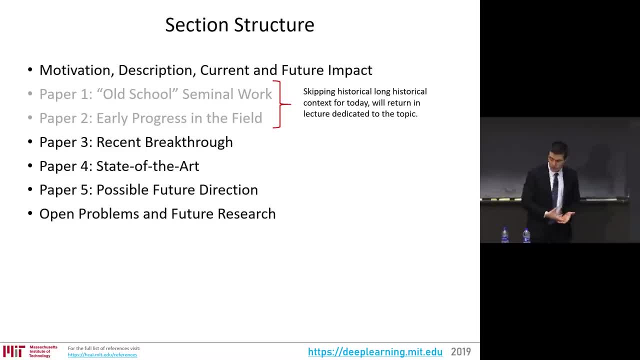 And the paper three is the recent breakthrough often associated with deep learning. Paper four is the current state of the art And paper five is the thing that defines the future direction, The possible set of things that define the future direction, And then the open problems in the field. 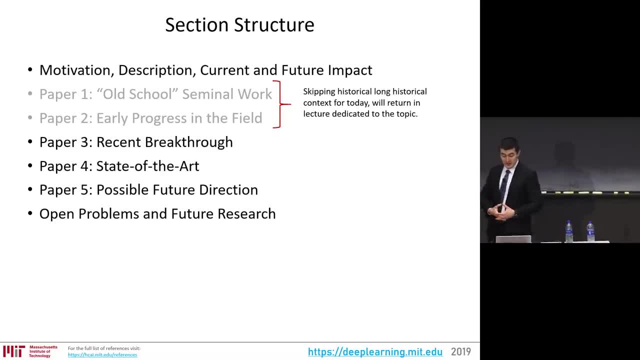 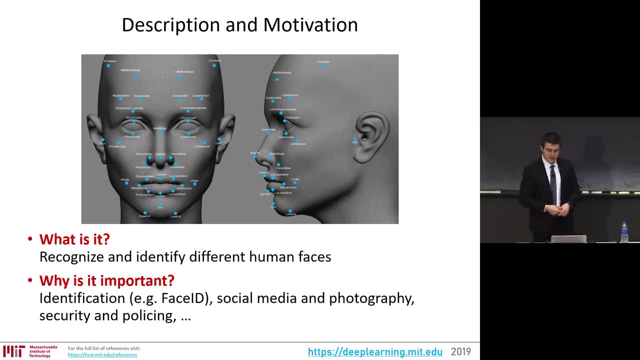 And then the open problems in the field And where the future research is very much needed. That's kind of the structure of every topic I'll cover here as quickly as possible. Face recognition. So what is it? It's the first thing you know. 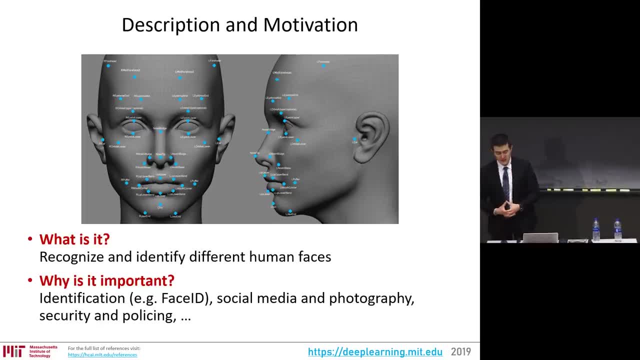 the face contains so much rich information about the state of the human being. So understanding the human being really starts at the face, And detecting the face is the first step, Detecting the body And then that there's a head on top of that body. 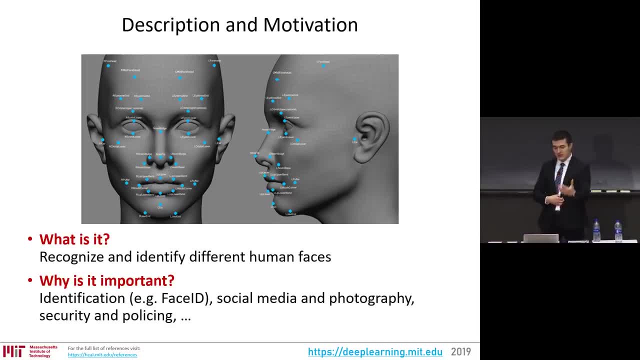 That's the first step, And then there is the task of face recognition Been an exceptionally active area of research because it has a lot of applications And through that research we're able to now study a lot of aspects: how we perform perception on the face. 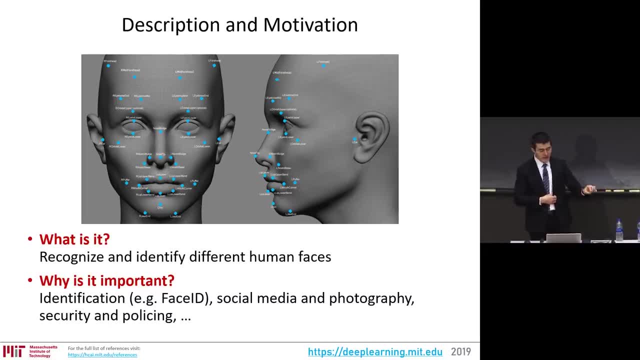 So recognition, purely stated, is the recognizing the identity of a human face. Who is this Detecting? Detection is just detecting a face. Now, recognition means there's a database of identities. What is it? Seven billion of them on Earth. 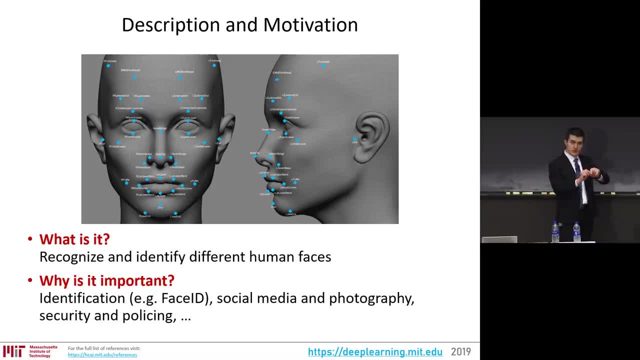 And you're trying to determine which of them it is, Which of the seven billion it is, Or whatever the database is. The face verification problem is something that your phone uses when you unlock it with your face. Is it saying: is it you or not? 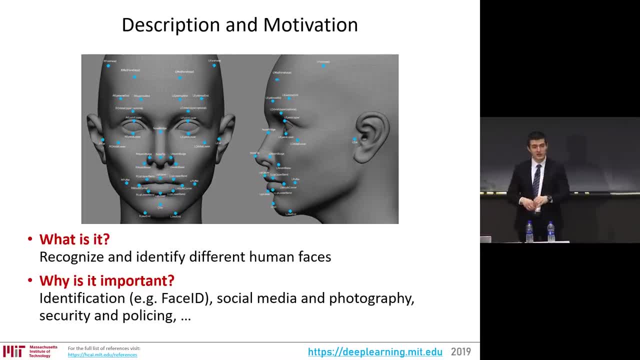 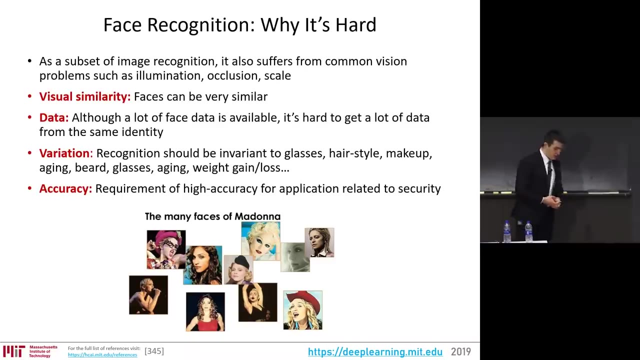 Is it Lex or somebody else? It's a database of two, One person versus everybody else. There's a lot of applications here, Obviously, from identification to all the security aspects of using the face as a sort of fingerprint of your identity in all the interactive elements of AI systems. 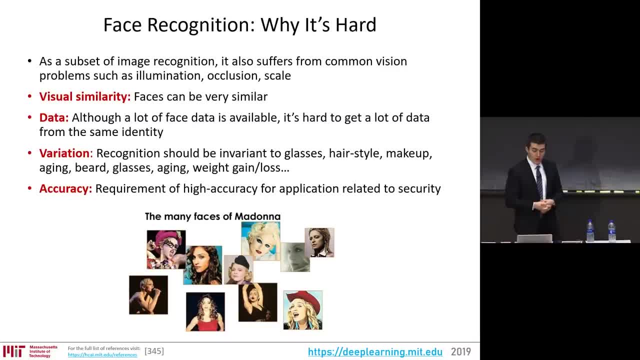 software-based systems in this world. Okay, So why is it hard? Why is it hard? So all the usual computer vision problems come in: Lighting variation, pose variation. That's just computer vision is really hard. It's just you get these raw numbers. 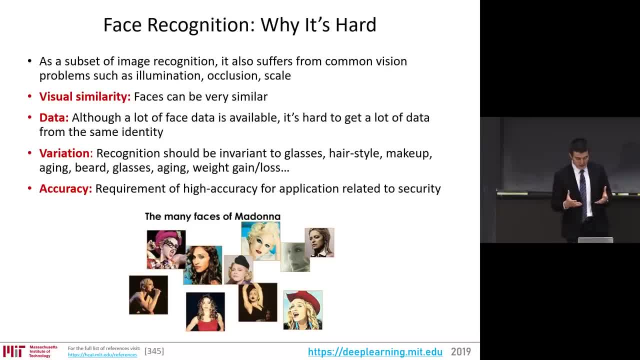 and you have to infer so many things that are that us humans take for granted, So the basic computer vision stuff. But there's stuff on top of that, So faces we're trying to. it's like cats versus dogs. 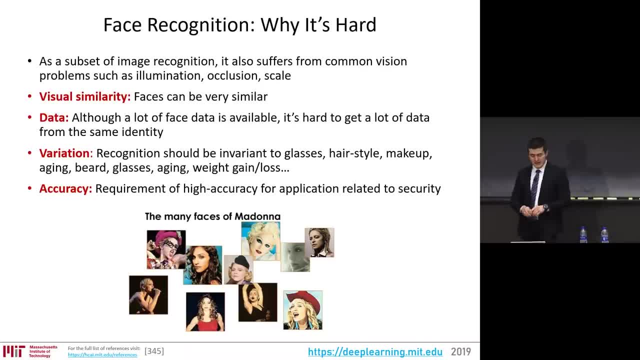 There's thousands of breeds of dog and thousands of breeds of cats. In that same way, there's faces can look very similar to each other. So these two classes that you're trying to separate can be very, very, very close together and intermingle. 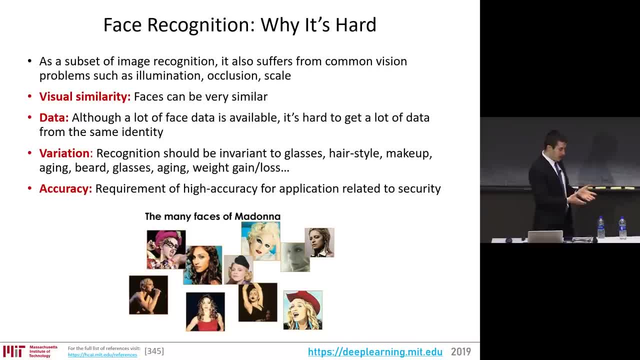 Now there's a lot of face data available Now because of the application, because of the financial benefits of such data sets, But for any one individual, unless you're Brad Pitt or Angelina Jolie or celebrity, there's not many samples of the data available. 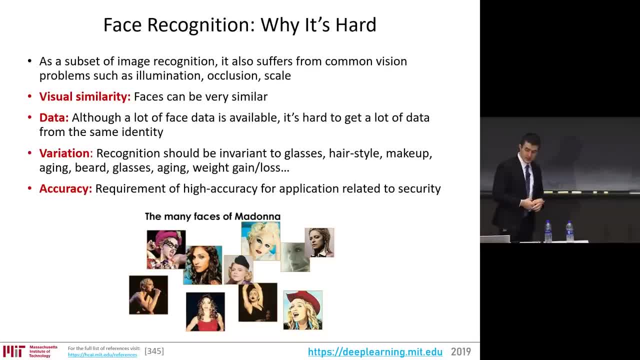 So the individuals based on which the classification's to be made. there's often not very much data. Then there is the a lot of variation. So you have to, in making the face recognition task, you have to be invariant to all the hairstyles. 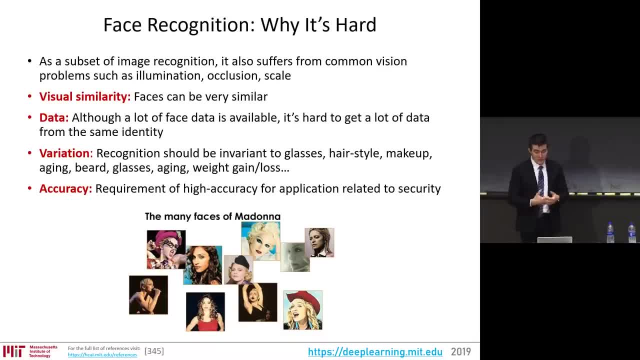 all the that you change yourself over time: the weight gain, the weight loss, the beard you decided to grow, the glasses you wear sometimes and not others, the different styles of glasses, and so on. Makeup or no makeups, all of these things, it's still you. 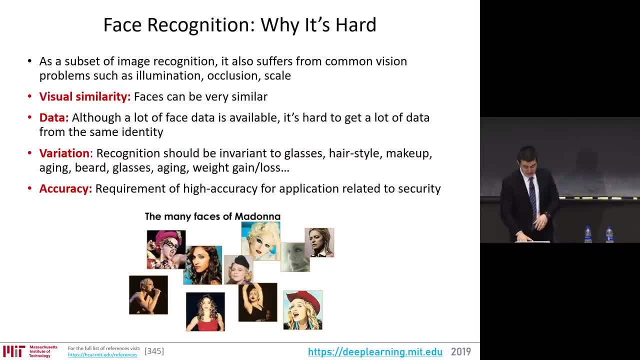 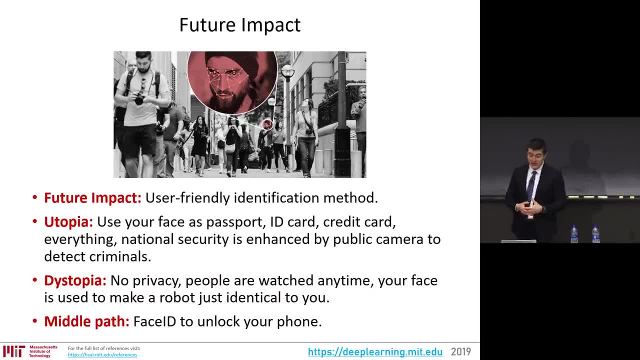 It's still the same identity. You have to be able to classify that And the kind of accuracy- especially for security applications- extremely high that's required. The reason it's an exciting area is there's a lot of possibility, but and there's also a lot of concern, right. 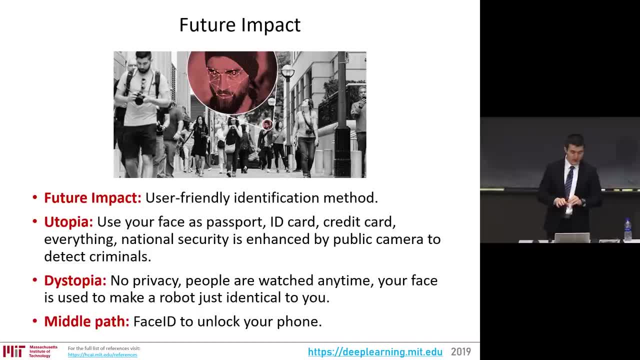 So the future impact, utopia, dystopia and the more reasonable middle path here is face- provides a very user-friendly approach of way of letting your devices recognize you and say hello. Your voice is certainly one, but one of the most powerful ones. 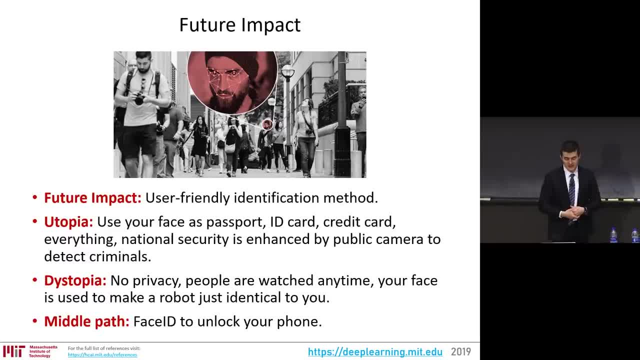 to really classify at a distance is face. So what does that mean? The utopian view, the possibility of the future, the best possible, brightest possible future is you can use your face to as a passport. you know you replace the license. 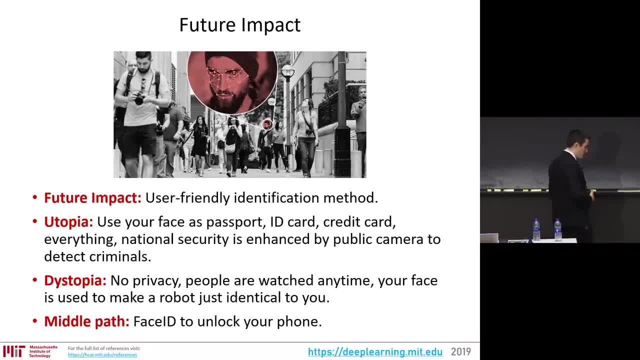 the place. all the security. you know all the security, all the security measures we put from the passwords on our devices to the credit card and so on. all of that you know. Apple pays, it'll be face pay. You show up, it'll automatically connect. 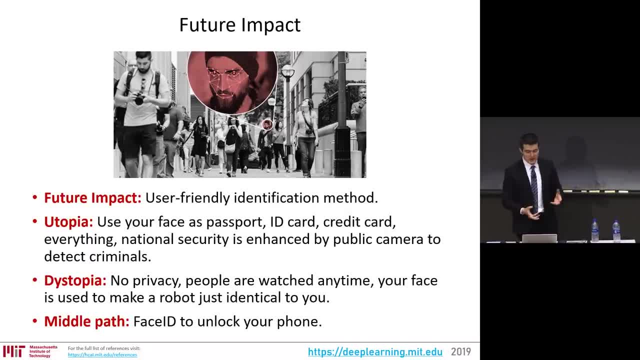 to all your devices, all your banking information and so on. Obviously, the flip side of that- just rephrasing that sentence- is also can be dystopian, because you know complete violations of privacy being washed at any time being able to enter your Facebook. 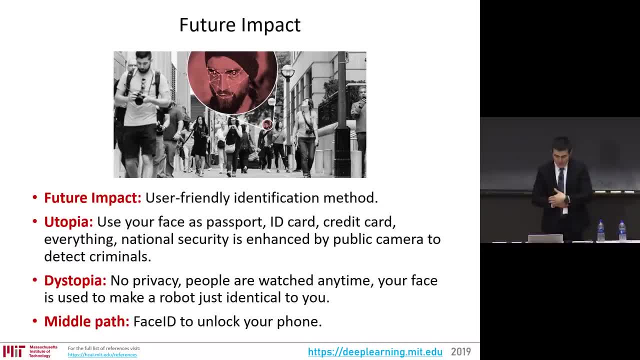 and social media and all your devices being able to identify you, making it impossible for you to sort of hide from society. The fundamental aspects of privacy, maintaining privacy that many of us value greatly. The middle path is really just a useful way. 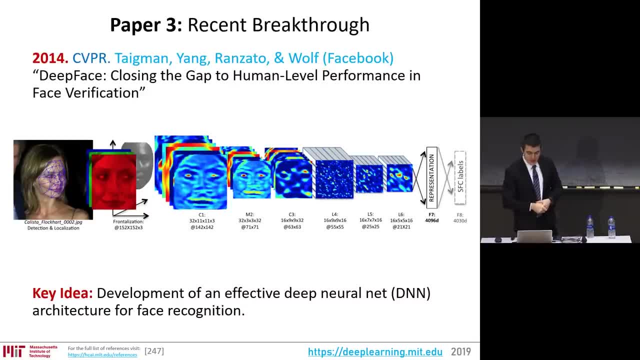 to unlock your phone, The recent breakthroughs here. it started with the with deep face. The essential idea there is applying deep neural networks to the task of face recognition. I mean with a lot of the breakthroughs here on the perception side. 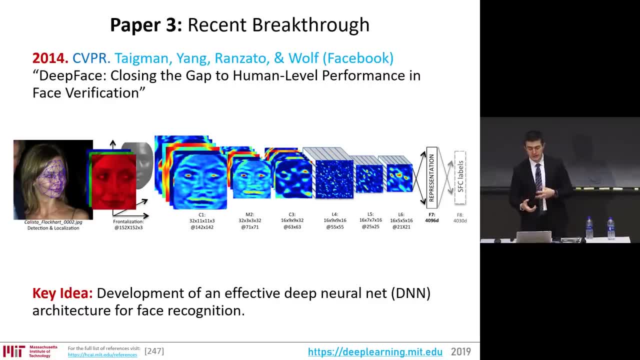 we're not covering the old school papers and so on and the historical context here. biggest breakthroughs came in with deep learning 2006,, seven, eight, last 10 years. So that's the same is true with face recognition. 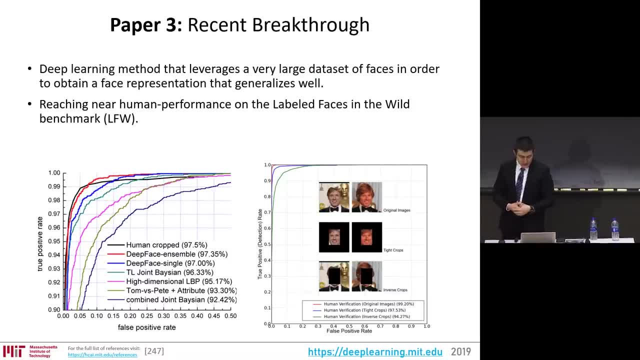 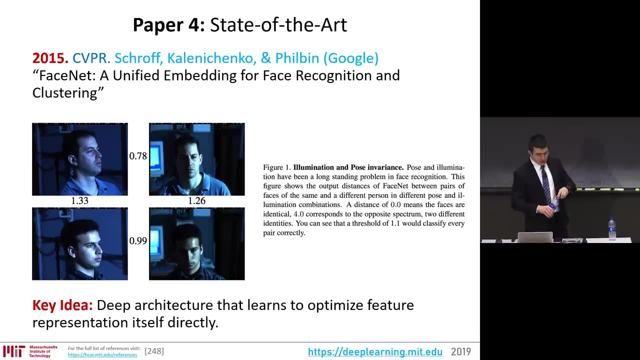 Deep face was the big first application that achieved near human performance on the one of the big benchmarks at the time on the labeled faces in the wild. So, using a very large data set being able to form a good representation, The state of the art, or at least close. 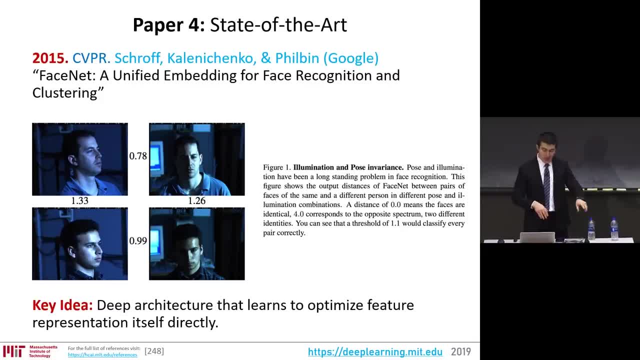 to the state of the art is face net. The key idea there is using those same deep architectures to now optimize for the representation itself directly. The notebook we're putting out, or we shared with some of you for the assignment, describes face recognition, the challenge there. 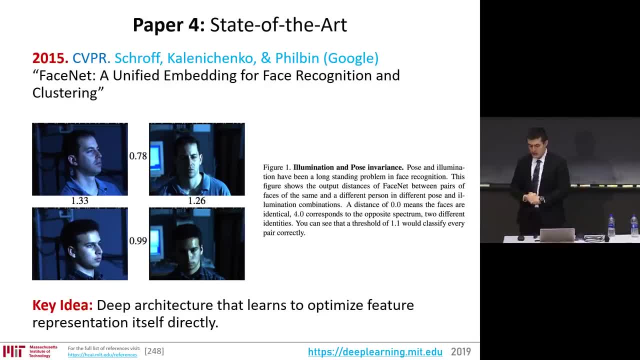 that it's not like the traditional classification problem. You have to, you have to form an embedding of the face into a small vector, compressed vector, such that in that, embedding faces that are similar to each other, so identities that are close together. 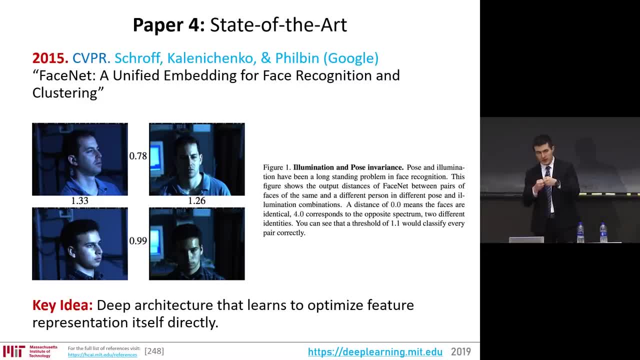 are close in the Euclidean sense, in that embedding and people that are very different are far away, And so you use that embedding to then do the classification. That's really the only way to deal with data sets for which you have so little information. 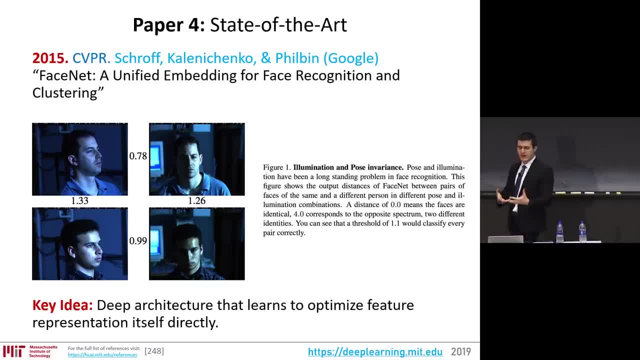 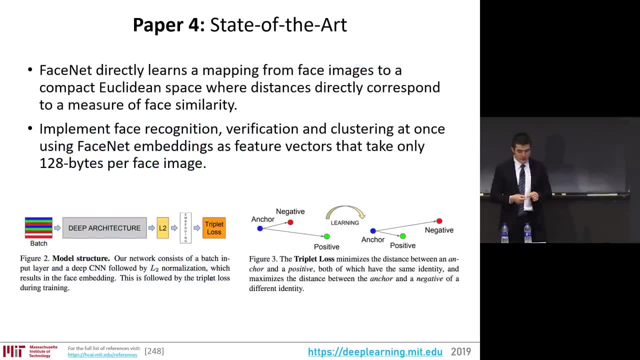 than any one individual person, And so face net optimize that embedding in a way that directly optimizes for the Euclidean distance between non-matching identities. So there's still a lot of excitement about face recognition and there's a lot of competition. 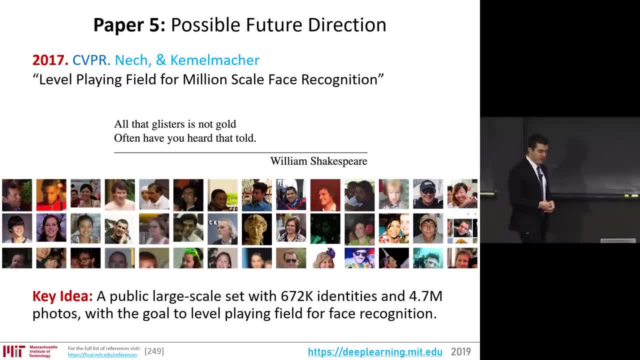 There's a lot of benchmark competitions and a lot of people working in this, and really bigger, better networks and more data is really one of the ways to crack this problem. So public, large data set with 672,000 identities, 4.7 million photos- that's in 2017,. 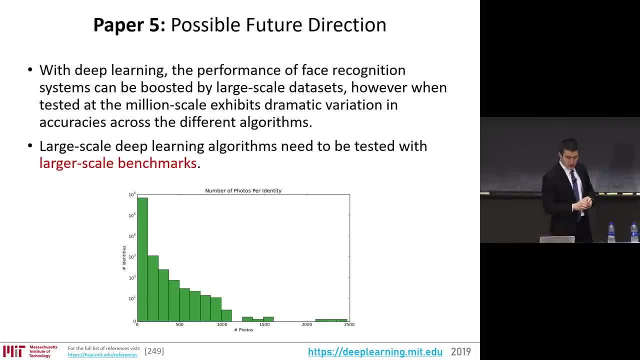 and that just keeps scaling up and up, and up and up. Now we have to also be honest here on the possible future directions of work, in that, you know, even though the benchmarks are growing, that's still a tiny subset of the people in the world. 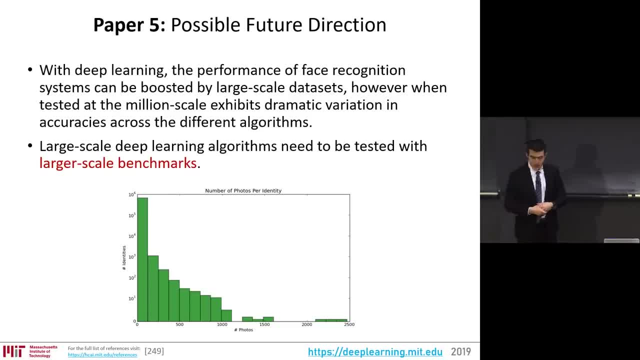 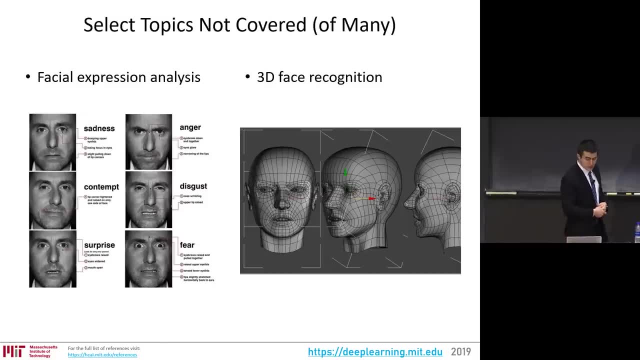 We're still not quite there to be able to have the general face recognition applicable to the entirety of the population or a large swath of the population of the world. So in this topic here, brief coverage. we're not covering all the aspects of the face. 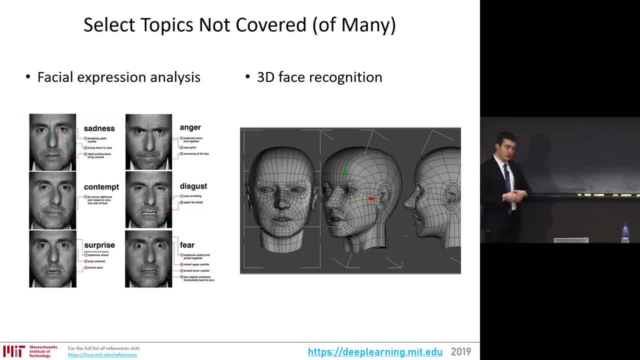 especially temporal, that are useful in face recognition or useful saying a lot of things about the face, which is the FACS facts, the different kinds of facial expressions that can then be used to infer emotion and so on. you know, raised eyebrows and all those kinds of things. 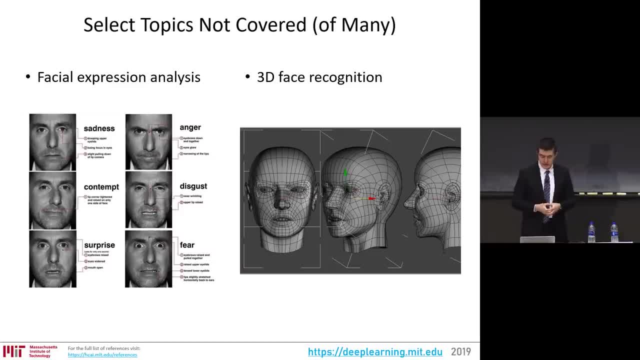 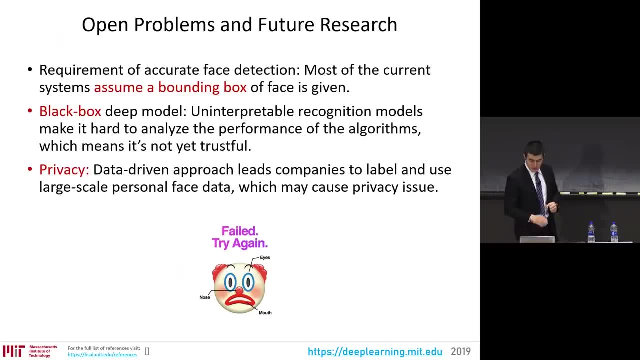 that could provide rich information for recognizing and interpreting the face and the different other modalities, including 3D face recognition we're not covering. There's a lot of exciting areas there where we're just looking at the pure formulation of the face recognition problem of looking at a. 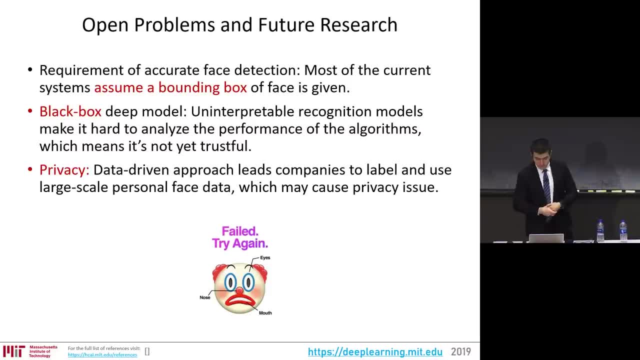 2D single image. The open problems here is: first, not often stated and misinterpreted by people, is that most of these methods of face recognition start with assuming that you have a bounding box around the face. Now, oftentimes recognition can happen. 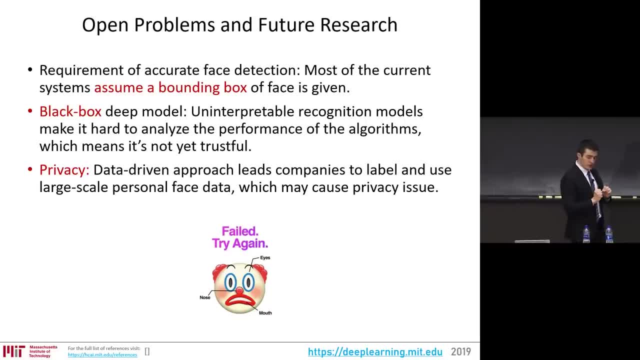 so they're assuming a frontal or near-frontal view of the face. but you can do recognition in all kinds of poses and it's very interesting to think you know that recognition- the way we recognize our friends and colleagues, parents and children- is often using a lot. 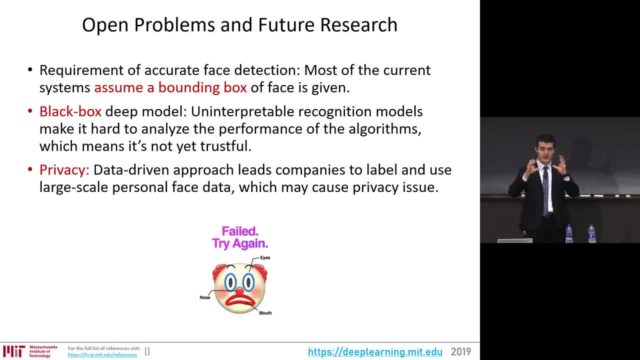 of cue context information that's beyond just the pure frontal view of the face. It can do pretty well on profile views. it can from body language and so on. So all those things that's open in the field, how we incorporate that into face recognition. 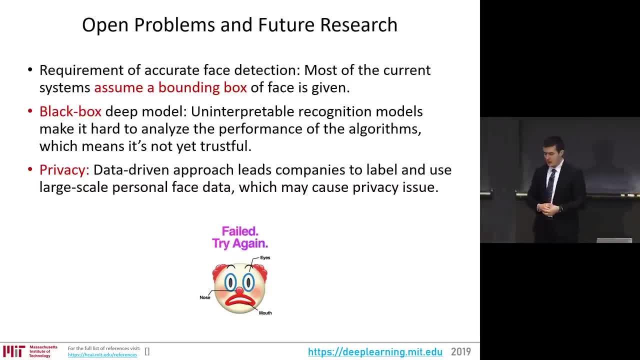 Then the black box side is problematic for both bias, and just being able to understand why incorrect decisions are made is the making those face recognition systems more interpretable. And then, finally, privacy: The ability to collect the kind of data where the face recognition would be performing. 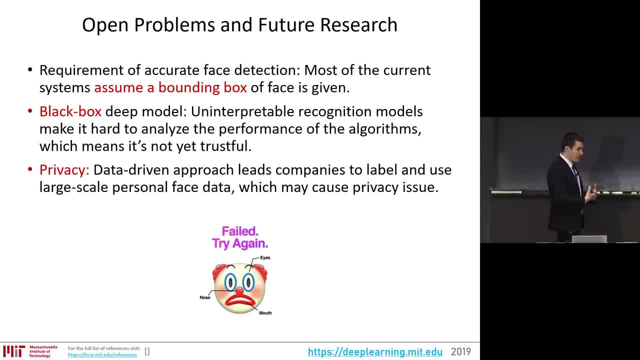 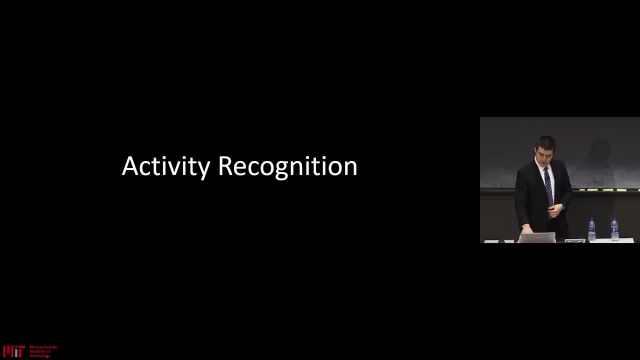 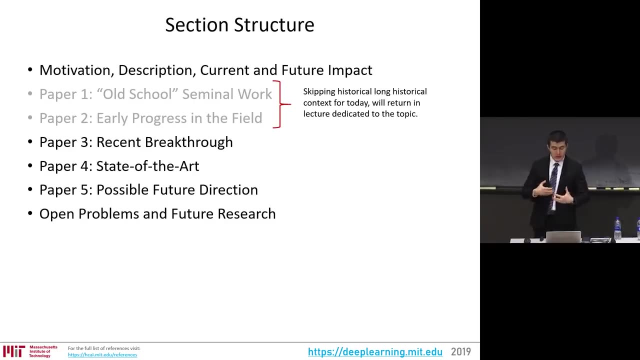 extremely well and yet not violating the fundamental aspects of privacy, And that's the kind of privacy that we value. Activity recognition: taking the next step forward here into the richer temporal context of what people do- Again the same structure from recent breakthroughs. 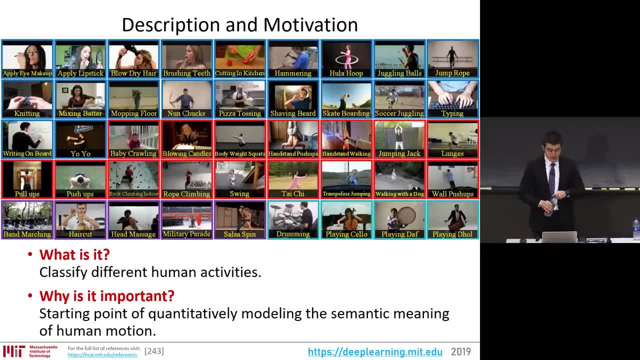 to the future direction of work. What is it? It's classifying human activity from images or from video. And why is it important? Because it provides, depending on the level of abstraction for the activity, it provides context for understanding the human. 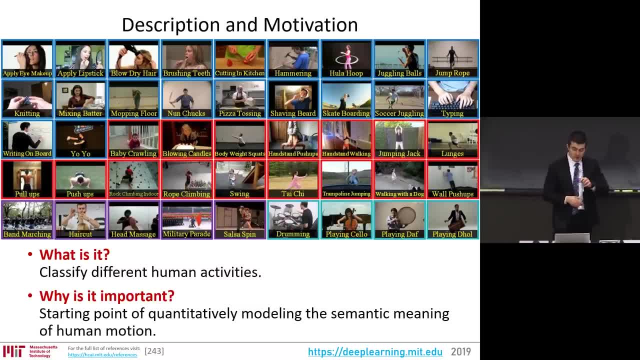 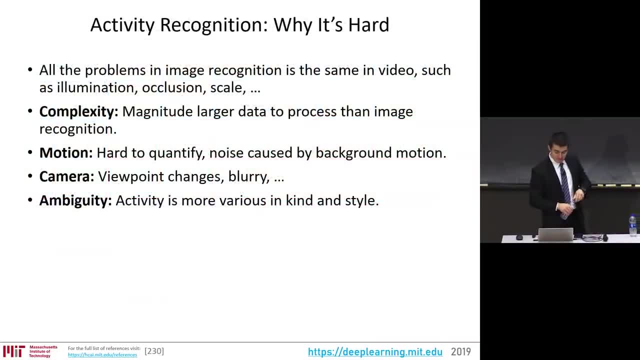 What are they doing? Are they playing baseball? are they singing? are they sleeping? are they putting on makeup, knitting so on, mixing butter. Why is it hard? Again, all the usual problems in image recognition. The kind of data we're dealing with is just much larger. 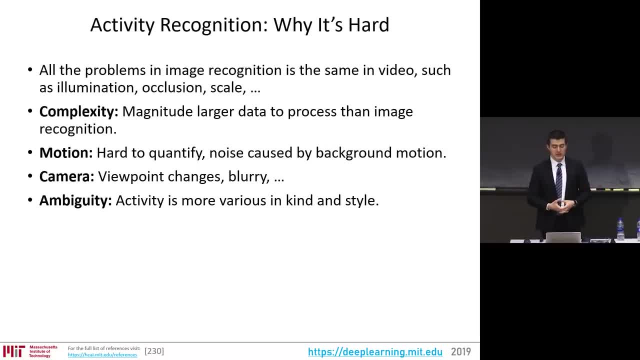 The kind of video, the richness of possibilities, the kind of data we're dealing with is just much larger. The possibilities that define what activity is is much larger, so the complexity is much larger. It's often difficult to quantify motion, because the fundamental aspect of activity 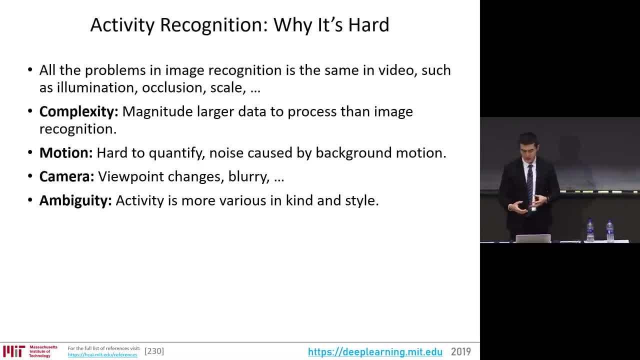 is the change in the world, is the motion of things, And then it's difficult to determine how the dynamics of the physics of the world, especially from a 2D view of what's background information, what's noise and what's essential to the to, I don't know. 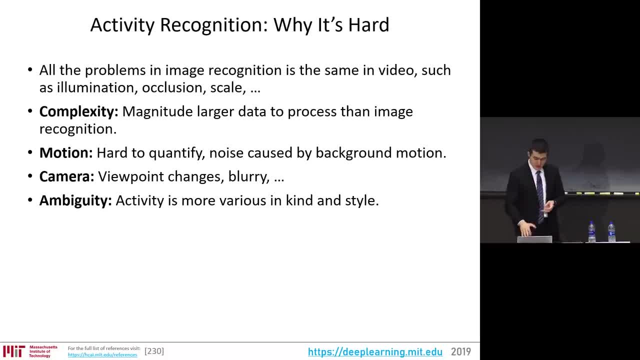 understanding the activity And the subjective ambiguous elements of activity. When does when does a particular activity begin? when does it end? what's all the gray areas when you're partially engaging in that activity, and so on, When you start to annotate these things? 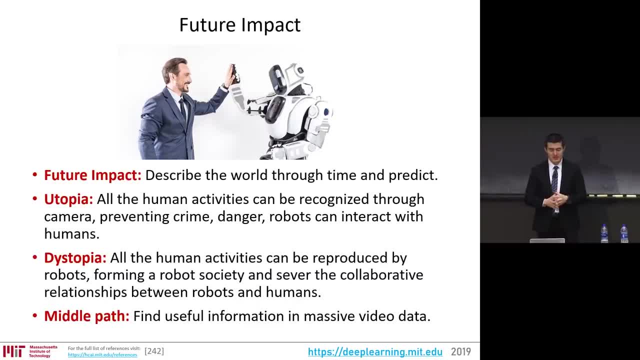 when you start to try to do the detection, it becomes clear that sometimes the activity is partially undertaken And the beginning and the end is fuzzy. Future impact, utopia, dystopia, middle path. So the impact here comes from the being able. 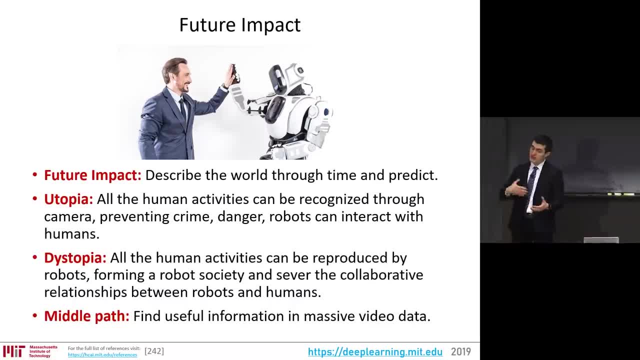 to understand the world in time and be able to predict The utopian possibilities is that the contextual perception that can occur from here can enrich the experience between the human and robot, The dystopian view, the flip side is being able to understand sort of human activities. 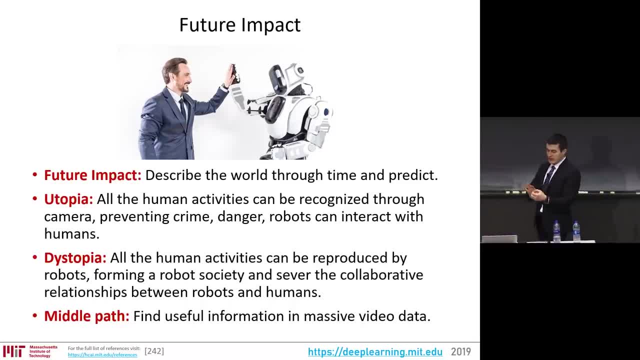 can let the robots sever the relationship So it can damage the human-robot interaction to where they just do their own thing. The middle path is just finding useful information, massive amounts of data, like YouTube. Now there's a YouTube video data set. 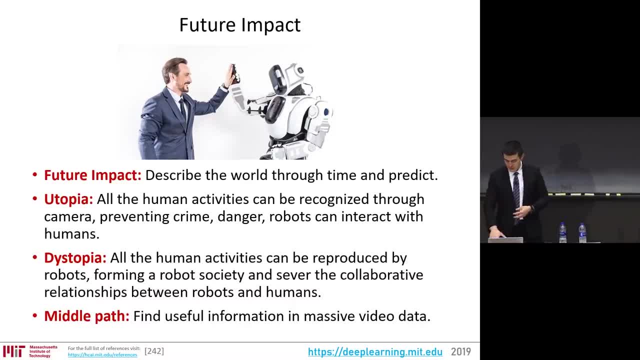 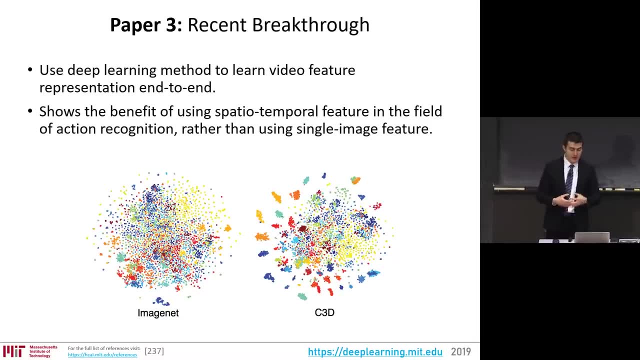 being able to identify what's going on in this video, being able to infer rich, useful semantic information, And so what do we do with video? How do we do perception in video? Now, the recent breakthrough came with deep learning and C3D, this 3D convolution, neural networks. 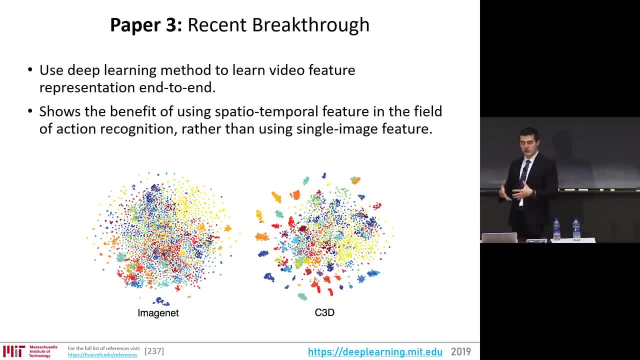 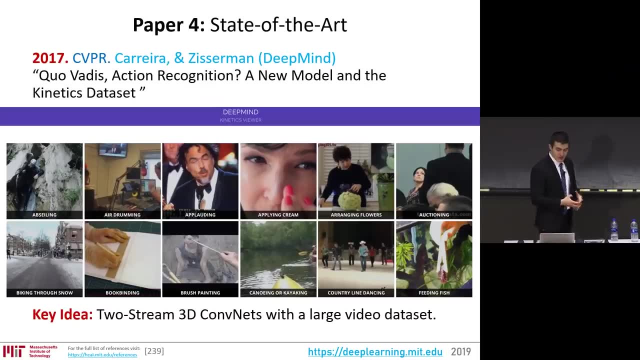 that take a sequence of images and are able to determine the action that's going on in an end-to-end way. what's going on in the video? That was the recent breakthrough, The state of the art coming from a slightly- well, from a different architecture that takes in two streams. 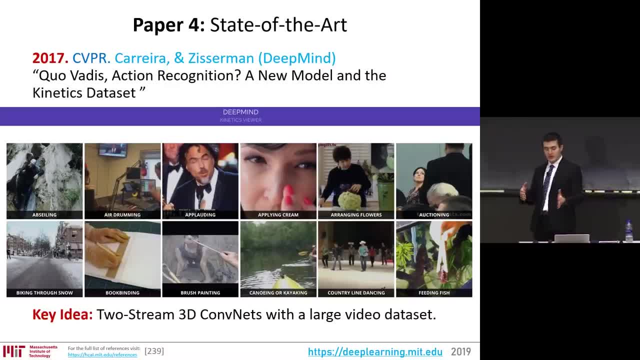 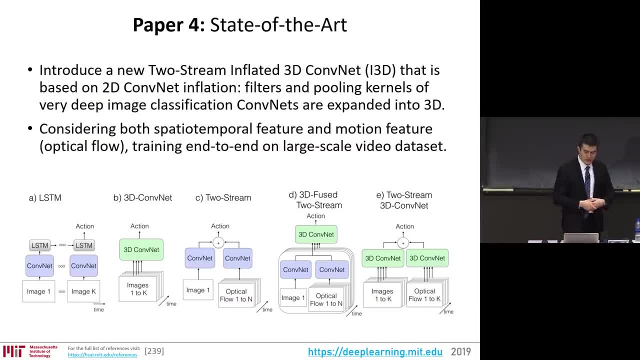 One is the image RGB data, the other is optical flow data that's really focusing on the motion in the image. Those are the two. That's opened the wave of two stream networks here. from that paper showing the different architectures, On the far right is the two stream architecture. 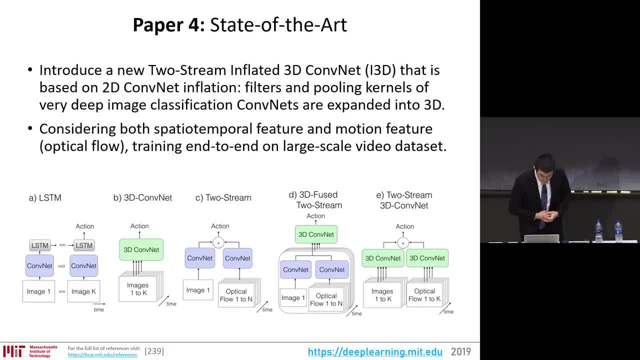 and the C3D shown under B here taking a sequence of images. But all these are just different architectures. And then, first one is LSTMs. There's different architectures of how do you represent, how do you allow a network, how do you allow a learning model. 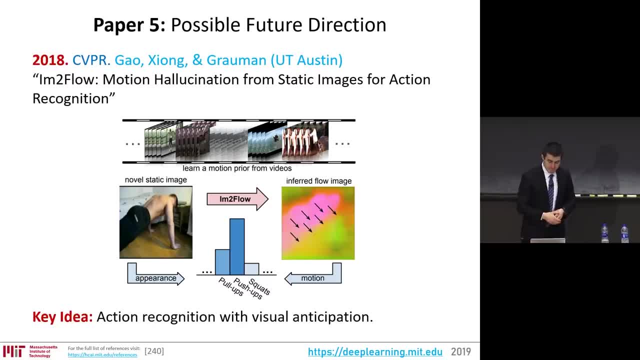 to be able to capture the dynamics in the data. The future possibilities has to do literally with the future: being able to take single images or sequences of images, and predicting the future. It's very interesting to think about in our ability to hallucinate the future. 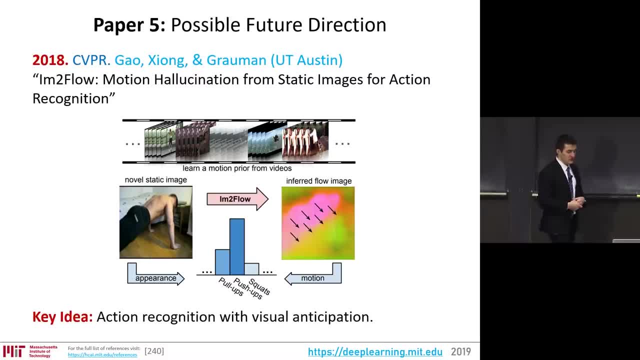 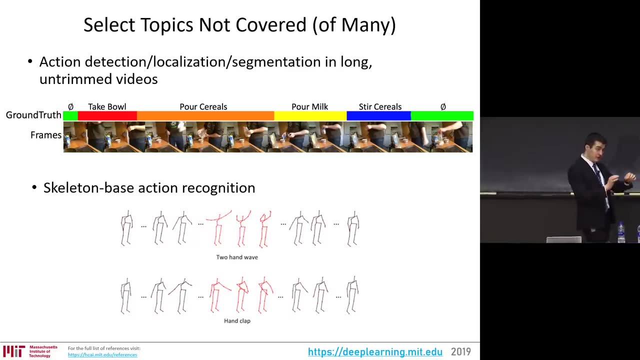 and generate the future from images. You start to think about what are the defining qualities of activities and in this way, augment data and be able to train much more accurate action recognition systems. Topics not covered is the localization of activity in video, So action recognition purely defined is. I give you a clip. 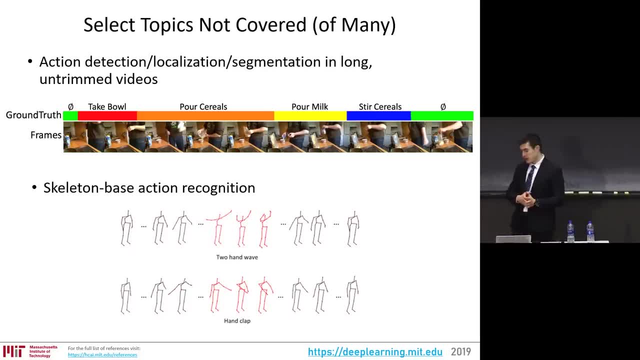 and you tell me what's going on in this clip. Now, if you take actually a full YouTube video, you want to be able to localize, find all the times when particular activities are going on. It could be multi-label, multiple activities going on at the same time. 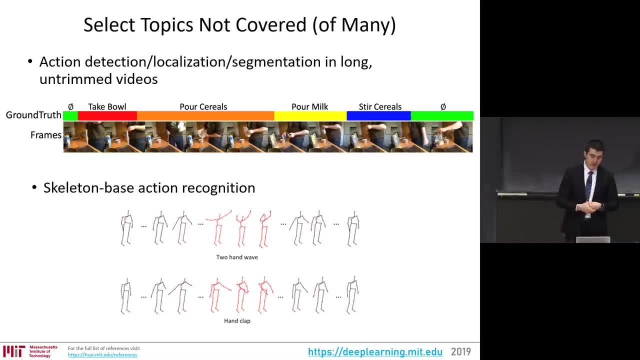 beginning and ending in asynchronously. And then there is, more richly, three dimensional or 2D classification of activity based on human movement. So looking at like from a connect from 3D sensors, looking at skeleton based action recognition from sensors that provide you more than just. 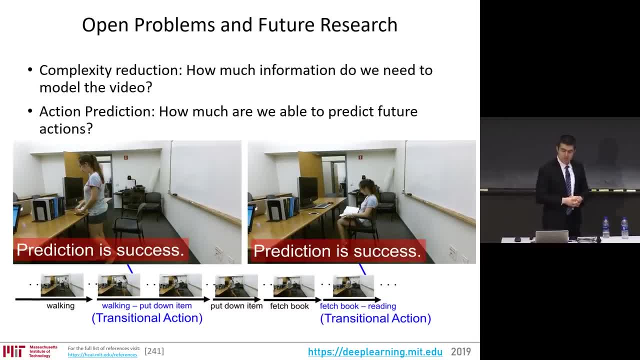 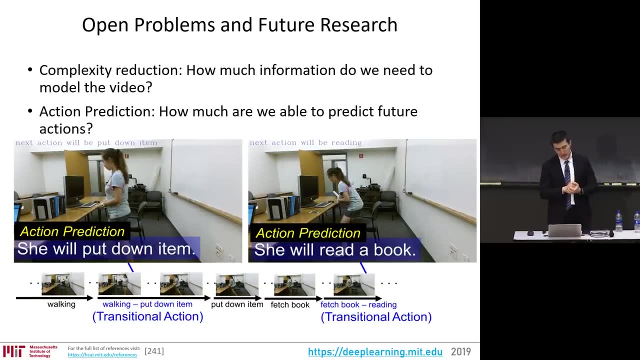 the 2D image data. The open problems is, that is, activity recognition is more than just the way we move our body or if it's baseball, like a ball in your hand and hitting- hitting it with a baseball bat. It also has to do with context. 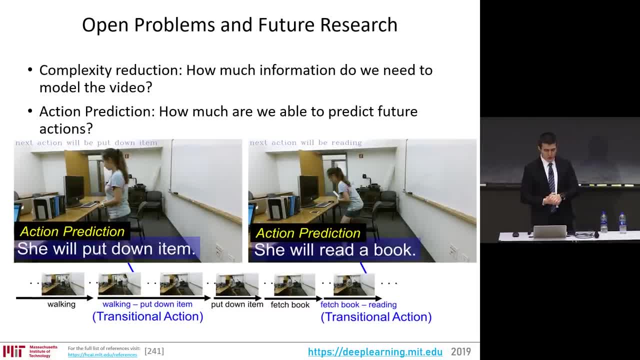 There's sitting down or working or looking at something and picking up an item, Those sometimes can change profoundly based on the other objects in the scene and the activity of other people in the scene, And so being able to work with that kind of context is a totally open problem. 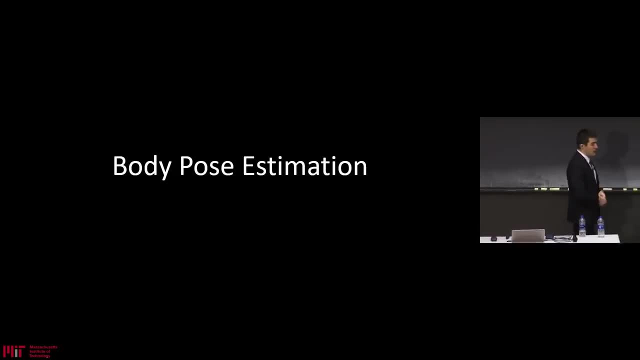 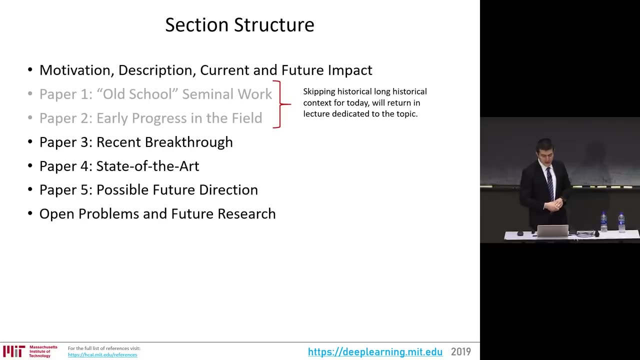 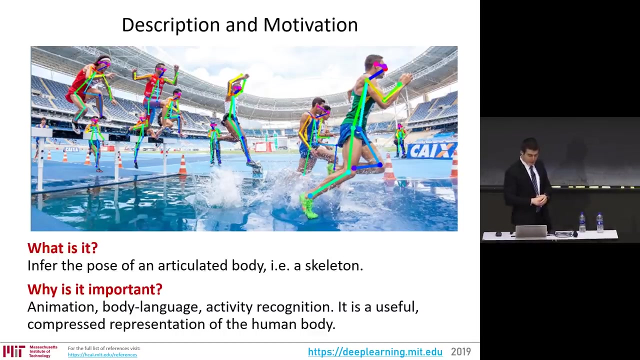 It's having to reduce a very complex real world context into something where you can clearly identify an activity. Body pose estimation is the task of localizing the joints that form the skeleton of the human body, So infer from visual information the positions of the different joints. 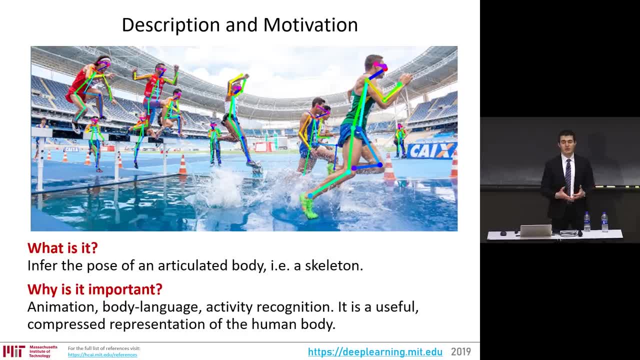 Along the line of complexity. it's important to be able to understand the body language, the rich information about the body of the human being. So that's from reading body language to animation, to aiding activity recognition, And it's just a useful representation of the human body. 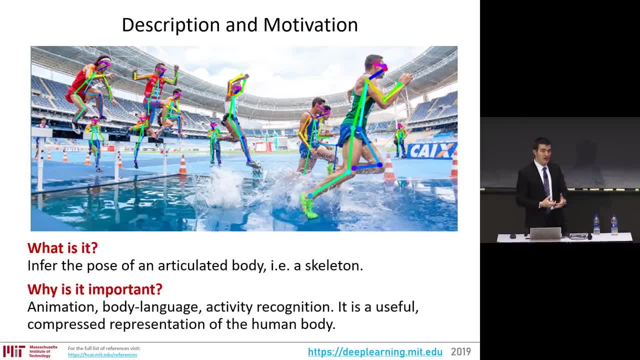 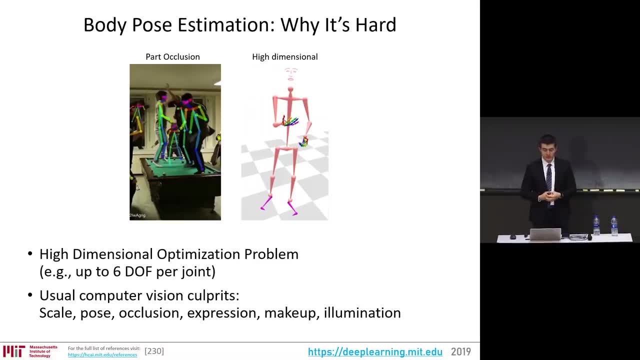 If you're analyzing pedestrians or in an interactive environments, human robot interaction, being able to understand what the heck it is the human is trying to do- A body pose is really, is really useful. It's hard because the body, when you look at it, 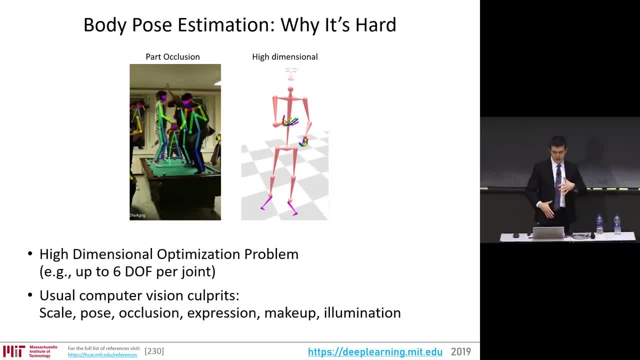 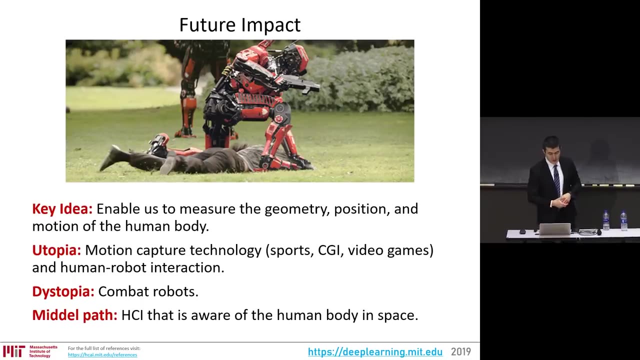 to 2D image projection of the body. there's a lot of. it's a highly dimensional optimization problem, figuring out how the raw pixels match to the actual three dimensional orientation of the human joints, And the usual computer vision challenges of pose, lighting and so on. 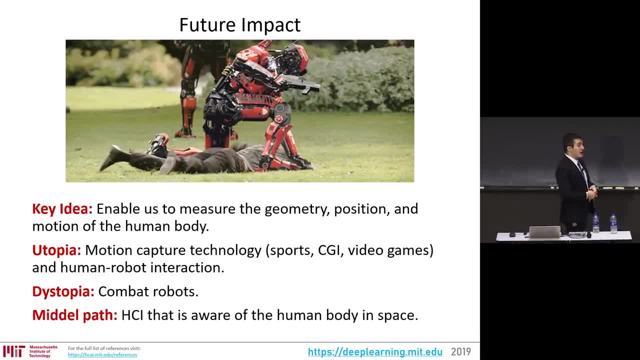 Future impact is. it's really exciting for interactive environments for a robot to be able to know the position of the human body when she's trying to interact, Whether it's a robot that's trying to get their favorite human a beer or whatever your favorite choice of drink. 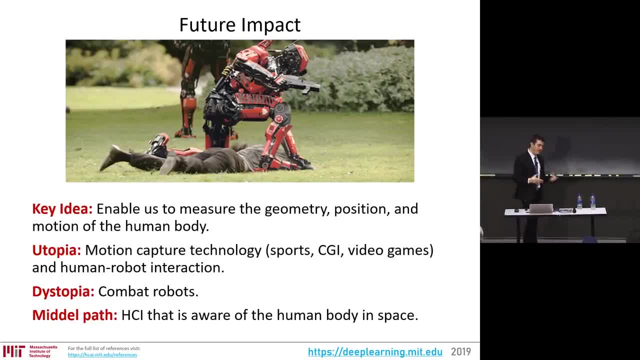 You have to be able to find where their hand is so you can do the trade off. Same thing in the car: You have to determine if the person's hands are on the steering wheel, if their head and orientation is such that they're able to physically take control of the vehicle. 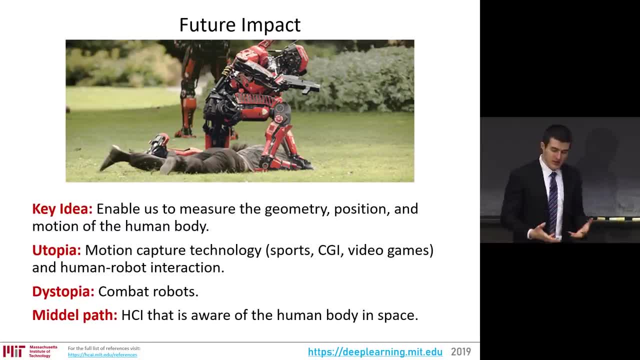 That's a really exciting set of possibilities there, And there's applications and sports and CGI and video games and all aspects when the robot and human have to work together. The dystopian view you can imagine is, of course, being able to localize all those joints. 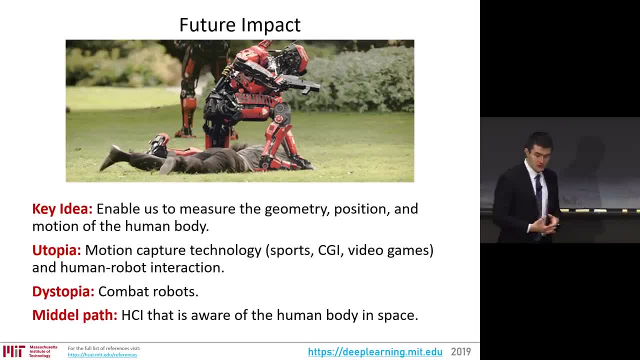 means robots that are able to more effectively hurt humans, And so that's always a huge concern and always a dark, dystopian view of the world with so much AI in it. Of course, the reality is it's just more rich fulfilling HCI. 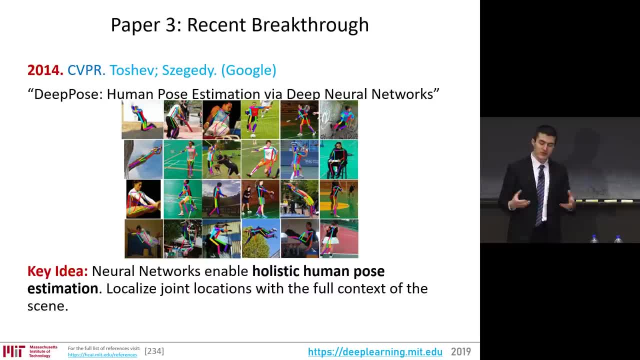 that takes advantage of not just the face stuff coming from the face, but also stuff about the body of the human that the robot is interacting with. So it started with deep learning being applied to the body. pose estimation problem 2014, with DeepPose. 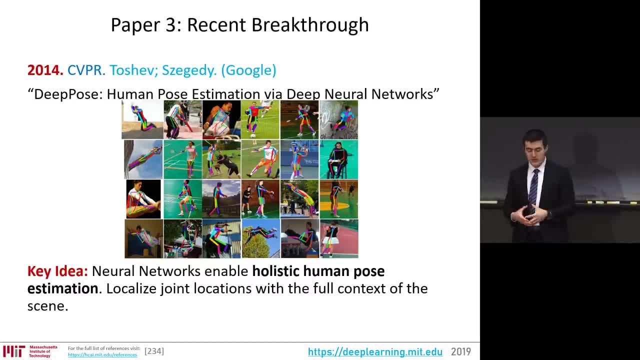 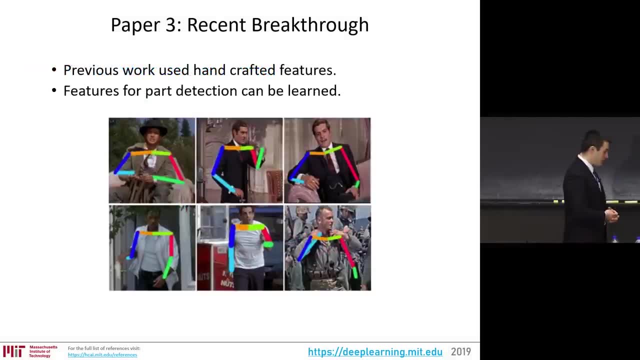 The key ideas there is looking at the holistic human pose estimation problem of detecting all the different joints of a single person in an image. Power of deep learning is that you no longer have to do handcrafted, expert engineered features. Power of deep learning is that you no longer have to do handcrafted, expert engineered features. 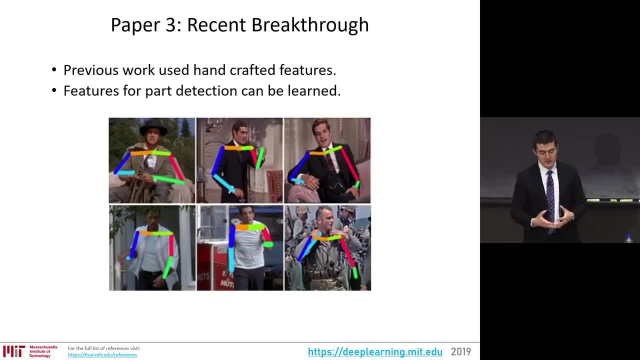 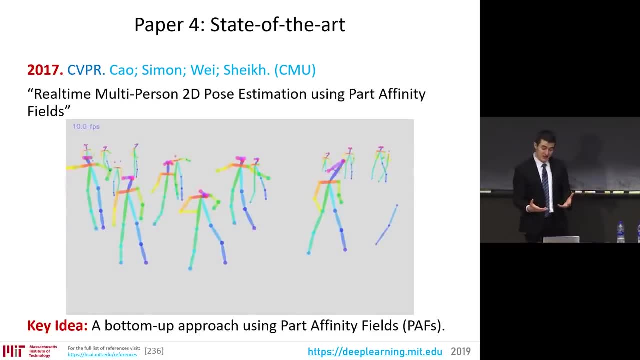 Power of deep learning is that you no longer have to do handcrafted, expert engineered features, That it automatically determines a set of features. All the parts are being detected for you. So this highly complex problem is all solved with data. This is the state of the art of 2017 and beyond. 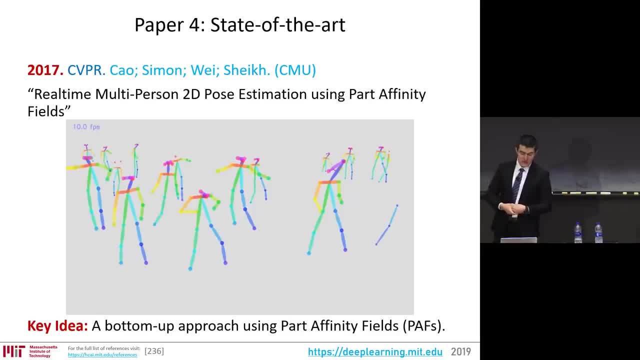 There's been a few papers from CMU along this line. It's doing real-time multi-person 2D pose estimation, but in a bottom-up way where you're detecting individual joints first. So all the knees in the picture, all the elbows. 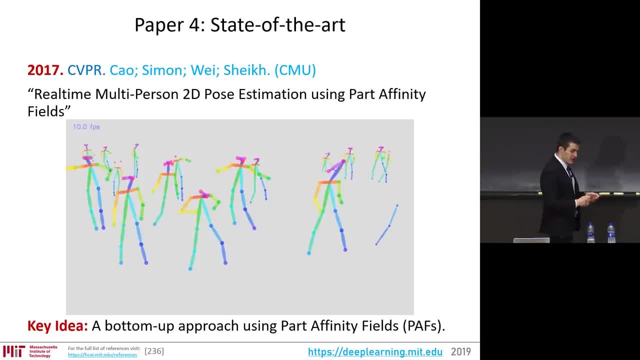 all the shoulders, all the wrists and so on, And then stitching them together using parts affinity fields, What is the most likely? So if you find 17 elbows in a picture, you then have to try to see which elbow belongs to which person. 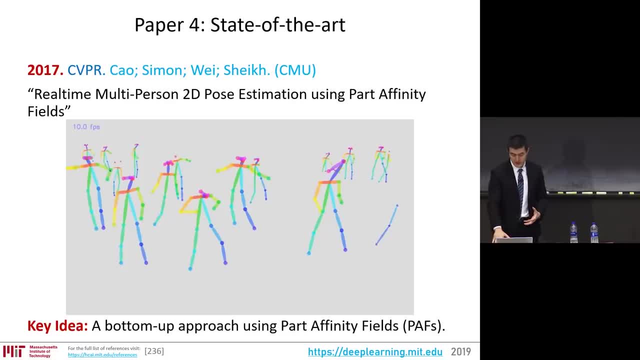 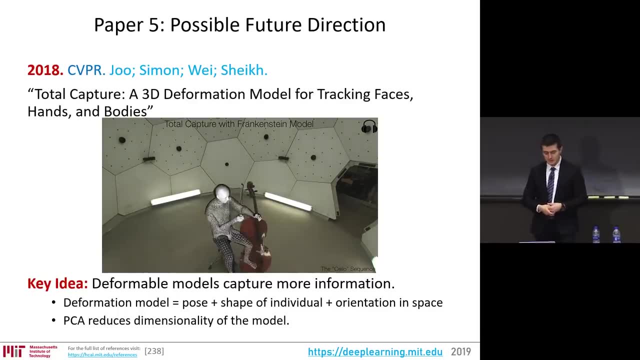 So that actually turns out to be extremely powerful way to detect, especially multi-pose, especially to deal with occlusions- way of detecting body pose. It's really interesting and also is able to because of that, because of the separation of the detections. 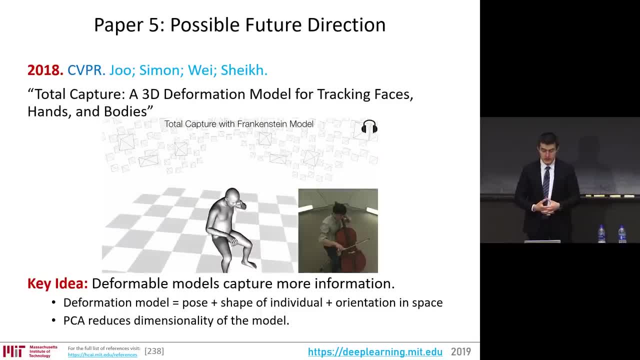 is able to run in real-time, which is also really exciting. Possible future direction is using much more information, using deformable models of the human body, So not just the skeleton- rich volumetric information to do the detection and then optimizing for what's the most likely orientation. 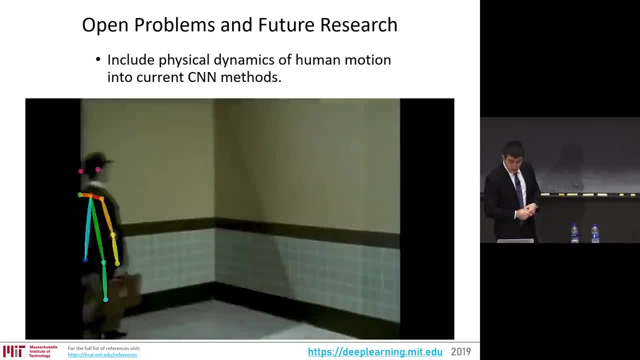 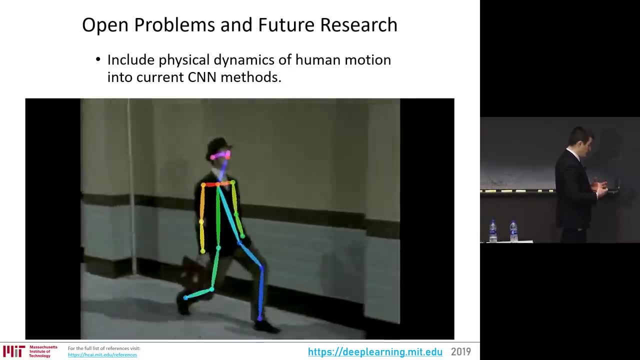 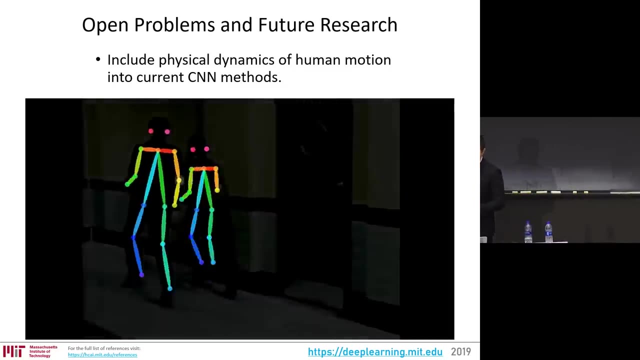 of the body. The open problems in the field is the fact that, you know, pose is not a thing that happens in a single image. pose that happens is part of human behavior and part of movement through time. So here Monty Python, minister of silly walks. 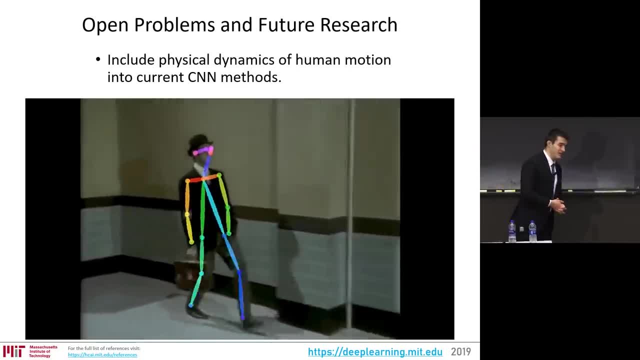 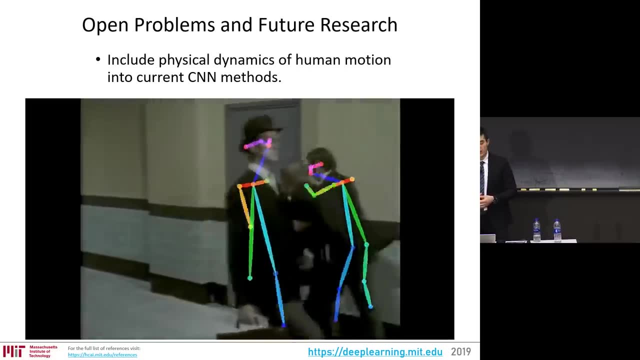 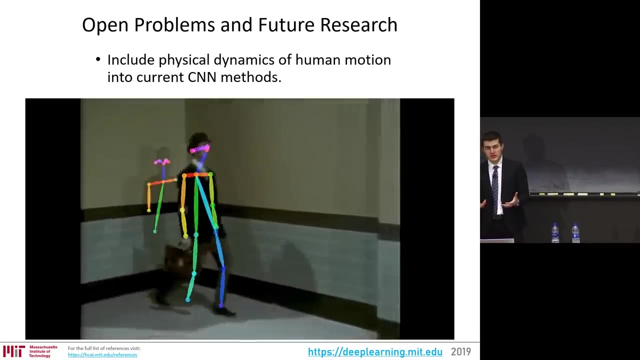 people walk in funny ways, but so we collect a lot of data on pedestrians. I can tell you that people walk in different ways and people position their body in different ways, And so the temporal, temporal aspects of human motion are, for the most part, not incorporated in the body. 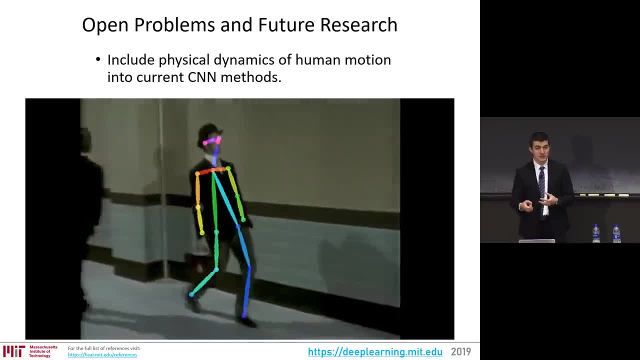 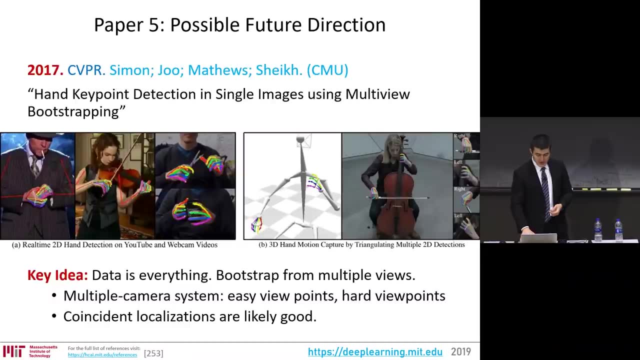 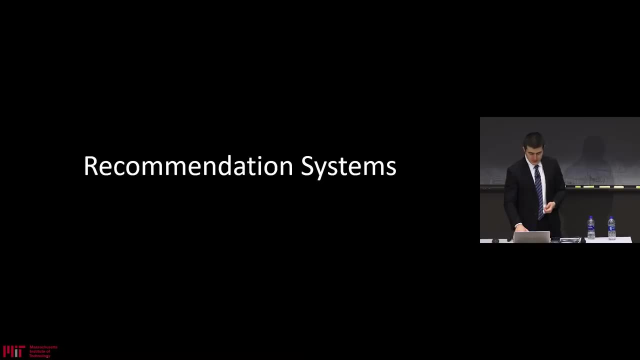 pose estimation problem- and they should be. There's a lot of exciting possibilities of capturing the temporal dynamics. There's a lot of awesome slides here that I'm just skipping through. speech recognition: That was 2018. that was really big for recommender systems for 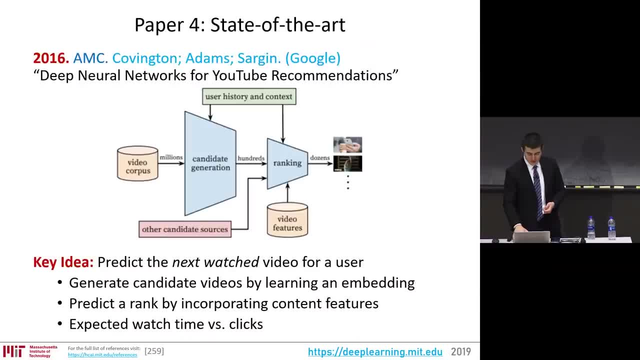 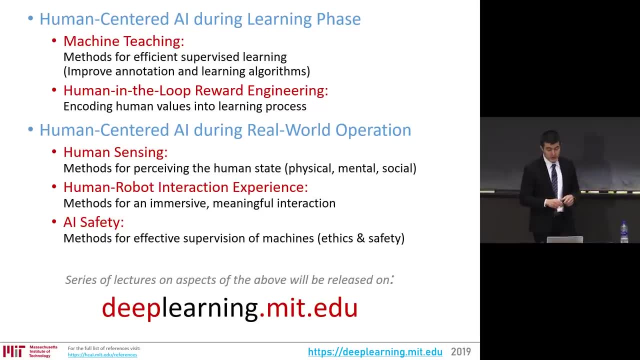 Netflix. Ok, Cupid AI. for president, Each one of the things that I mentioned briefly today will have a separate mini lecture. I taught an entire course on this at CHI last year, so deep learning for understanding the human. It's a topic I'm really excited about. 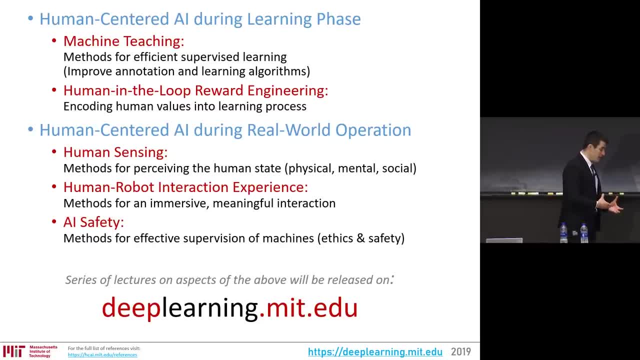 because it's really the first step for a machine to be able to interact in a rich way with a human being is to understand it, And it's also area where the most near-term impact can happen: a system to be able to effectively detect what a human being is up to what they're thinking about. 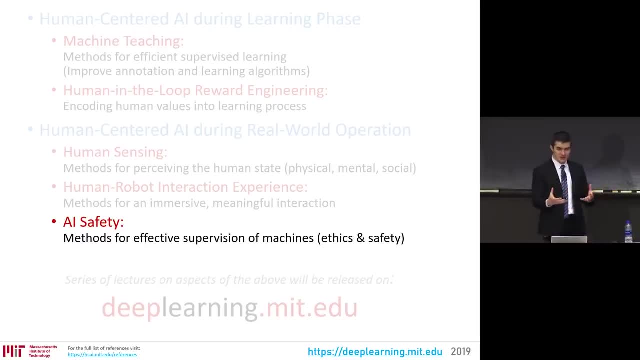 how to best serve them and enrich the experience of interacting with that human. Let me jump to AI safety and then the interactive experience with humans and robots, to just give examples of some work in that direction, some research in that direction I'm really excited about. 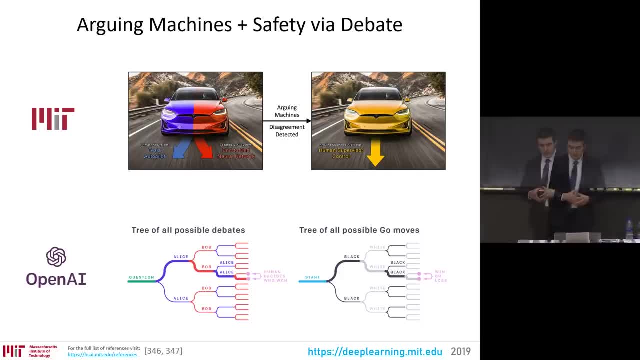 So AI safety at the very basic level. there's an AI system that's making decisions where we want human beings to supervise those decisions. We've done quite a bit of work here at MIT on that aspect of supervising machines, arguing machines. 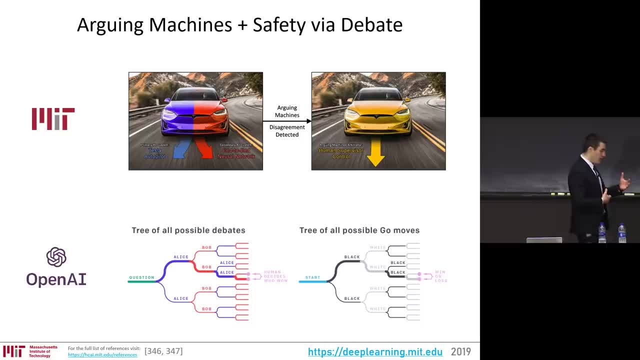 and OpenAI has done work with safety by having machines debate each other. So this kind of idea that you can achieve safety by not giving ultimate power to any one decision maker, And the disagreement that emerges from two AI systems or multiple AI systems having to make decisions. 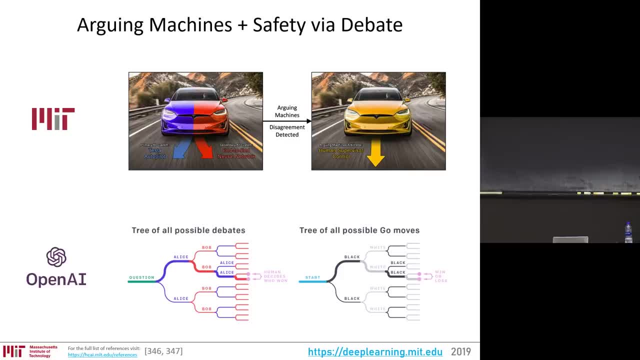 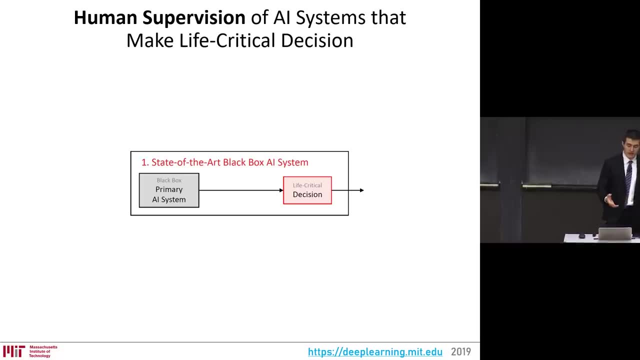 and agree with each other. it allows us to then produce a signal of uncertainty based on which the human supervision could be sought. Without that, when we have a state-of-the-art black box AI system that does something like drive a car, all we have is a system that just runs. 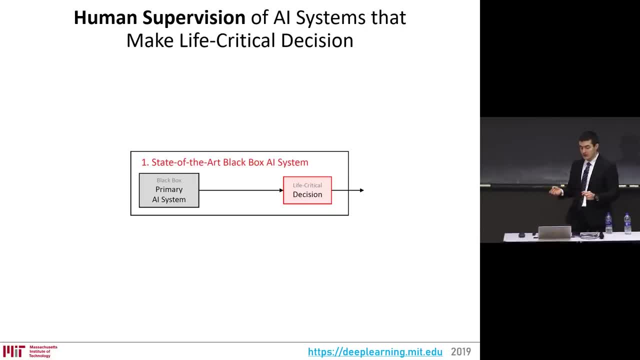 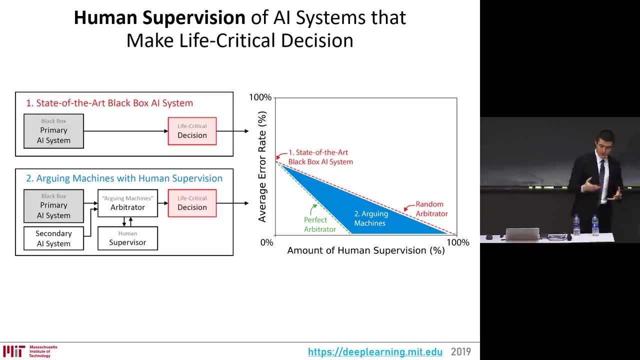 and we're supposed to have faith that it's always going to be right. We don't have any uncertainty signal coming from the system. So the idea of arguing machines that we've developed and been working on is to have multiple AI system, an ensemble of AI system, where the disagreement, when they're 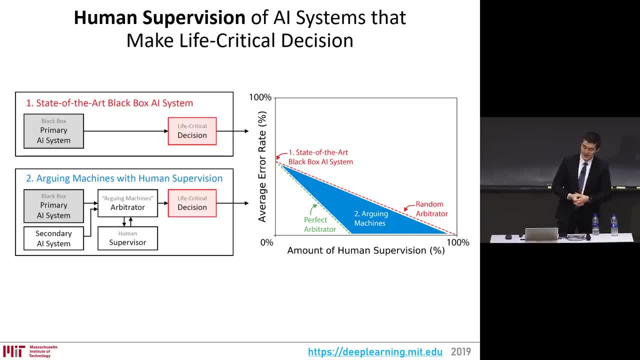 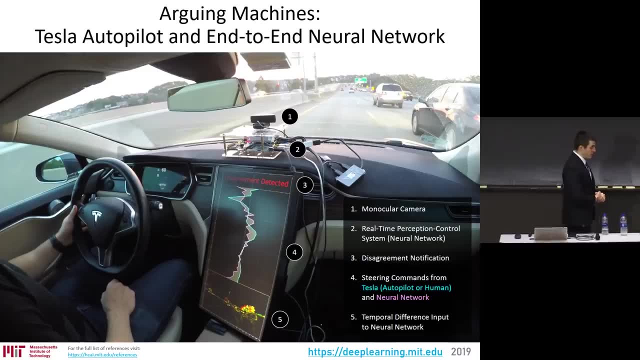 and there's a disagreement detected. the human supervision is sought And the idea there is that when you have a system like Tesla Autopilot- here we have instrumented a Tesla vehicle- when you have a system like Tesla Autopilot, it's telling you nothing. 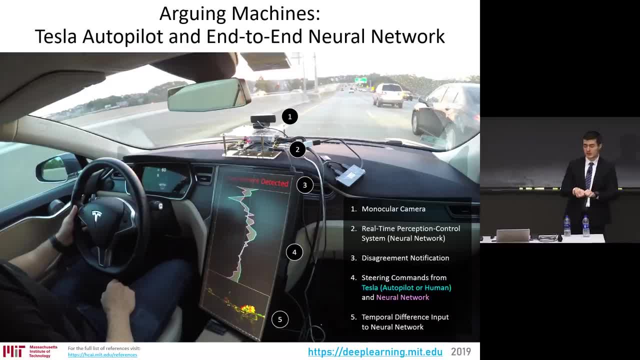 about how uncertain it is about the decision it's making. It just knows. once the system is on, it's now steering the car for you, And in very rare cases this is just disengage. But no matter what, it's not showing to you the degree. 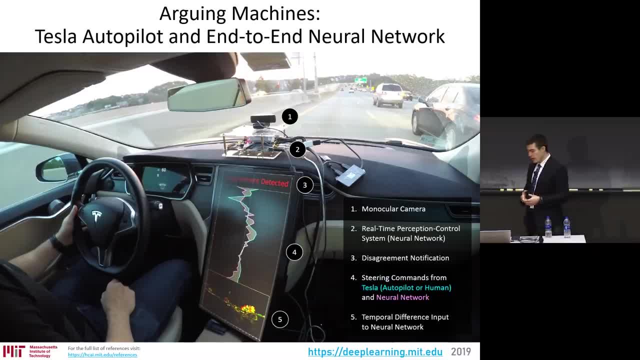 of uncertainty it has about the world around it, And so the way we create that signal of uncertainty is by adding another- in this case end-to-end- vision system that's looking at the external environment, making steering decisions, and, whenever there's a disagreement between the two, detected 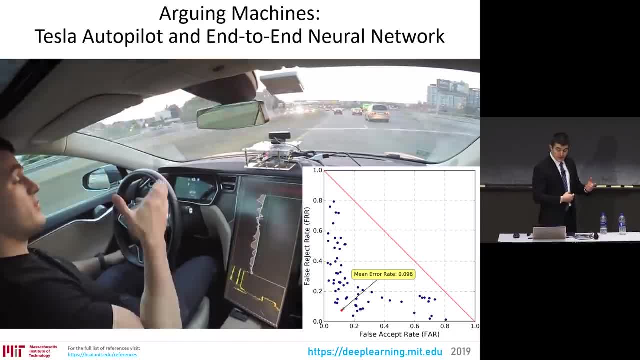 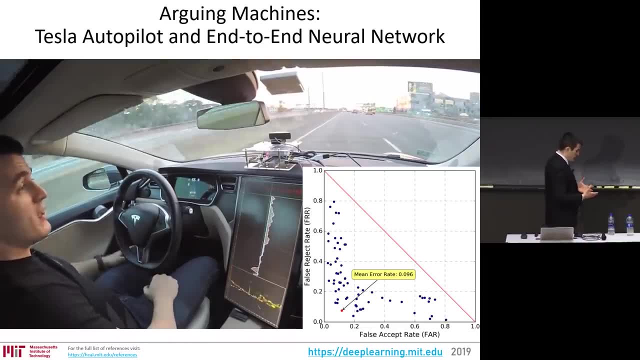 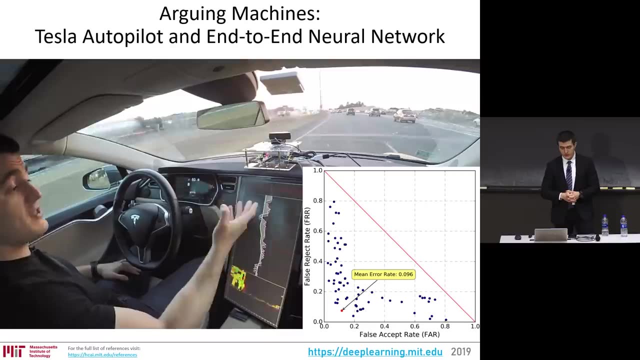 that's when human supervision is sought And we can predict in this way shown in the plot there is, we can predict with high accuracy the times when the driver chose to disengage the system because they were uncomfortable. So you're detecting, you're using this mechanism. 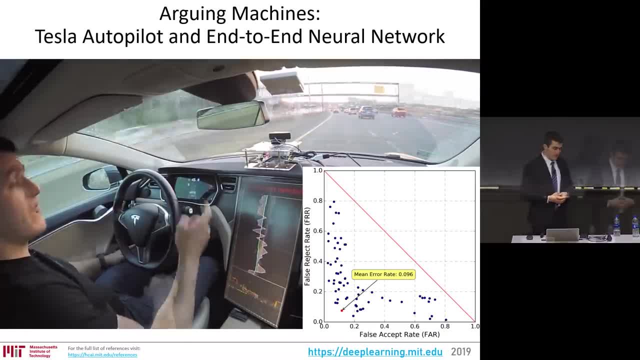 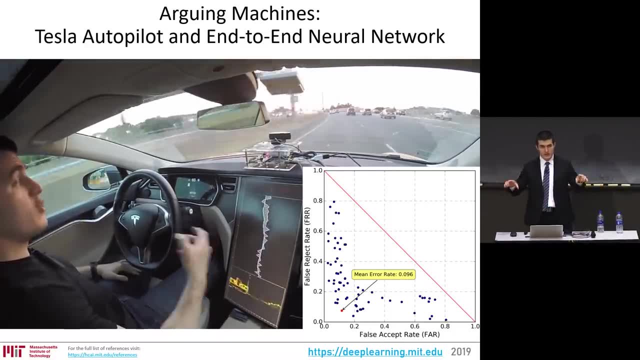 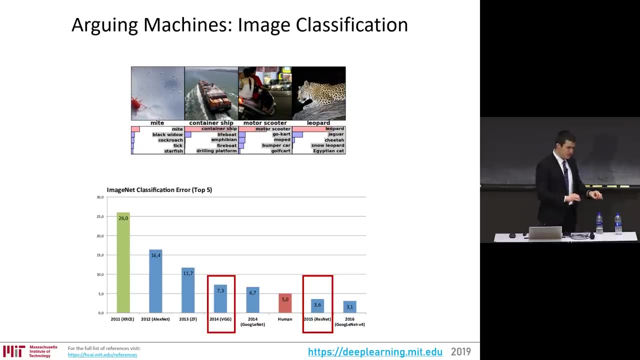 to detect risky, challenging situations. It's an idea about how we supervise AI: by having multiple AI systems that are independent and through their disagreement emerges the uncertainty signal, And we can apply this like the AI folks in natural language would debate. we can apply this. 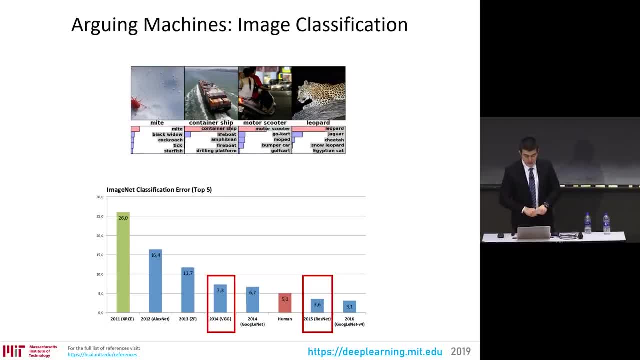 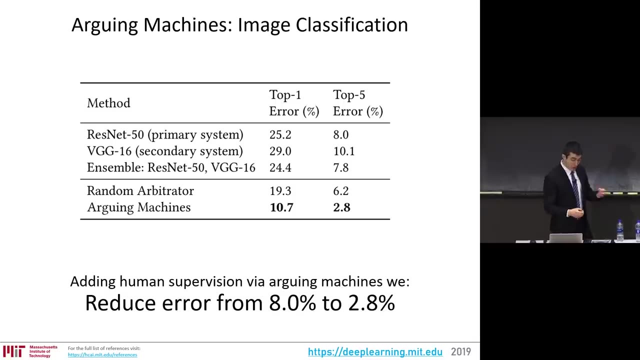 to vision as well, taking two independently trained but on the same training set networks, ResNet and VGGNet, trained on ImageNet, and we can have them argue and in the process improve significantly the accuracy. So when, in the case of ResNet, as an architecture, 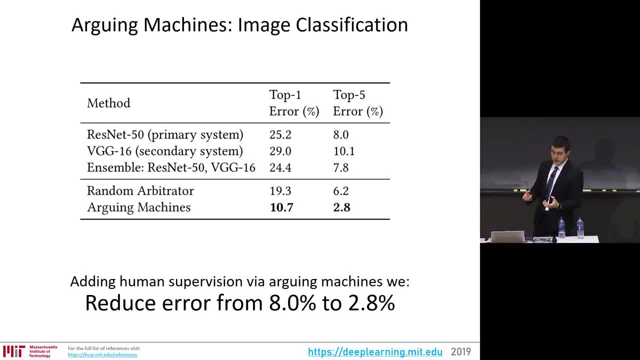 VGGNet. as an architecture trained on the ImageNet training data set, they separately have a certain error. ResNet has an error of 8%. VGG16 has an error of 10%. When we apply the arguing machines framework, when the disagreement is brought to the human. 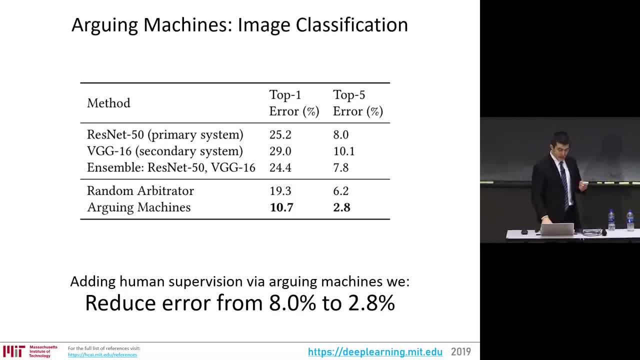 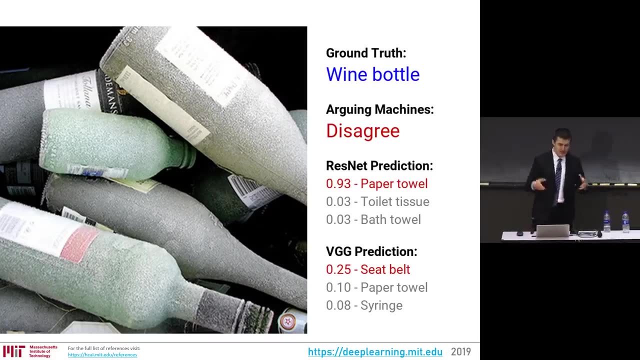 that error rate decreases at 2.8%. Now, if that this is just ImageNet challenge, but if that error meant the loss of human life, this kind of framework is really powerful for overseeing the operation of the AI system. That just examples here where they disagree. 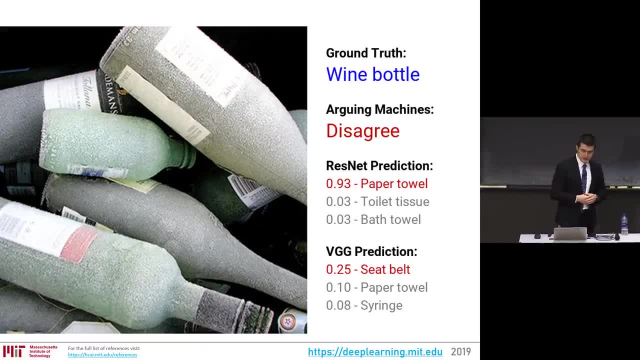 that's a good example. They disagree. so, taking this image that's from ImageNet, the ground truth is a wine bottle and ResNet prediction is that it's definitely 0.93, 93% confidence that it's a paper towel. 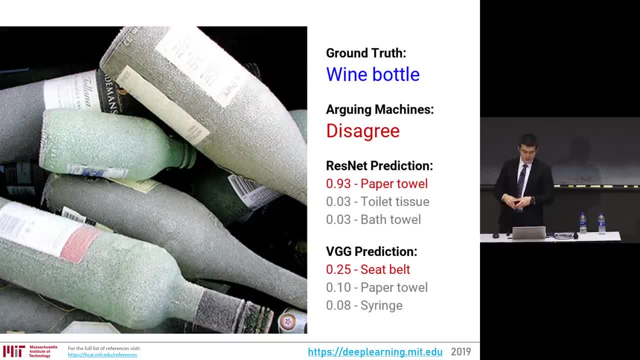 and VGGNet 25% confidence that it's a seatbelt. So these disagreements are then brought in, and then we- the fact that they disagree- arises, the uncertainty, and then human supervision is brought, and then humans are able to annotate correctly. 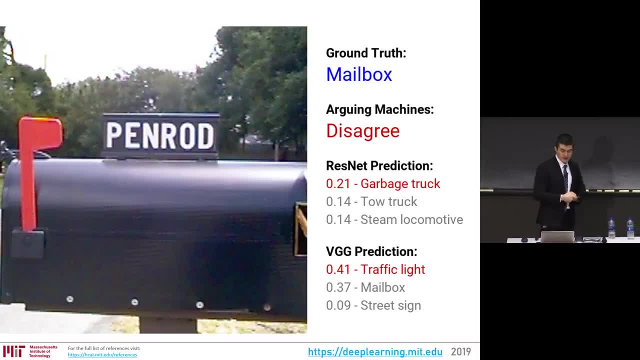 what's going on in this picture? Same thing here: mailbox. the ground truth is a mailbox, The again, the two architectures disagree. One says traffic light, the other one says garbage truck For an autonomous vehicle. you can imagine this being problematic. 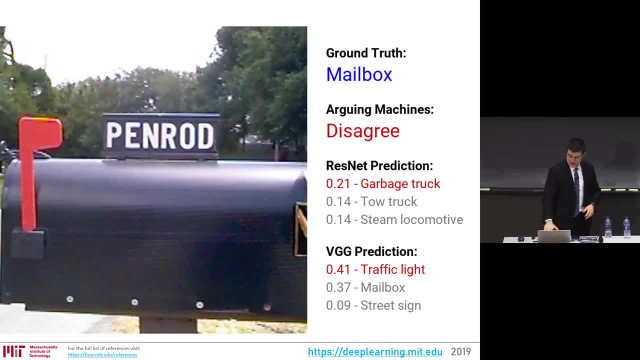 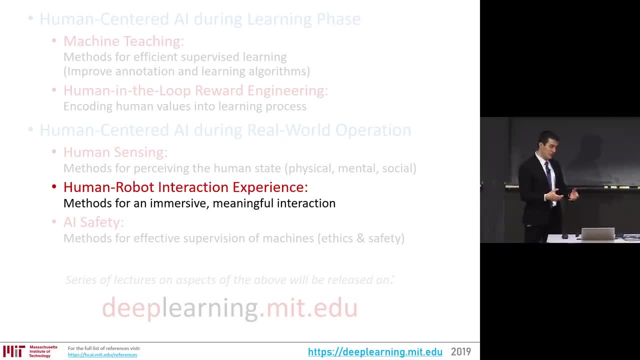 If this is traffic light, it might stop for this mailbox, that kind of thing. That's early research in the field of how do we have AI systems that are more and more powerful? We can also inject human effort to supervise when it's needed. 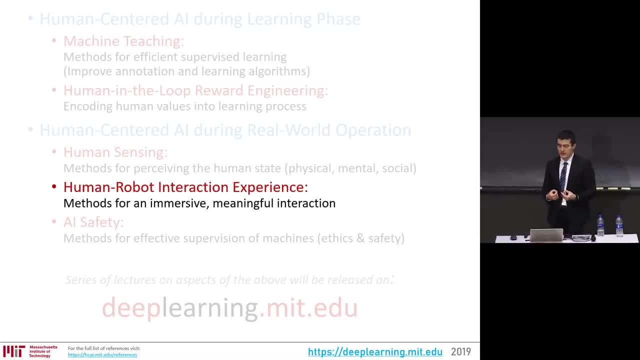 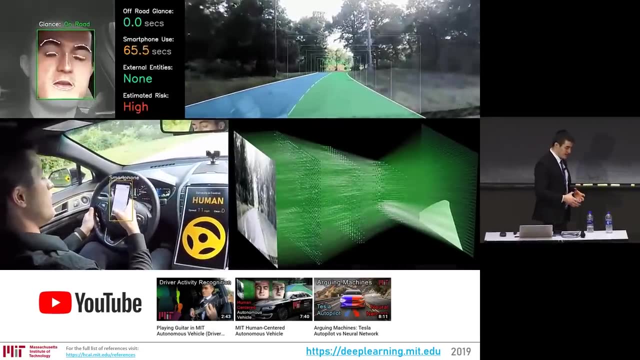 The one that's needed part. the uncertainty signal is the critical thing. so we have to figure out ways to create that uncertainty signal, The sub-area of just creating a rich human interaction. So this is: we're doing a lot of testing. 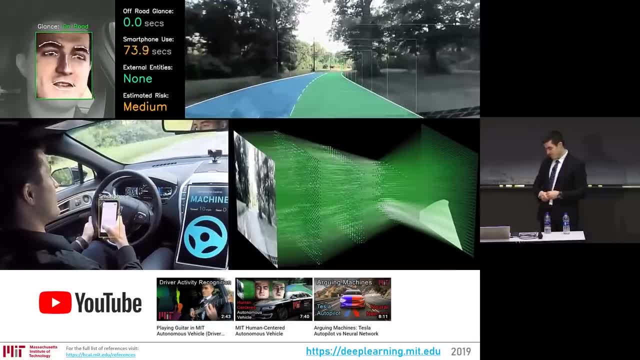 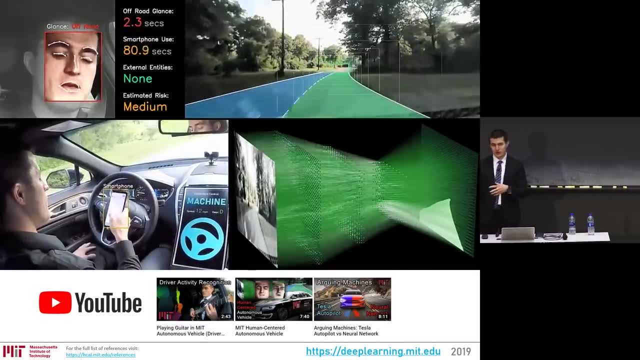 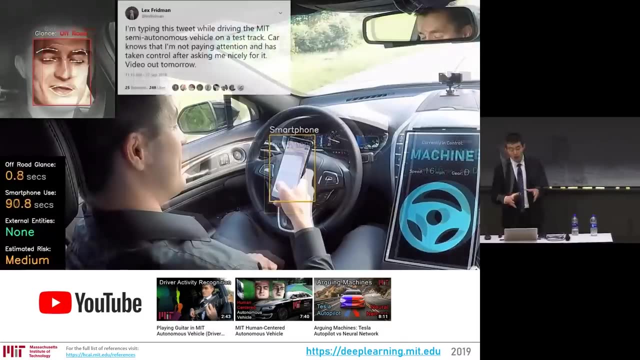 with autonomous vehicles. here I'm tweeting, So we have a human-centered autonomous vehicle here, Here at MIT, that's taking control back and forth from the human based on the activity. That's just me explaining. the video Point is that the driving experience 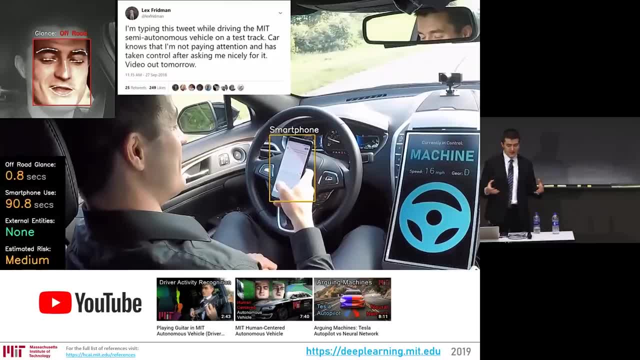 the human-robot interaction experience should be fun and awesome and enriching to life, And that's why you would want to use these kinds of systems. We have a bunch of videos online. You can check them out, including ridiculous one of me playing guitar. 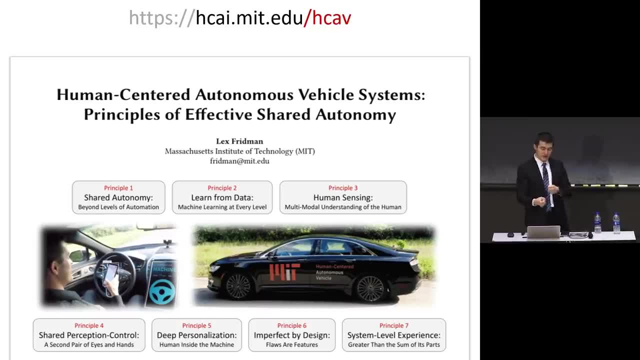 And there's a paper along with this describing different principles of how we have humans and robots work together in this kind of way. There's a lot of totally untouched problems in that space. Most of the robotics community and the machine learning community approaches AI as a system that we want to make perfect. 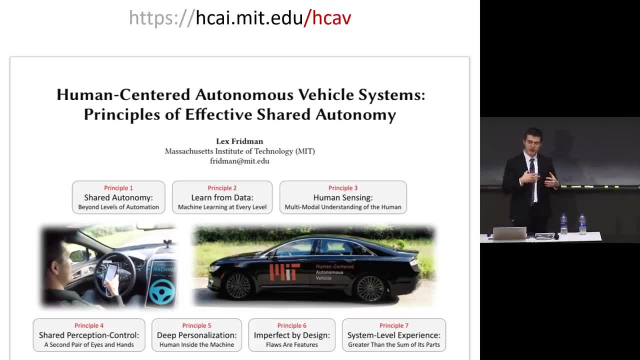 And once it's perfect, we want to then put it in the real world where us humans get to interact with it. Just like what is it? Robin Williams in Good Will Hunting Talking about relationships that nobody's perfect, I think the way I foresee it. 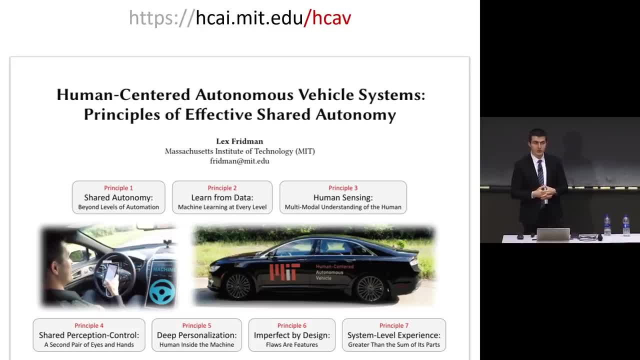 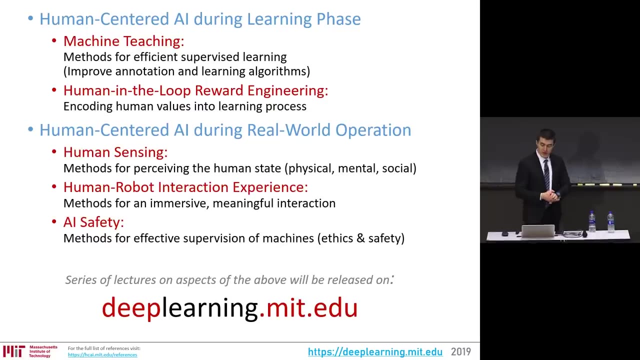 AI systems will not be perfect for the next hundred years, And so we have to have humans and AI systems work together and optimize that problem, solve that problem That both of us are flawed, but together there's something enriching to both. As I mentioned, the videos here will be available online. 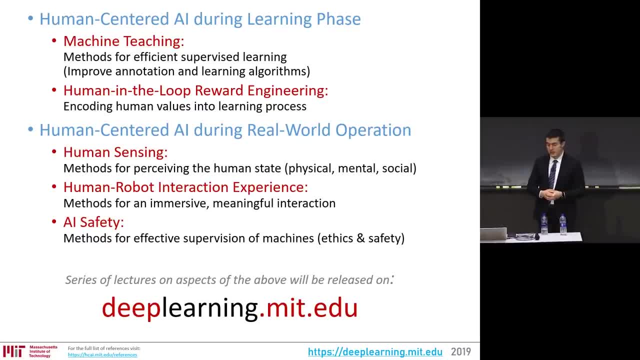 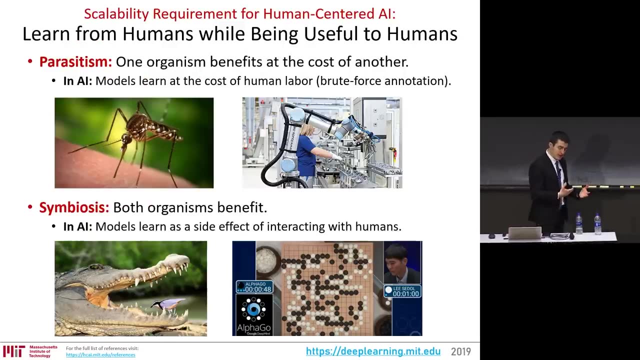 The lectures underlying all the deep learning for understanding the human and underlying the five principles here of human-centered AI, And it's an area of active research here at MIT and globally, And it's one that I'm extremely passionate about And one of the analogies I think about. 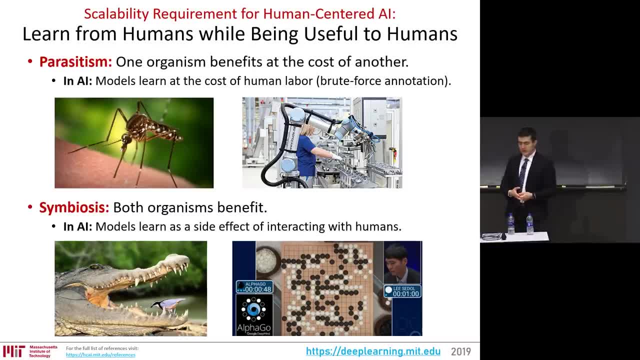 when I think about the success of artificial intelligence systems as an analogy of parasitism and symbiosis, a lot of the ways we're training machine learning algorithms. now we inject a lot of human labor, a lot of really costly human labor, separately, offline, out of the loop. 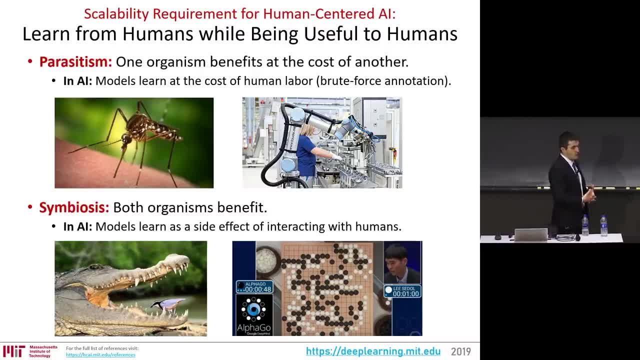 in order to improve the learning models through brute force annotation, And what I see as success in the future requires that the learning is done. the models improve in a symbiotic way as a side effect of interacting with humans. This is done a lot now in reinforcement learning. 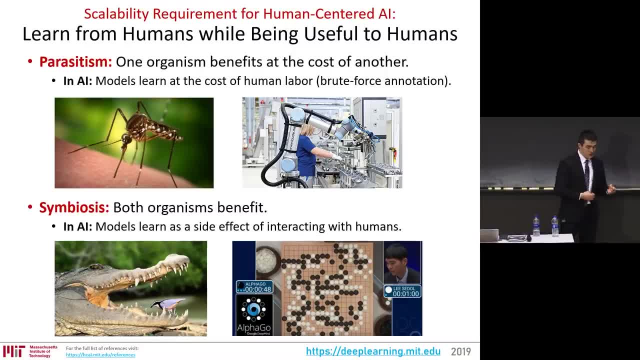 through game playing and so on. But the human computation, the human effort of annotation is something that happens naturally through interaction, not a costly thing you have to pay for, Because when it happens naturally in a symbiotic way, we can increase scale. 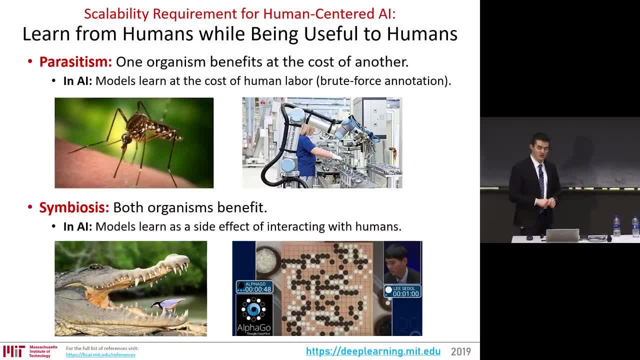 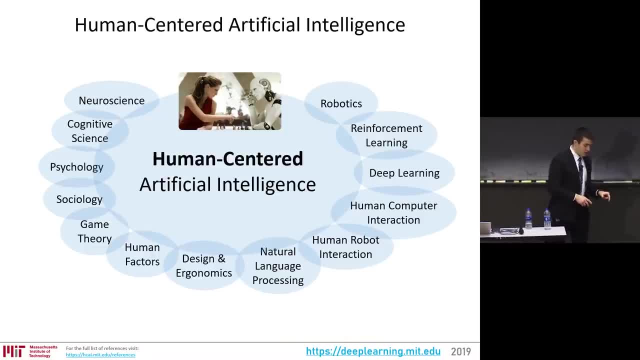 We can scale learning to a degree that's required to solve some of the real-world problems. That also requires solving a lot of aspects of human-robot interaction: from understanding our own brain, from the biological to the electrical and neuroscience to the behavioral aspects captured by cognitive science. 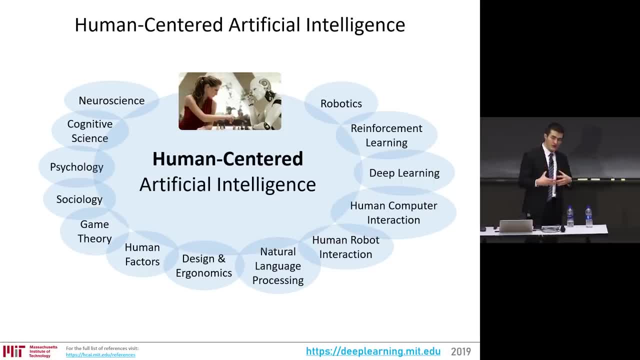 psychology, sociology, to the mathematical formulations of behavior and game theory, to the- when you take that human behavior and put it in the real world with engineering systems, human factors and design. these are all giant subfields with conferences and papers that all of them need to work together. 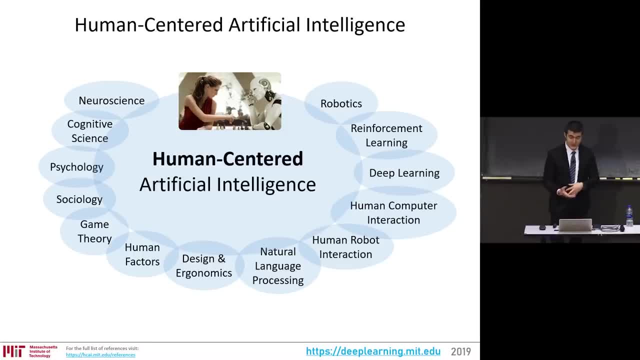 And then on the computer science side, with natural language processing, understanding, understanding language, the human-robot interaction, human-computer interaction, just the interfaces, the what does, how does and what does the computer, the robot, show to you. 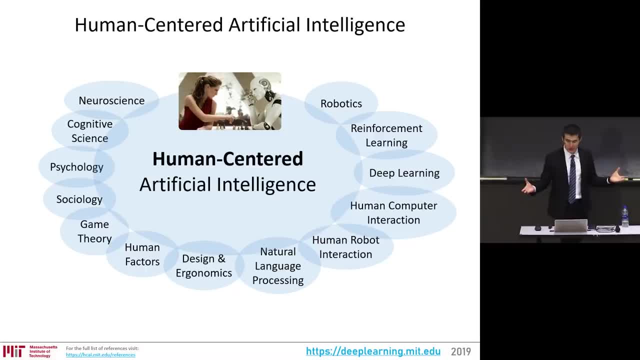 again, entire conferences, And then the exciting aspects of learning from data and deep learning and learning to act from data and reinforcement learning, deep reinforcement learning. And then the robotics is actually building these things, the building the hardware, the- again an entire.